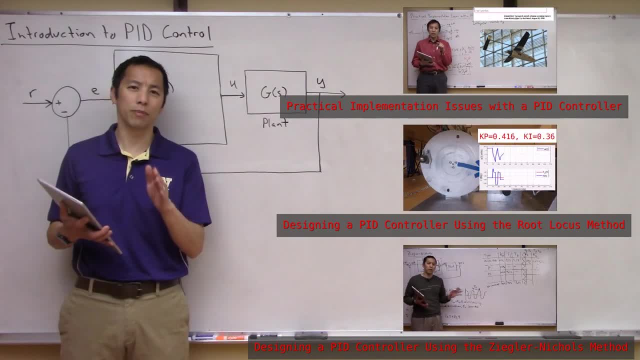 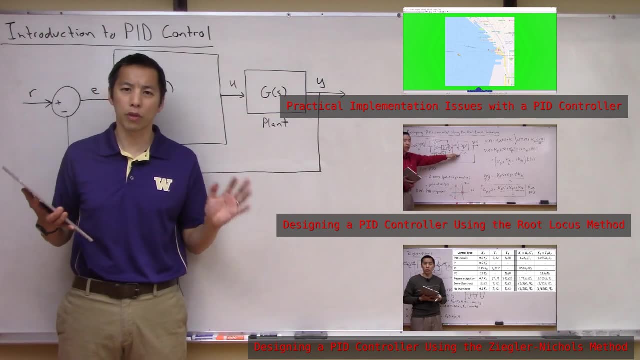 detail. So this extended discussion is very well warranted, because PID controllers are probably the most popular control scheme in history. So if you spend any amount of time working with controllers or looking at control systems, you're almost guaranteed to run across at least one or 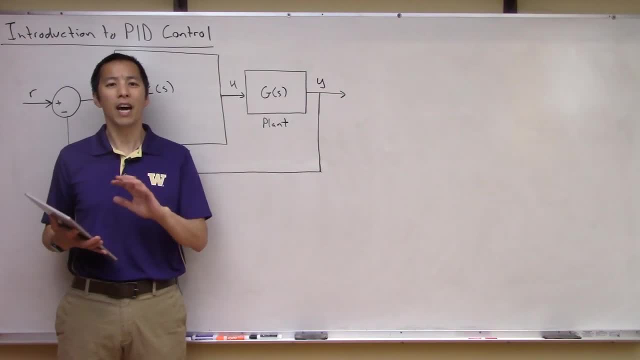 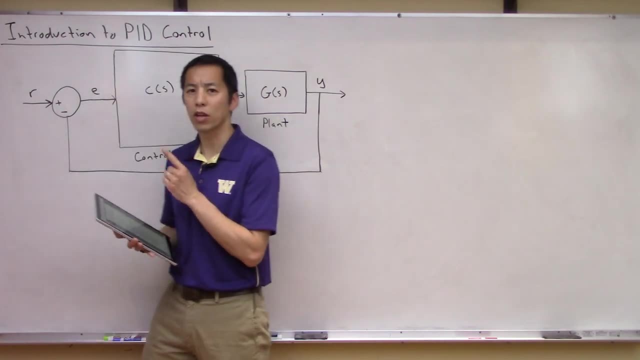 two PID controllers throughout the course of your career. So for today, I just want to get everyone comfortable with some of the core concepts surrounding PID control. So if that sounds like fun, let's take a look at the board over here. All right, so to set the stage for PID control. 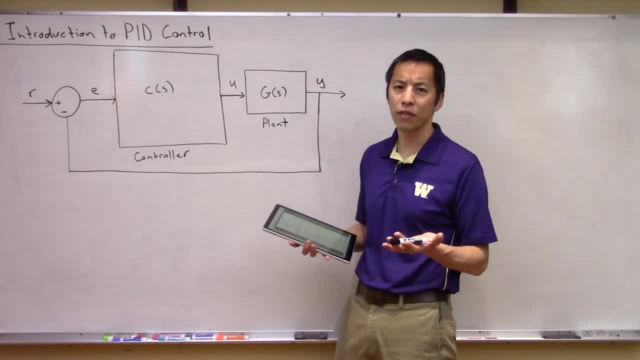 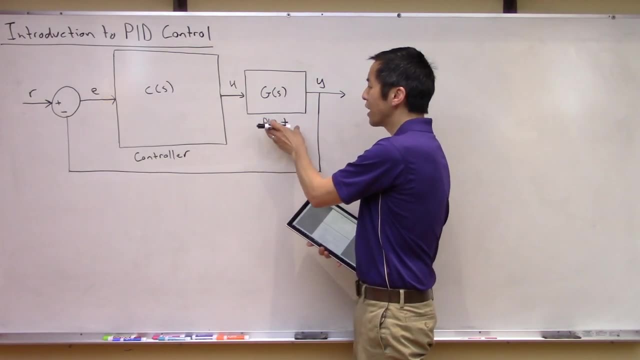 let's go back to our standard feedback control architecture that we've discussed in previous videos. So in this scheme, just to refresh your memory, we've got some kind of plant here, G, And the idea is: The idea is that this plant produces some kind of output, and we would like this output to match. 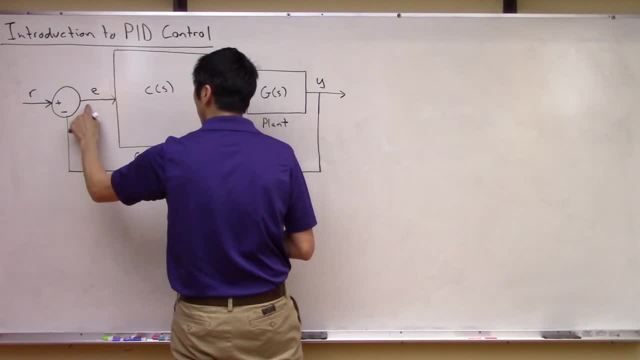 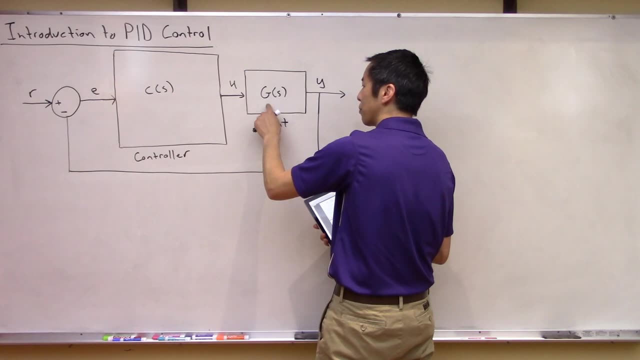 some reference signal. If they don't match, we're going to take their difference to create some kind of error signal And the controller is then going to look at this error signal and compute a control signal which is applied to the plant so that, hopefully, in closed loop, this output signal. 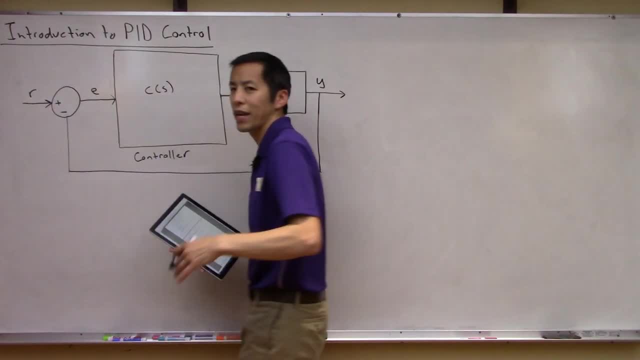 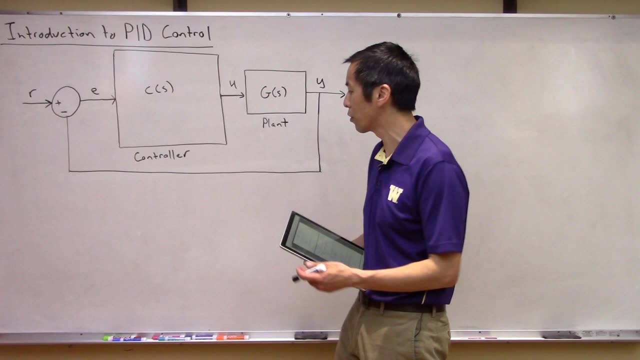 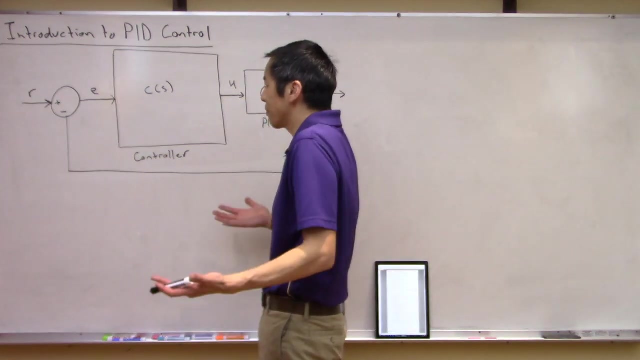 Y will eventually match the input reference signal R. So again, that's the grand scheme, That's the very general idea of a simple, sometimes referred to as an inner loop or a single loop controller. So the whole game at this point is: what does this controller look like? Let's think. 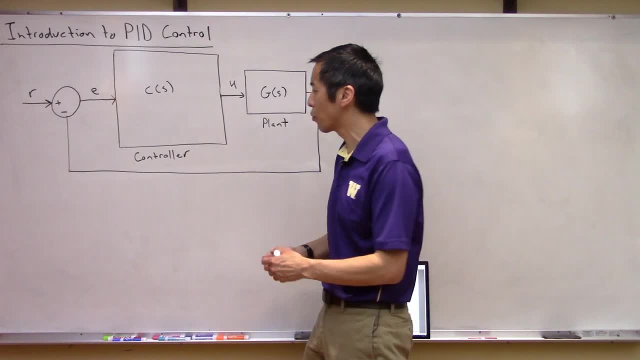 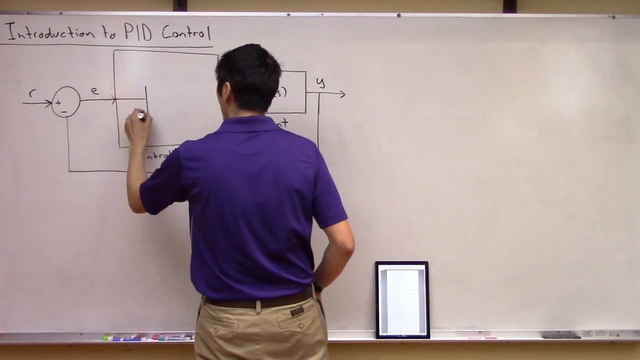 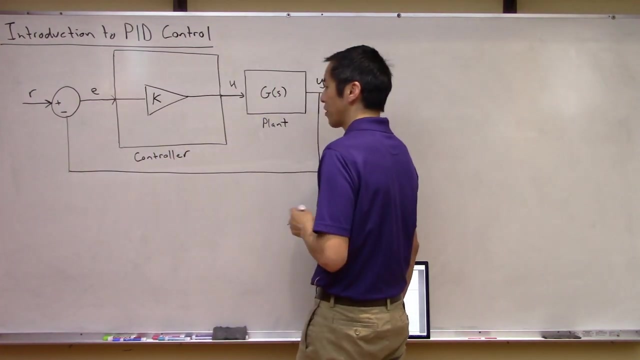 about this. What is probably the simplest thing that you can do here? Well, the simplest thing you can do is you can probably just take this E and run it into a gain of some value. Let's call this gain K, So something like this. This is about the dumbest thing you could possibly do. This is: 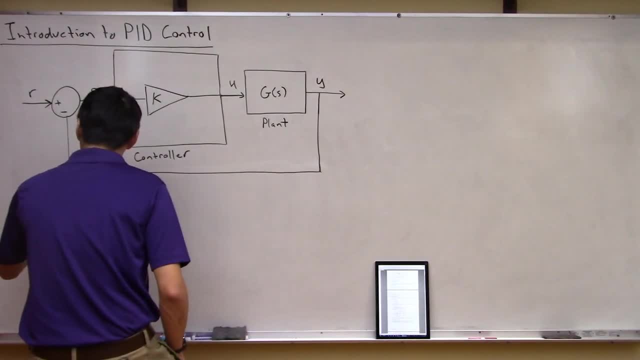 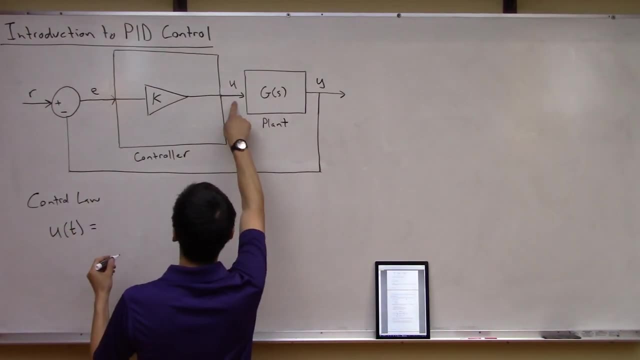 about the dumbest thing you could possibly do And in this case, let's think about what is the control law, right? So the control law basically says that the control signal, at any given time, it's just going to be here, which is just nothing more than this. gain K times the error. okay, So you can see that the control signal 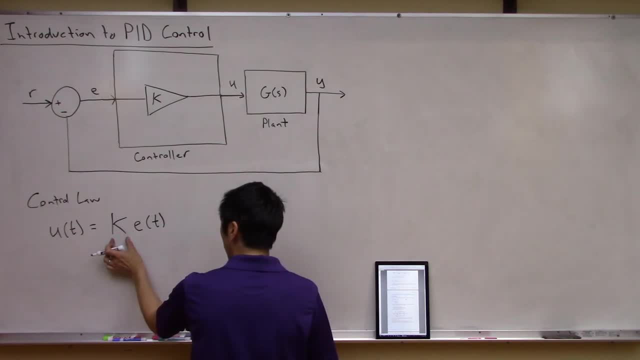 it's just the error multiplied by a number, K. So you can say that the control signal is actually directly proportional to the error right. It's proportional by this gain factor K. So this is actually what's referred to as proportional control right And this P here. 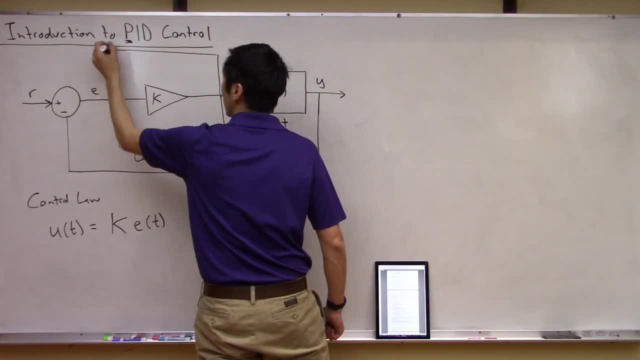 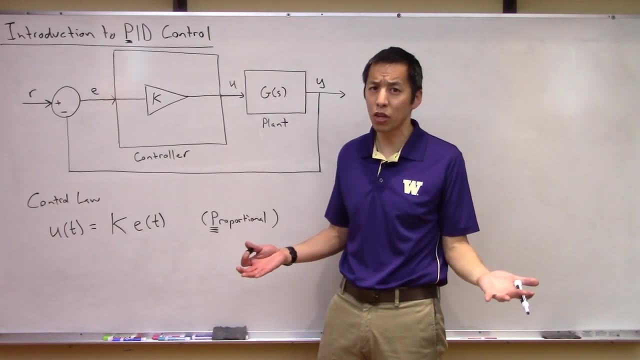 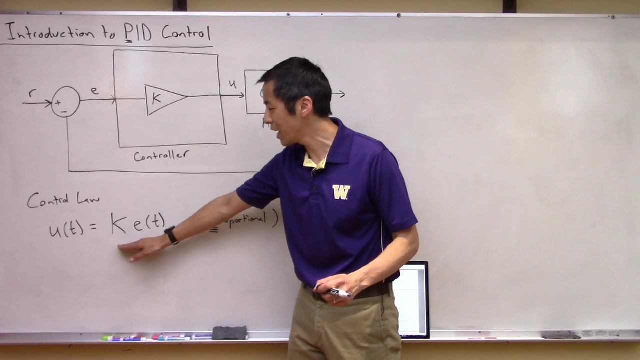 is actually the same P in the PID scheme, So this is pretty much the simplest scheme. It's actually a P, it's a type of PID controller is the simplest controller you could come up with. right, It's nothing more than take the error, multiply it by a static gain, K, to compute your control U. 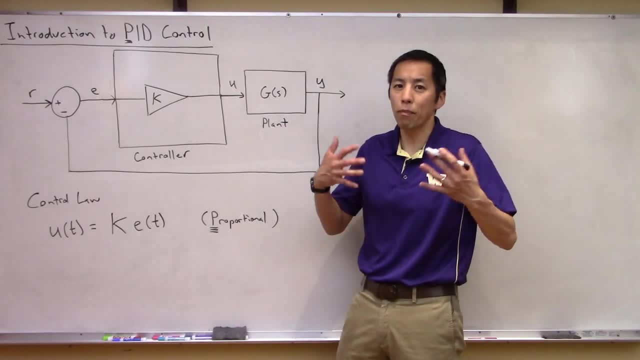 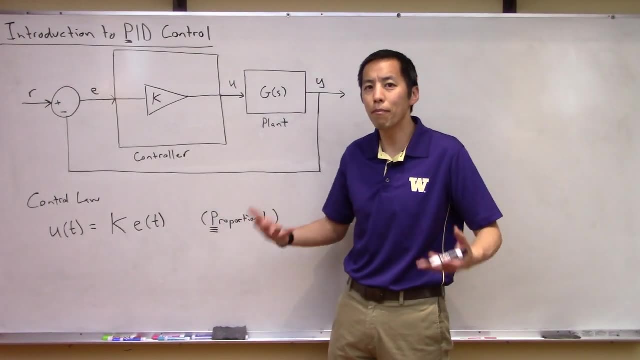 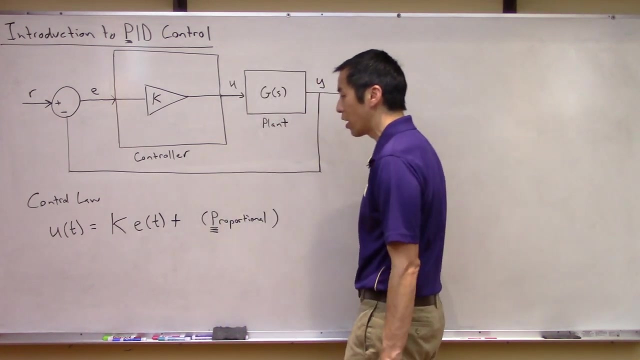 Okay, So that's the simplest thing you can do, And what PID control is and PID controllers is just extending on this. So, instead of just having one term, what if we had multiple terms? Like what else could we potentially do? So the thing we could do is let's start adding on extra terms to our control. 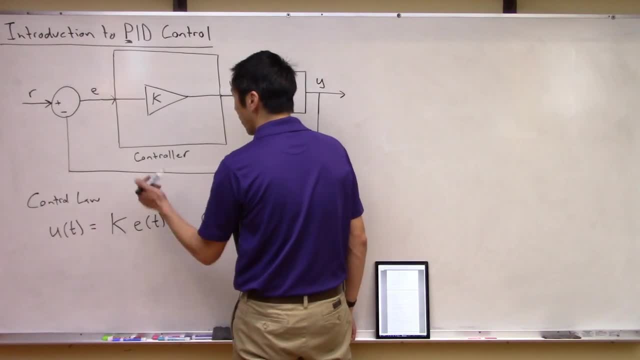 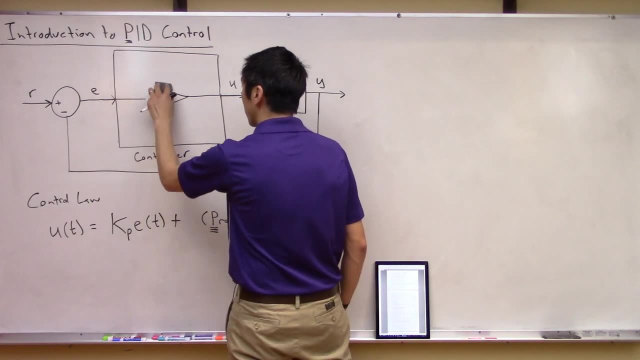 law. So to distinguish this, we're going to have multiple gains. So I'm actually going to call this KP, okay, And actually I'm going to draw this in a slightly different fashion. I'm going to move this up a little bit and you're going to see why we're doing this in a second. I'm going to do it like: 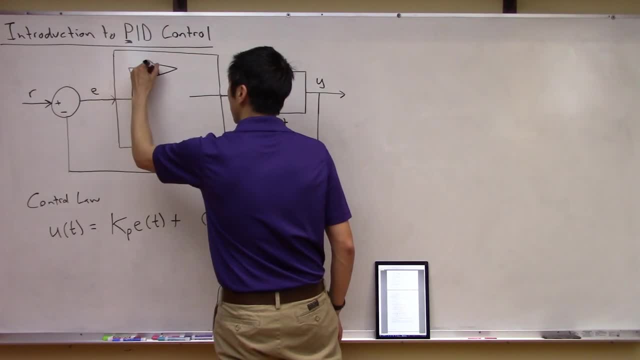 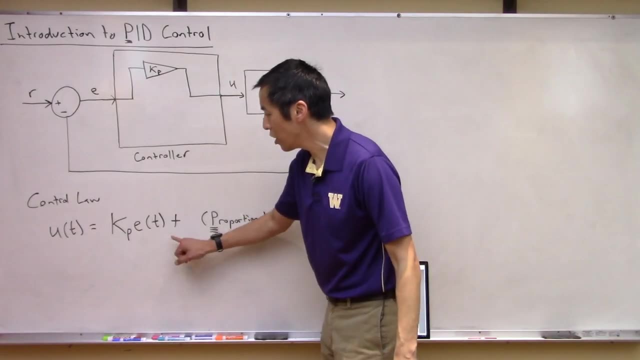 this okay. So you've got this KP. okay, Really, I haven't done anything fancy yet, right? But now what we're going to do is: let's add on another term here. So the next term in my control law it's. 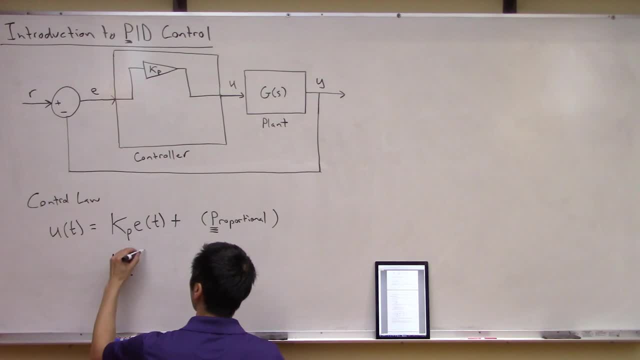 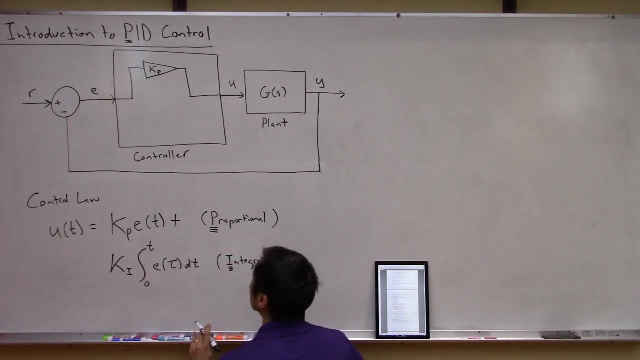 actually going to be a gain: KI multiplied by the integral of the error D, tau from time zero to time T. okay, So this term, right here is sometimes referred to as an integral component. right And again, this I here is this I in the PID. 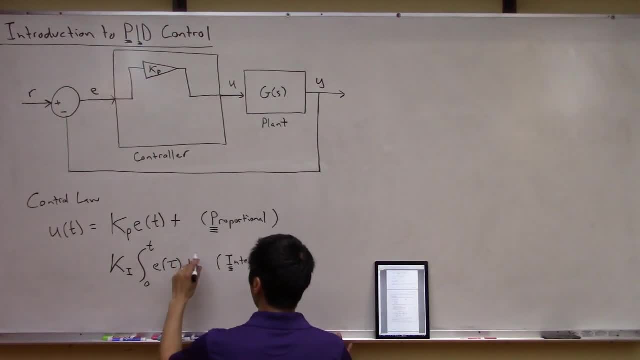 scheme right. And then what we're going to do is let's add on a third term, which is going to be KD times, the time rate of change of the error right, And this is sometimes referred to as a derivative right. And again, the D here is this: 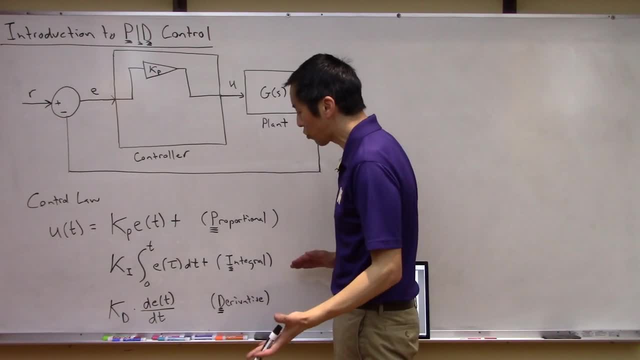 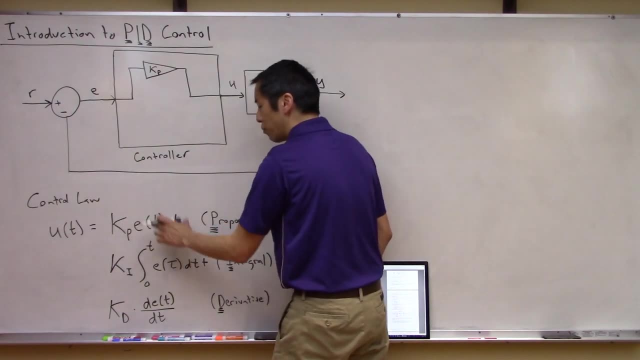 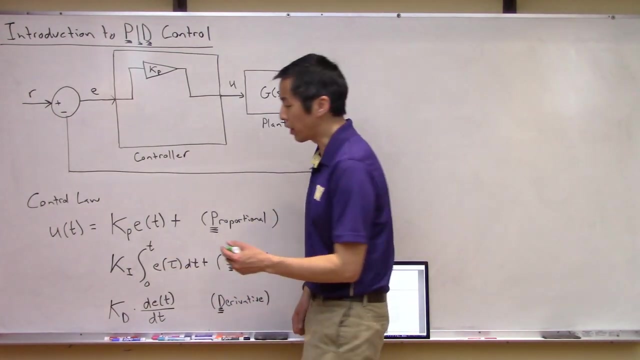 This D in PID control. So we can see that PID control stands for proportional integral derivative, because it basically has the control law being computed using three terms. So this term right here is the proportional part. Let's go ahead and maybe I'm going to put this here in blue. 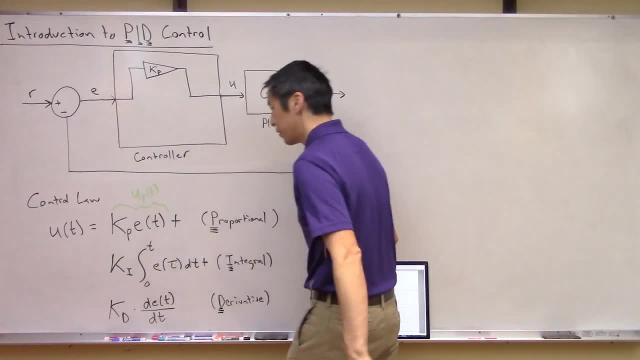 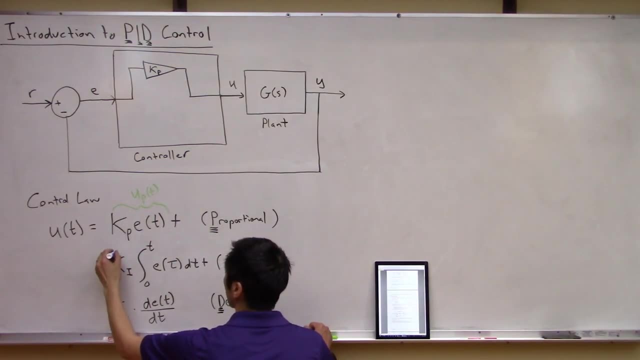 Let's call this U proportional, okay, Or sorry, I'm going to do this in green. and then let's go ahead and put this I term here. this entire I term here is going to be UI, okay, And then, finally, this term down here is UD, okay. 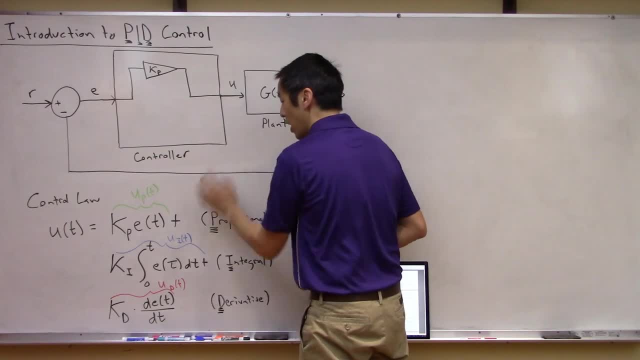 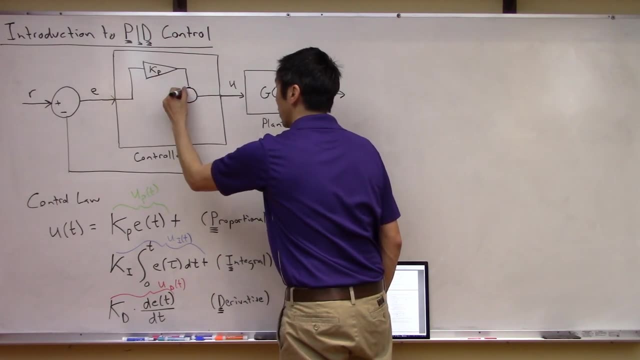 So we see that the control signal here is made up of three components. So maybe let's actually draw this in a block diagram format, because I like to always see things in block diagram format. I mean, this is an explicit control law, right. 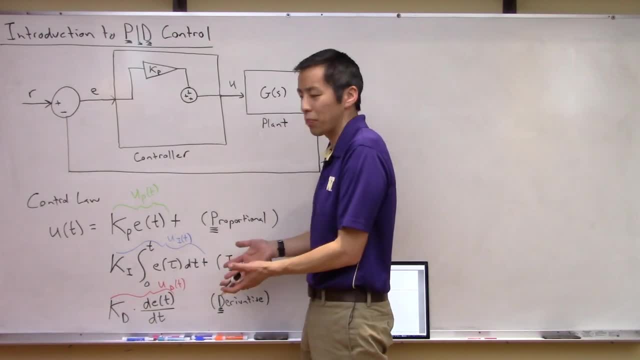 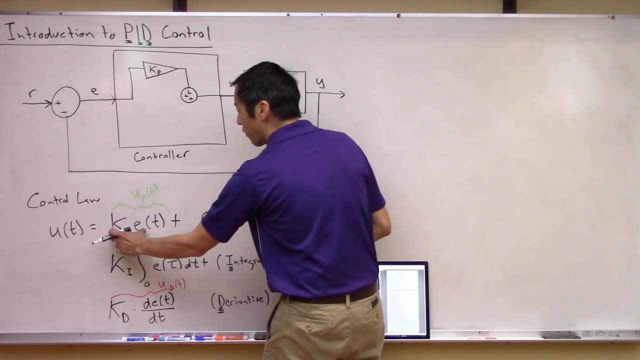 You could go ahead and implement this in a- you know, C++ or something like that, but I like to think in terms of block diagram. So let's translate this control law into a block diagram. So we already have this term right here, right? 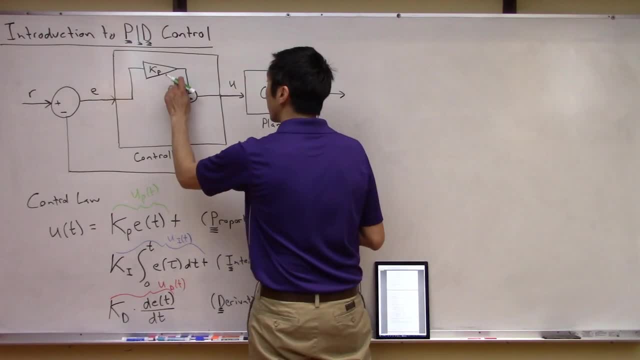 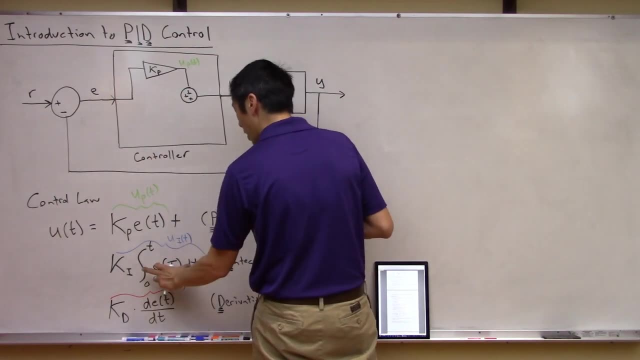 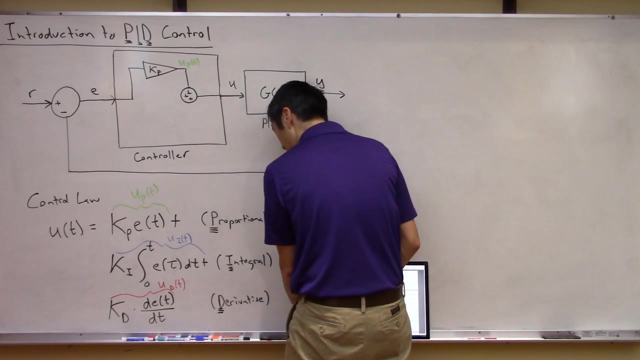 You can see clearly that right here. this signal here is UP right. It's the green part. right. It's nothing more than KP times the error. Now we got to get this blue part right. It's KI times the integral of the error. So what we need to do 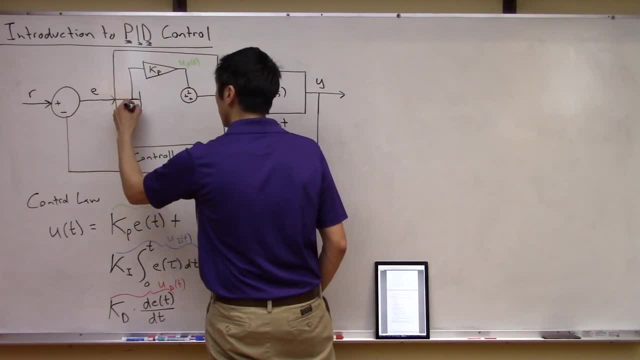 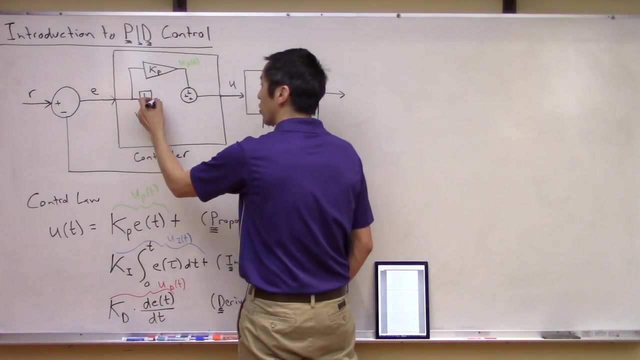 here is: we need to integrate, and I'm going to write 1 over S for the Laplace version of an integral. So this is an integrator right. So what this thing does is you give it E, it just accumulates or integrates all the error that's coming in. 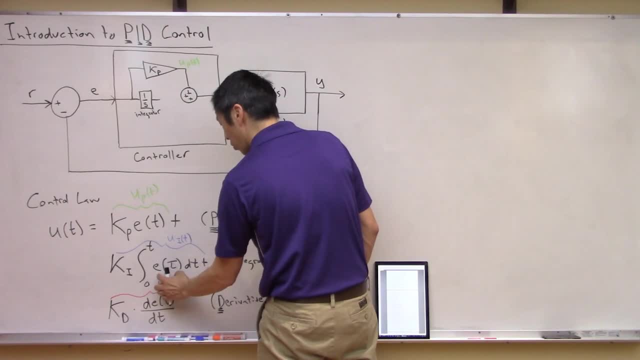 So coming out of this is basically this term here: integral of E, tau, D, tau from 0 to time, T. right, That's what that integrator block does. It just does the integration of the error signal. Now, all I got to do is multiply this by the. 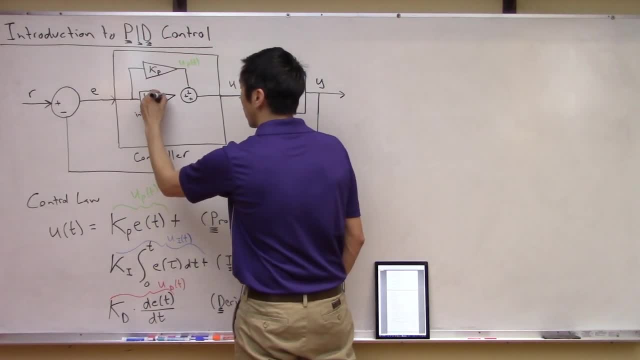 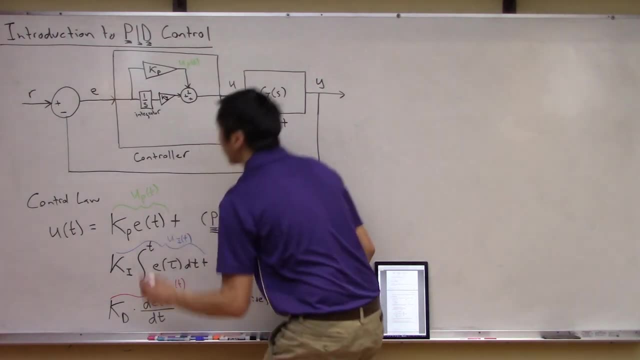 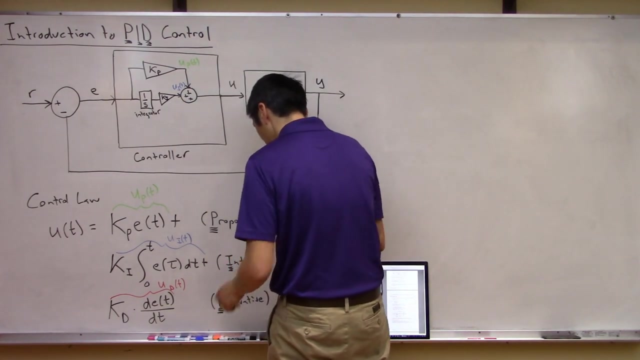 overall記得 to multiply by again KI right. So now here's your KI right, And then that goes into this summing block, And right here we have the signal Ui of time T right? That's this signal right here. And then, lastly, what we've got to do is: 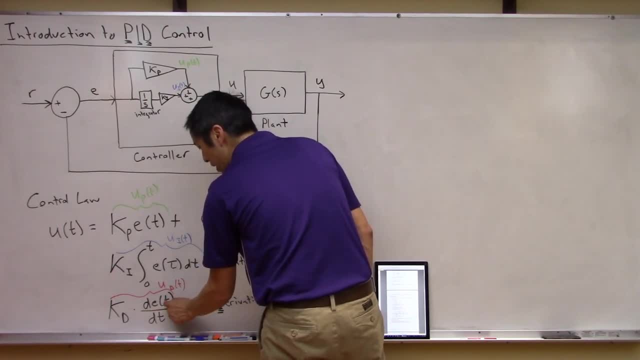 take into account this term right. So what this term says is you need to compute the instantaneous time rate of change or the error dot right of the error at time t. so again, let's go ahead and branch this off and i'm going to go write it. 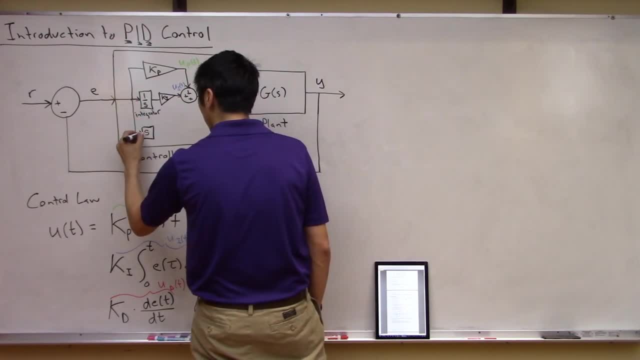 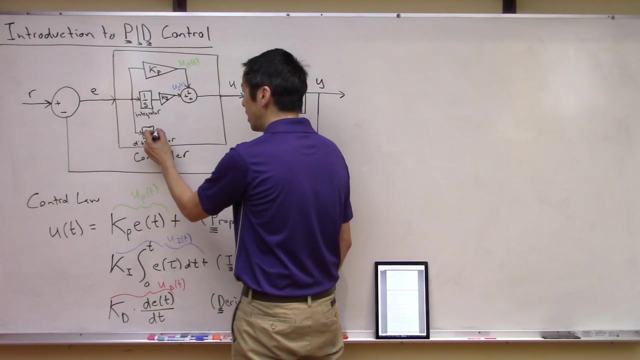 like this again. let's just use the laplace version of an integrator. so this is a uh, an s and you can think about this block as just a differentiator right whose sole job in life is you give it a signal. it computes its time rate of change of that signal. so coming out here is e dot this term. 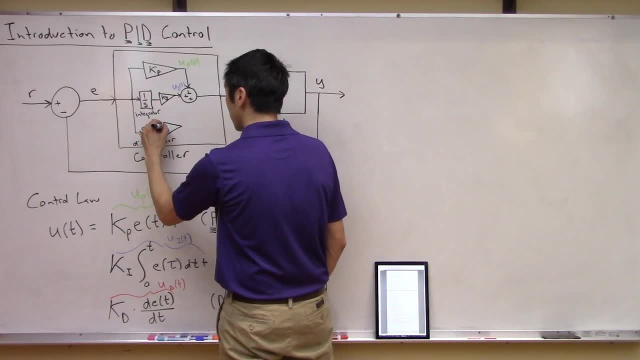 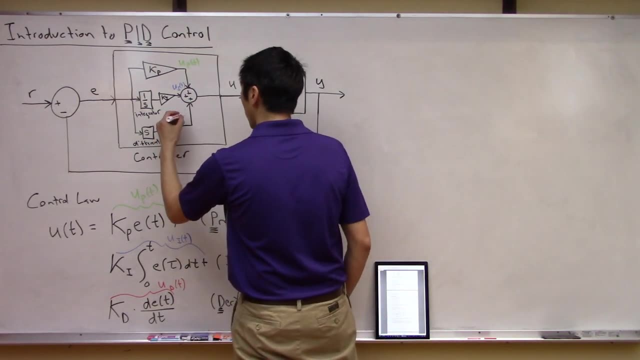 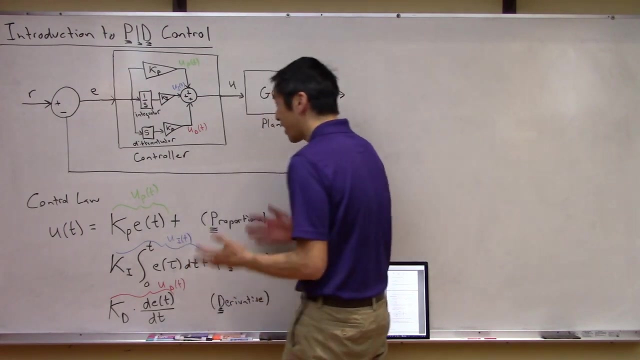 so i just need to now multiply it by kd, kd, right, and that goes into the summing block, and now this signal here is our ud. okay, so this is. what's great about a pid controller is that it is actually surprisingly simple. that's all there is to it. it's just a controller where you have the 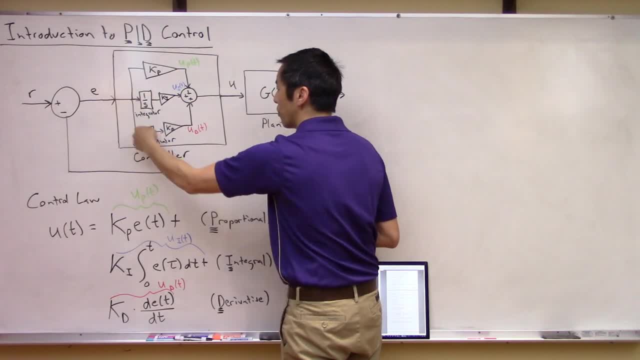 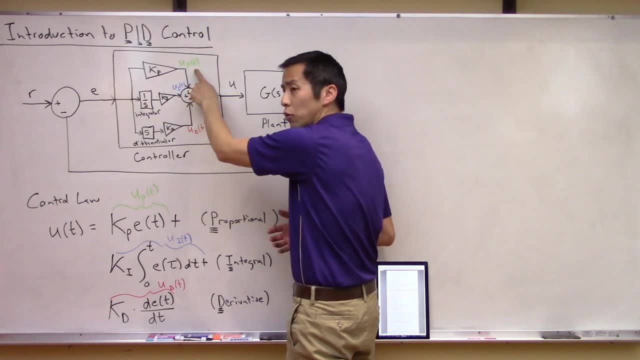 error coming in and the error then gets sort of split into these three branches or these three terms. and That's all you do, right? You just take the error, multiply it by kp. that gives you the proportional component of control. There's also an integral component of control. 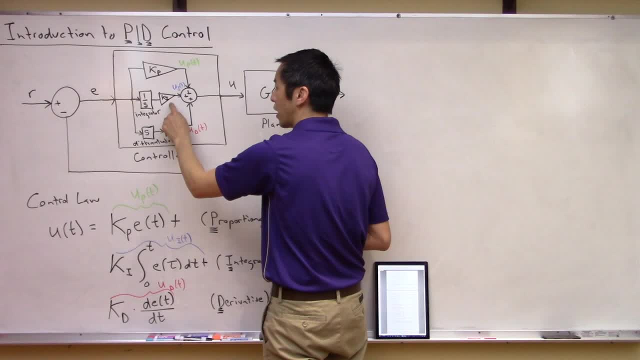 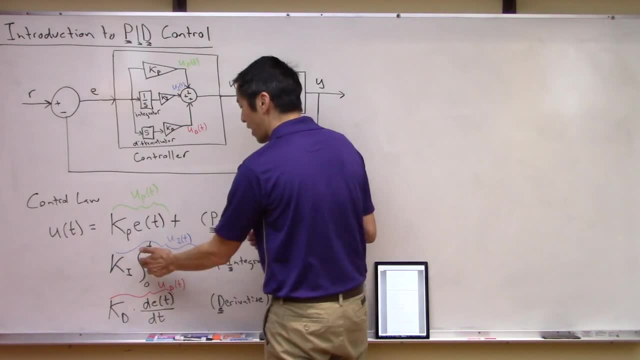 which you get by basically integrating the error and then multiplying by ki. Or you can flip these around right From our block diagram algebra discussion. for the fact that this is a linear system you can. actually, it doesn't matter if the ki comes before or after the integral right. 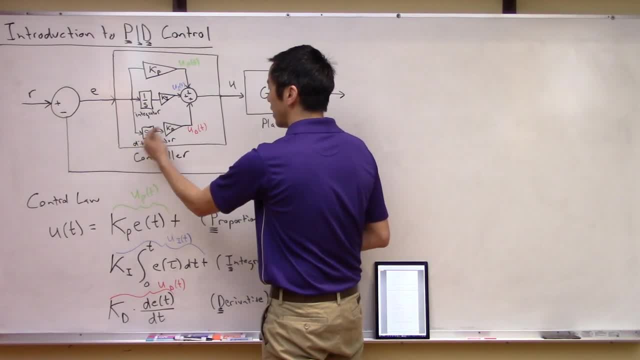 And then same thing for the derivative right. You can basically switch this around. It can be kd times s or s times kd, it doesn't matter. But at the end of the day you have this third branch here, which is basically has something to do with the derivative of the error right. 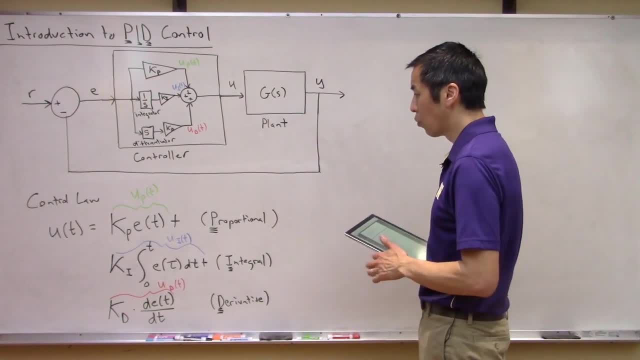 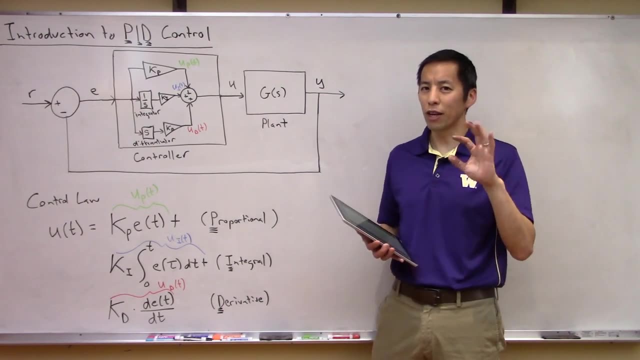 So, in a nutshell, that's pretty much what this does, right? So computing, it is really really simple. okay, Now I'm going to put in your mind right now- just stick in the back of your head- that, yes, this seems simple. 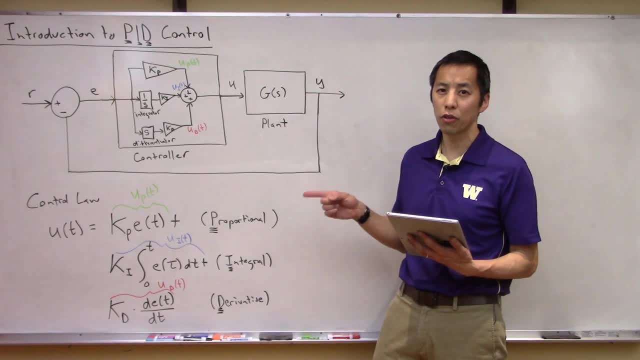 but there are a lot of ways this can go pear-shaped And we're going to talk about that in other dedicated videos. But for the time being, let's assume everything is hunky-dory, and we're going to talk about it in a little bit. 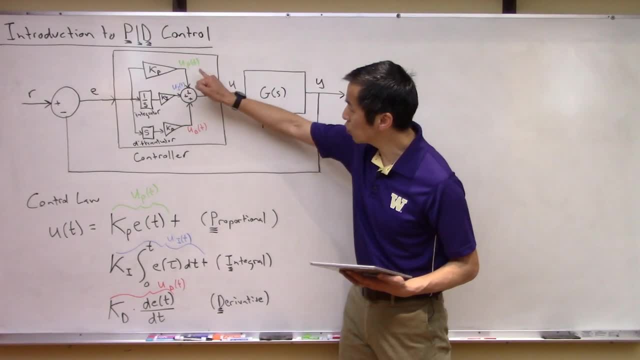 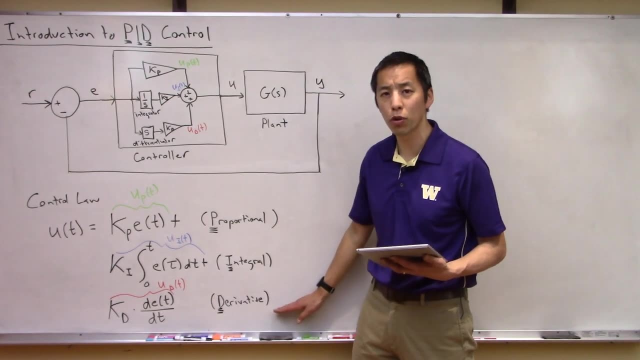 We're going to go ahead and maybe let's examine each one of these terms this up: ui and ud, or the proportional control, the integral control and the derivative control portions in isolation, by themselves, just so we can get a better feel for what they do and how they behave. 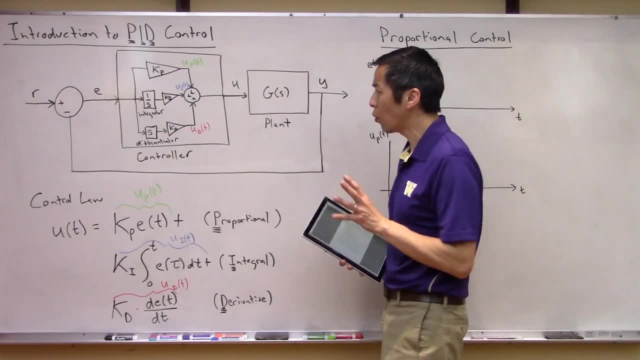 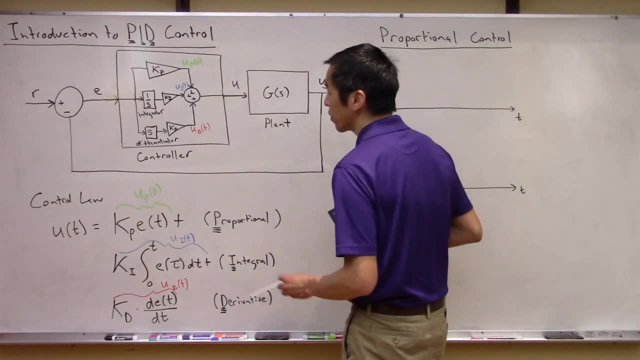 All right. so, to get a better feel for what each of these terms do, why don't we start with just the proportional control, And what we can do is let's consider it by itself? So, in other words, let's see if we can ignore. 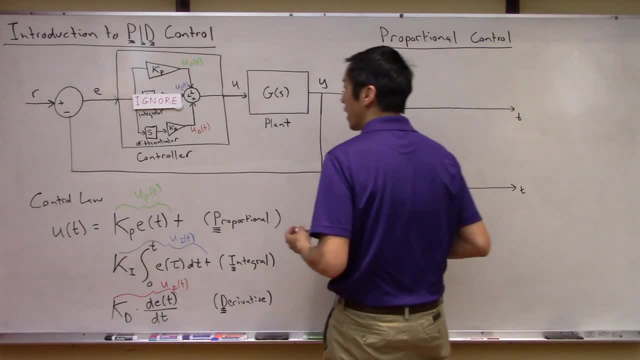 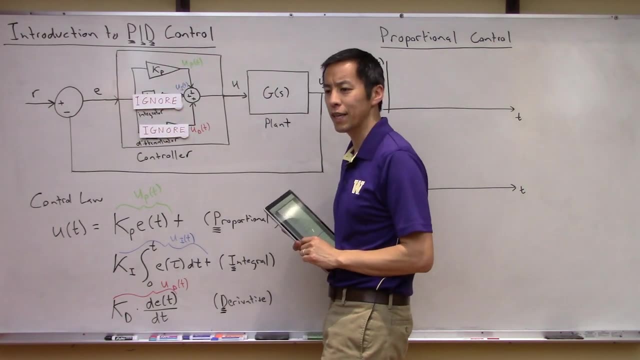 the integral control by itself. So I'm going to have a little sticker here that says: just ignore that And let's also ignore the derivative component. So the only thing we've got is this proportional control right. And again we said earlier at the beginning of this discussion: 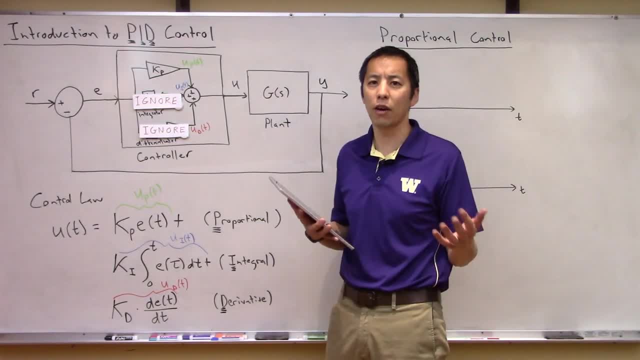 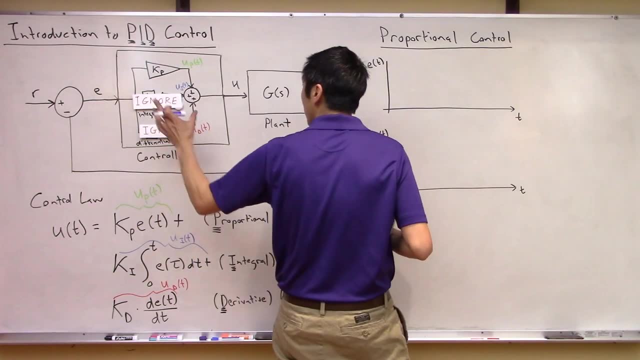 that this is probably the simplest controller you can have, So let's see if we can understand how it behaves and just some general characteristics about it, right, Okay, so what I've done here is: let's just look at, since we're only caring about the controller- 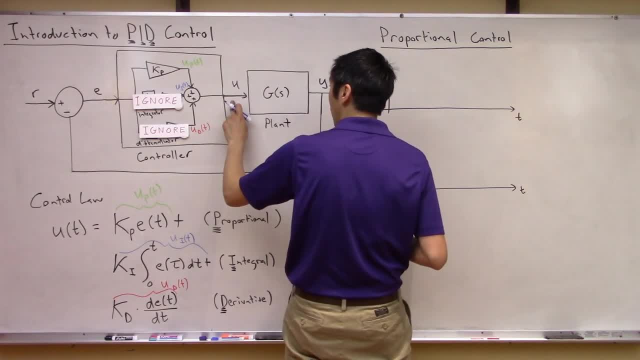 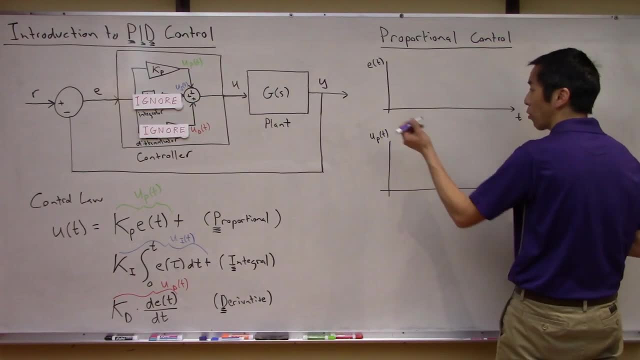 let's look at the error signal going in and what the control signal coming out might be. And again the control signal: it's just UP, right, It's only. that's the only component. So I'm going to draw the error in purple. 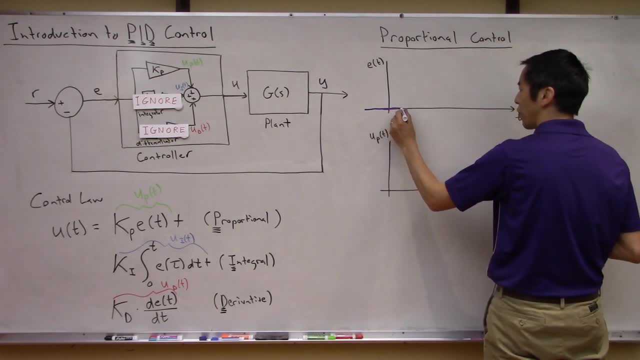 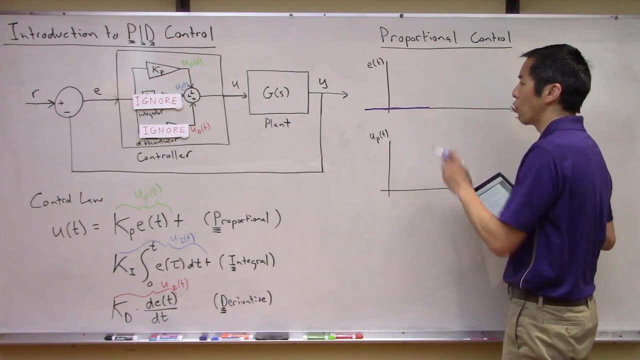 And let's go ahead and say that everything is fine, Everything is fine And we have zero steady state error or, excuse me, zero error, And then at some point we introduce some error. So what that could mean is that suddenly 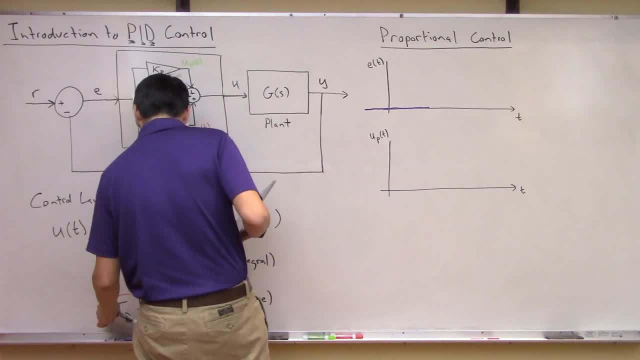 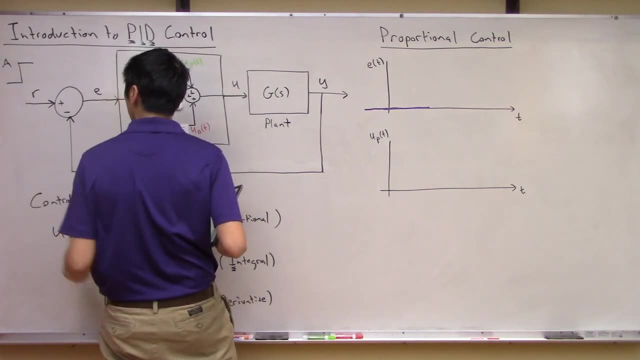 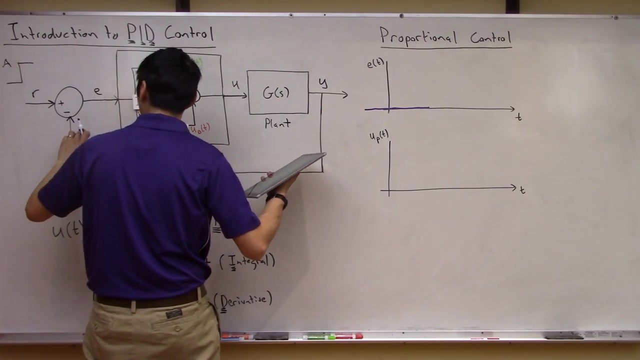 you know, everything is fine. The output is actually matching the reference And then at some point we maybe have a step input of magnitude A At some time and that will create a jump in the reference signal. The plant can't respond instantaneously, right? 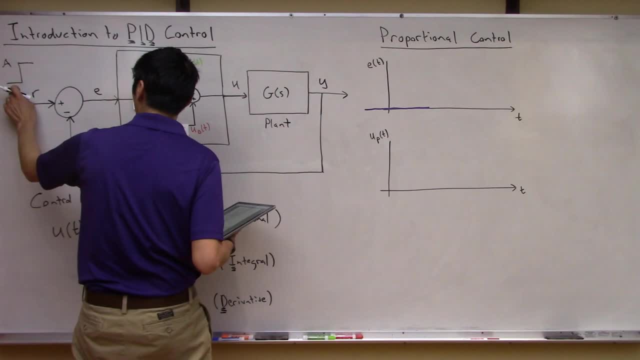 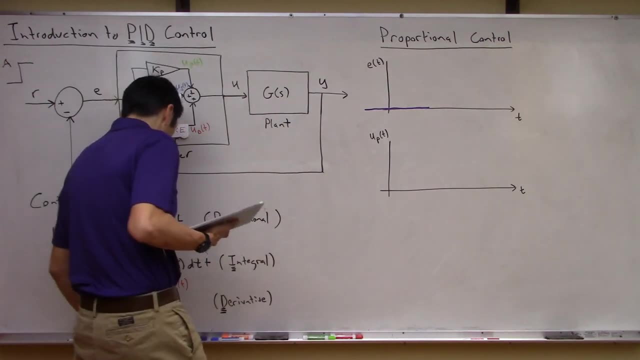 So this signal Y is still going to be at the old value. So when you introduce this step, there's going to be a step in the error right Of also of magnitude A. So what the error signal is going to do is it's going to jump up to A. okay. 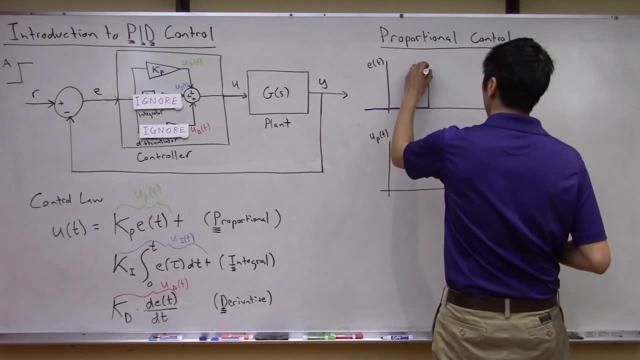 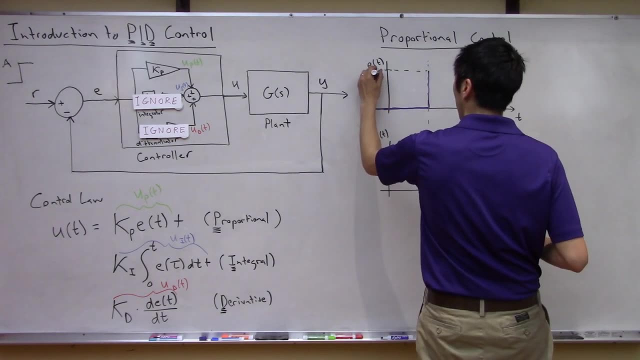 And I'm going to just label all of these about and I'm going to put a little dashed align so we can see this kind of event horizon. Okay, and this is now going to jump up to a value of A. okay, So let's now go ahead and draw in green. 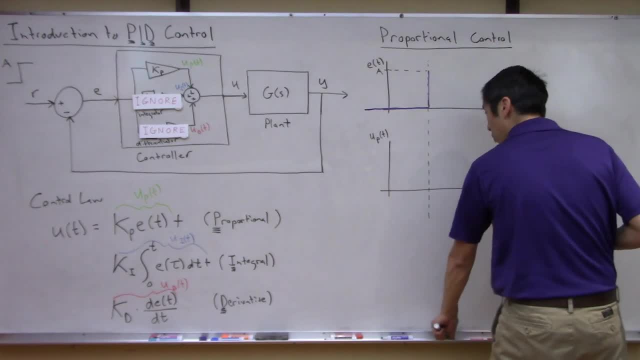 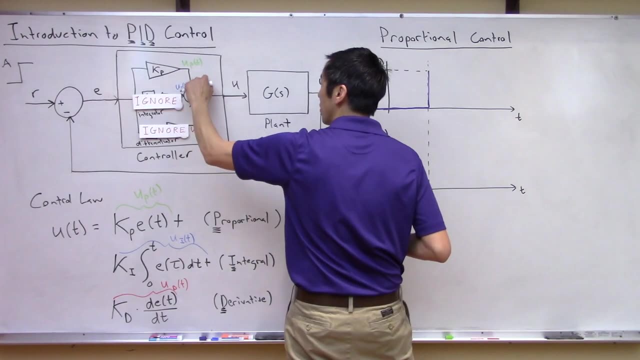 What is the proportional control signal going to do? So again, we can see very easily what it's going to do in this window. right, Because there's zero error. right, There's going to be zero control. right, Because that's how this works. 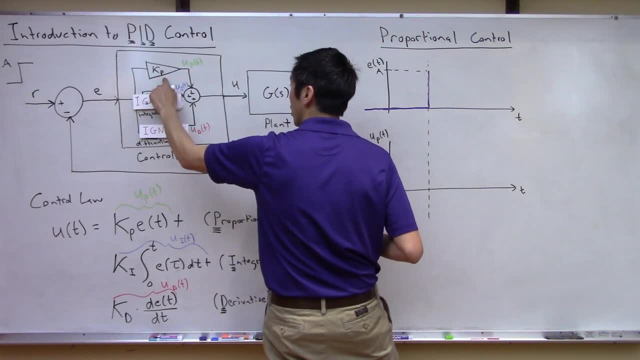 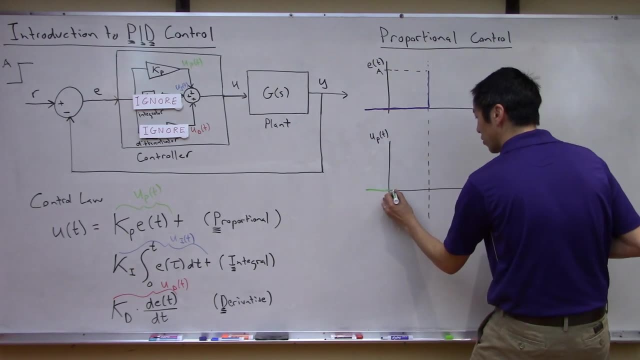 The control is just the error multiplied by KP. So I don't care what number KP you have. If E is zero, this is going to be zero. So the control signal is just zero, zero, zero, zero, zero, zero. 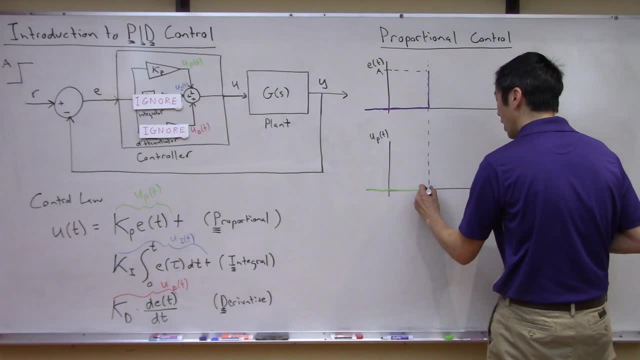 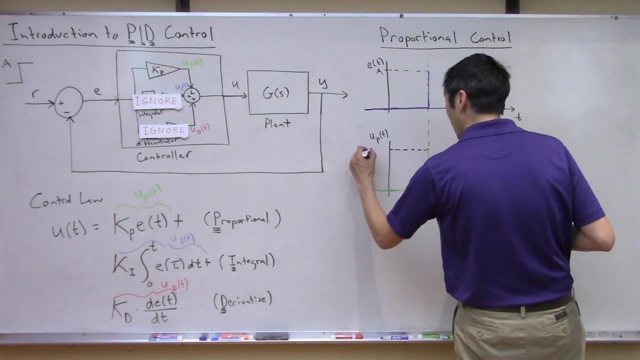 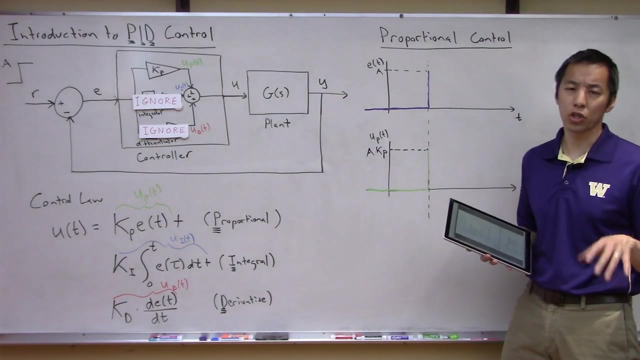 until this event horizon again, And now this is now going to instantaneously jump up to a value now of what This value is going to be: A times KP, right? So this is what's actually kind of nice about a proportional controller is a proportional controller. 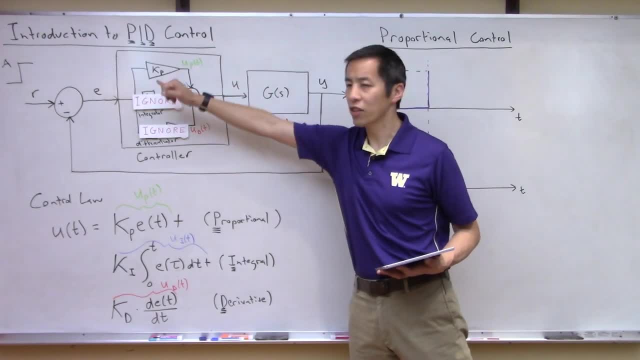 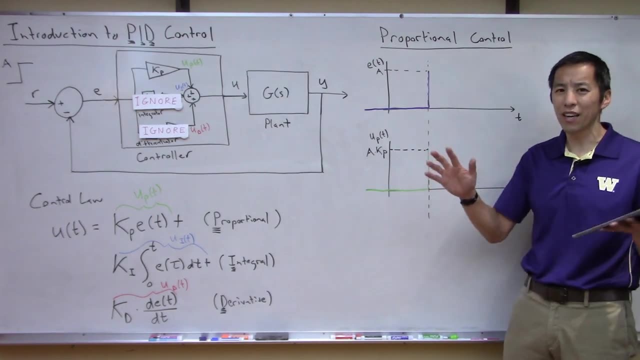 is going to respond instantaneously. right, This gain is just a multiplication that happens right away. There are no dynamics associated. So a proportional controller is going to kind of freak out a little bit. right, It's going to realize there's a large error. 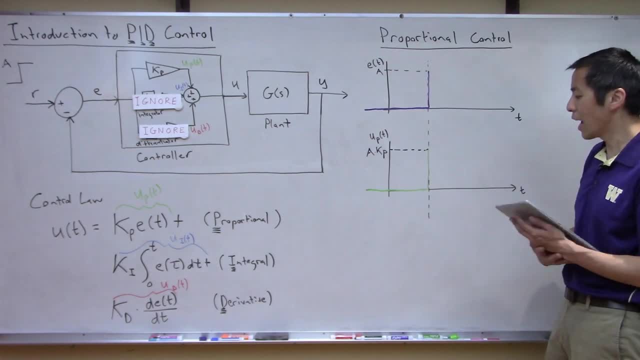 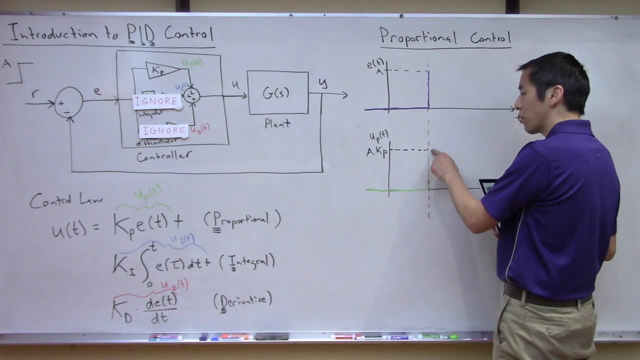 and it's going to then apply a large control signal right And hopefully you've got this control signal set up in the correct orientation, in the sense that this positive number of AKP, it's going to start pushing this signal Y to start matching this signal R. 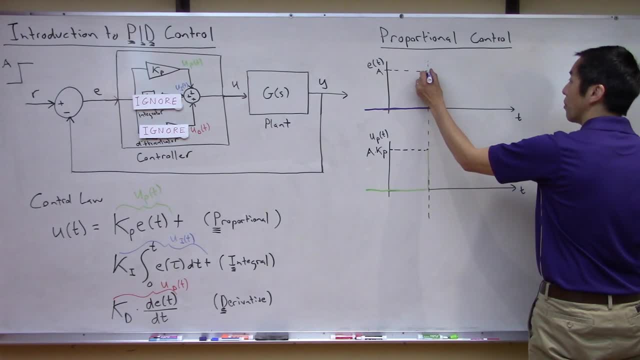 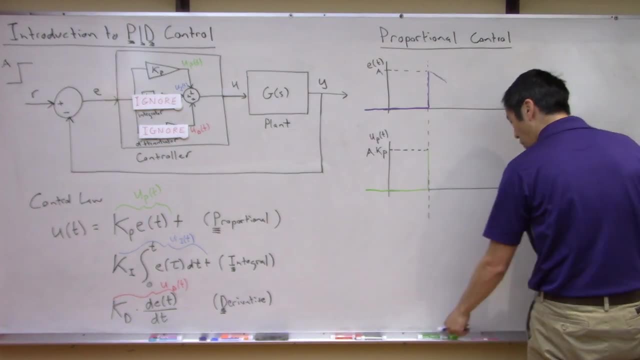 So what the error is probably going to do is it's going to probably start coming down. right, Would you agree? right, As the plant starts to respond, it's going to start coming down. Now, what is the control signal going to do? 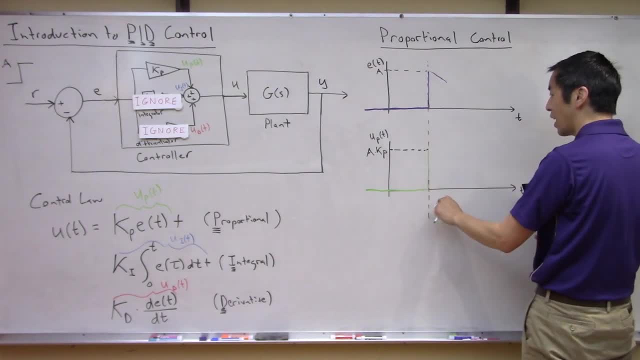 Again, the nice thing about this is to get the green line. we just multiply the purple line by a gain KP, So this is going to basically mirror it like that, right? So this is where it gets interesting, though, If you've got this long enough. 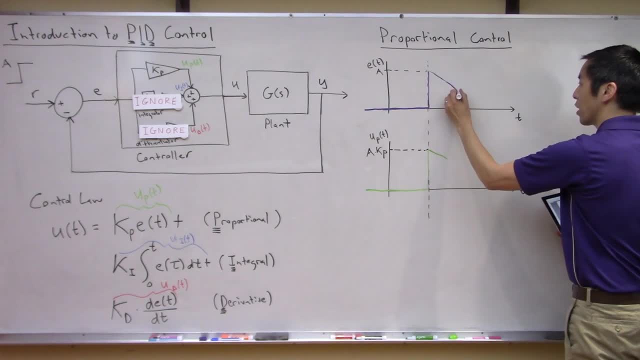 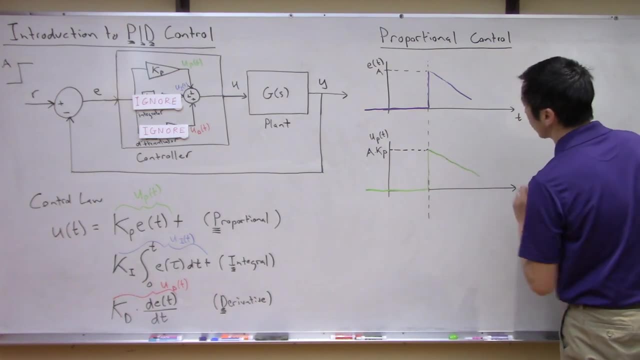 eventually, this error is going to keep going down. Hopefully, you're getting closer and closer and closer. And now what's going on is, at the same time, the control signal is getting smaller and smaller and smaller. right At some point for real systems. 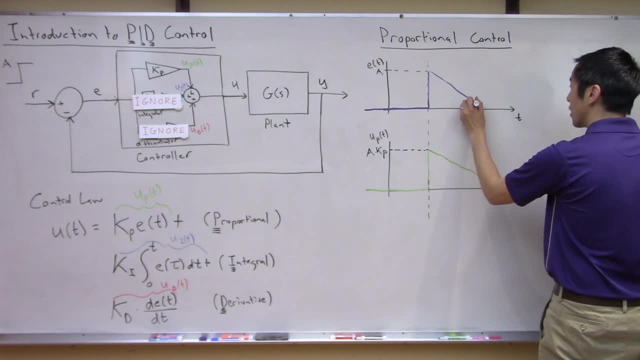 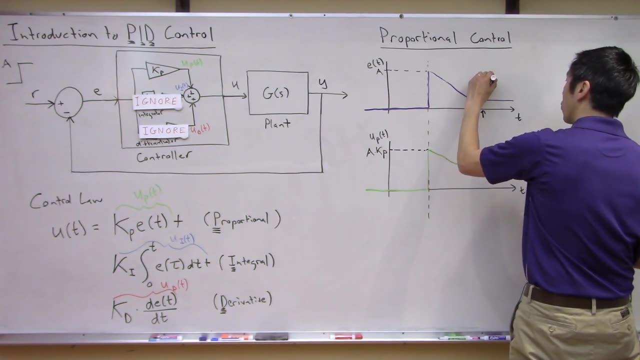 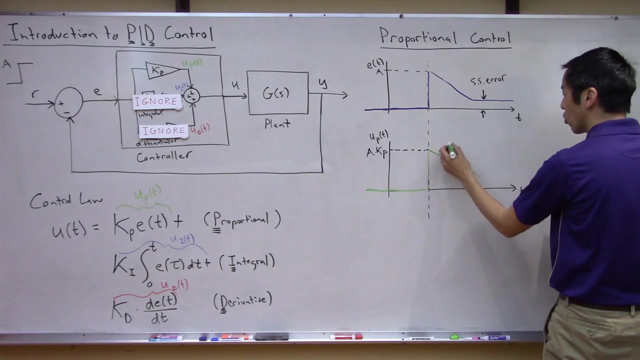 what might end up happening is you might get stuck and there might be some steady state error. And the reason this occurs, right, Is, if you think about this, what's going on is, as the error starts going down, so does the control signal right. 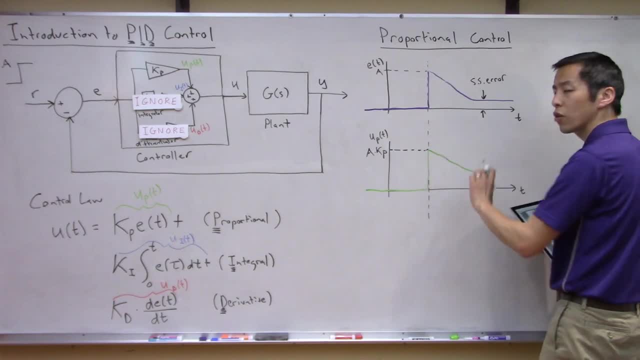 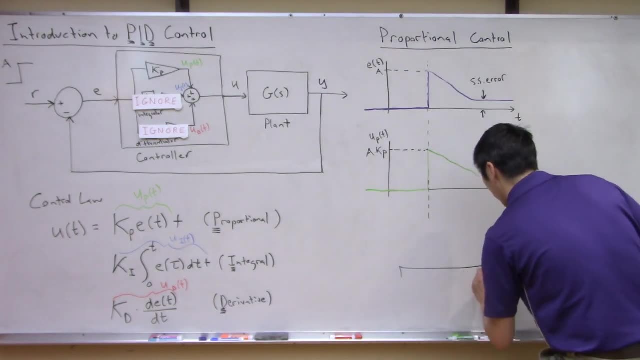 The control signal also starts going down. So the control starts getting weaker and weaker and weaker. So you're applying less and less control to the plant. So if you think about, like what if your system is a mass on some surface, right? 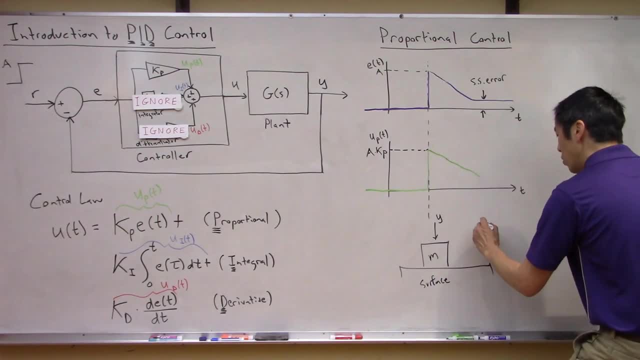 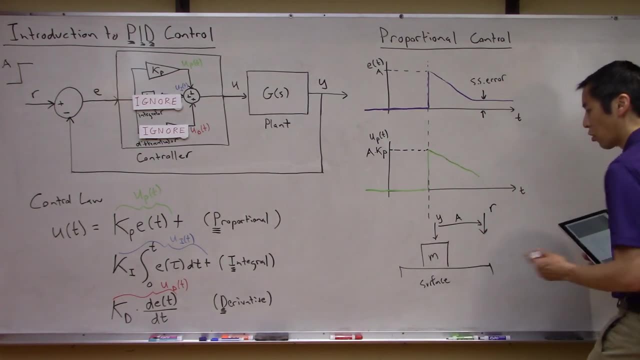 And you're sitting here at the location Y and now you want to move over here to a location R. right, There's a step input of magnitude A. right, So you are going to start right, You're going to start applying some proportional control. 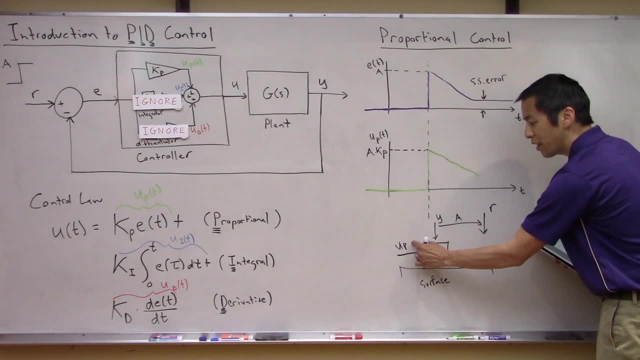 to this guy. right, And initially, when the error is large, this signal is large. So you're pushing the block hard, The block is going to start moving over and maybe it's going to get to over here, right At this point. here's your Y, here's your R. 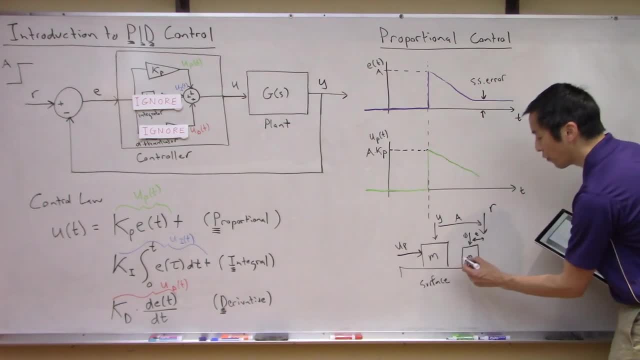 The error is now much smaller, right, So the force on the block is going to be much smaller. Do you see how, like, maybe if there are nonlinear effects like friction, right, Friction might grab the block And at some point, 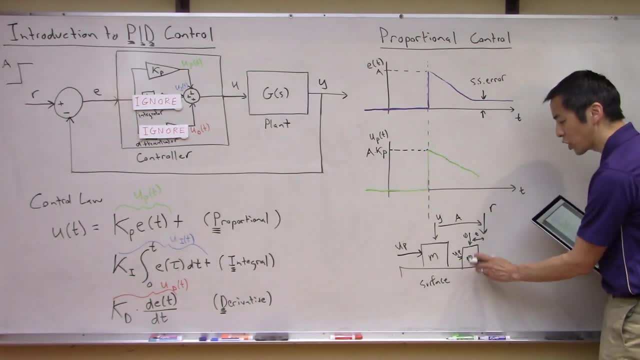 the control signal is going to be too weak to overcome friction and the block is going to stop and it's not going to move anymore. So the problem that you may see with proportional controllers is that at some point they become- basically the control signal becomes too weak. 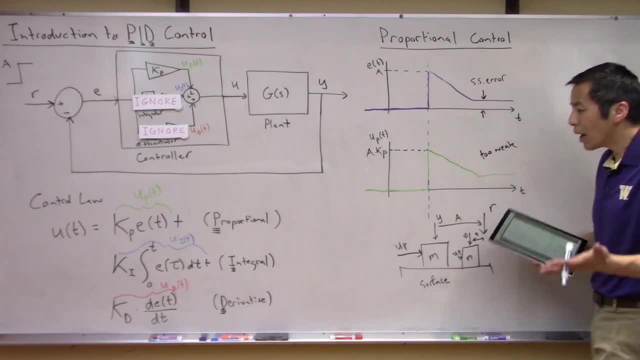 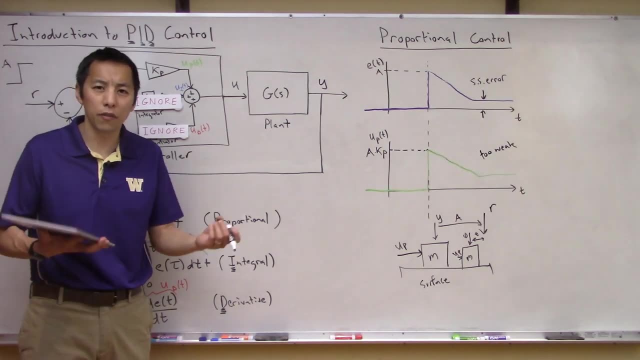 to drive the steady state error to zero, right. But it's actually quite simple though. The reason why the proportional control. it's easy to understand what's going on. We get a good feel for what it's doing. All it's doing is it's exerting a control. 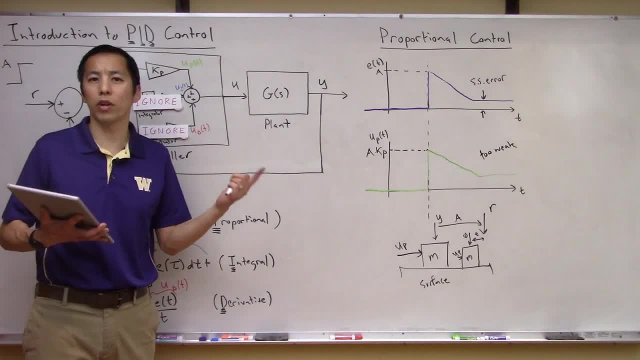 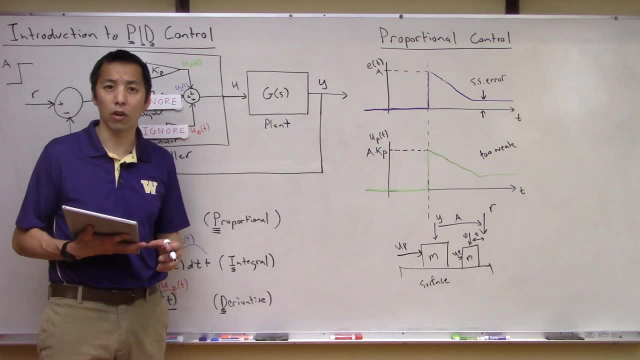 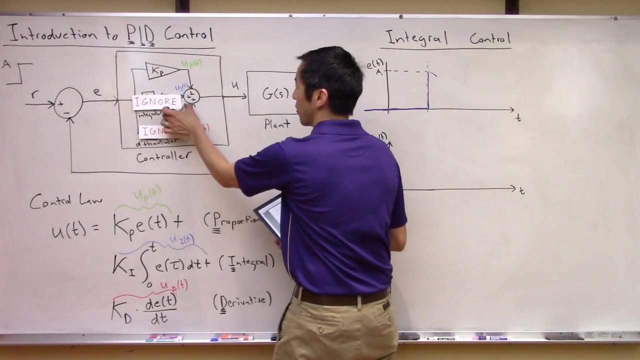 which is directly proportional to the amount of error. right, But one of the drawbacks of this is that, in many situations, a proportional control by itself is subject to this steady state error, which leads us to the next component. Okay, so let's modify our little diagram here. 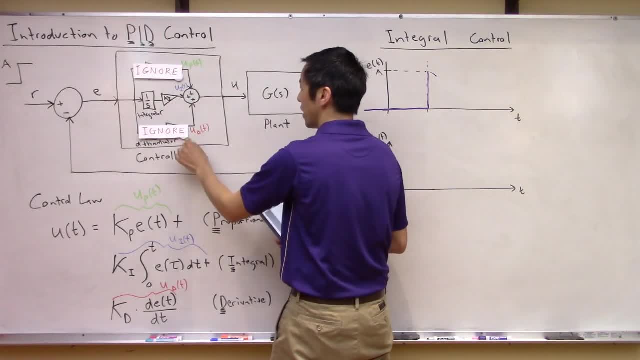 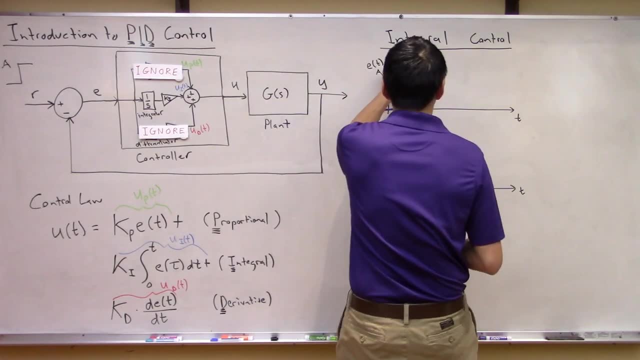 And now, instead, let's ignore KP and KD and just look at an integral term Like: let's pretend like you decided to make a controller which just has an integrator, So let's look at this integral control component and see what happens. 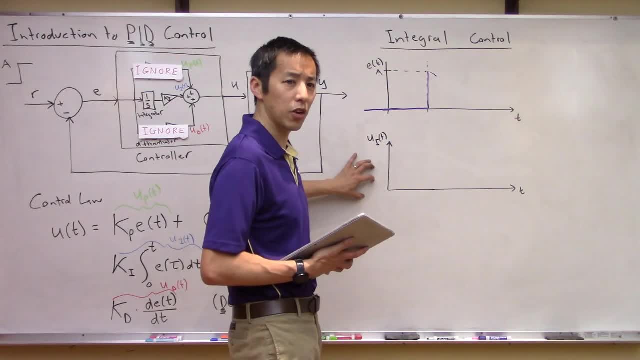 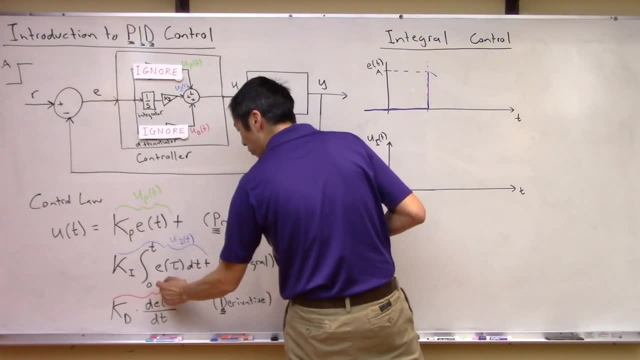 So again, we've got error on the top. And now let's ask ourselves: what is the integrator gonna do right Now? remember all this integrator does, this integral control component. it's given by this equation, right here, right. 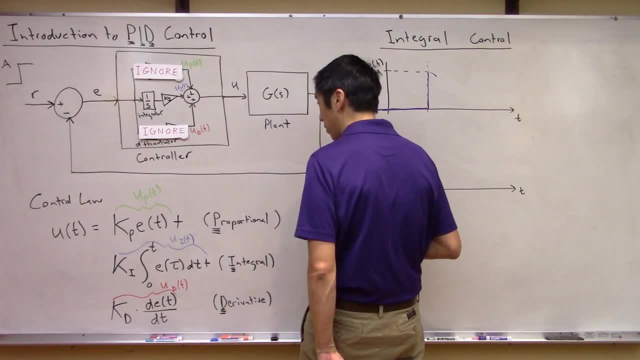 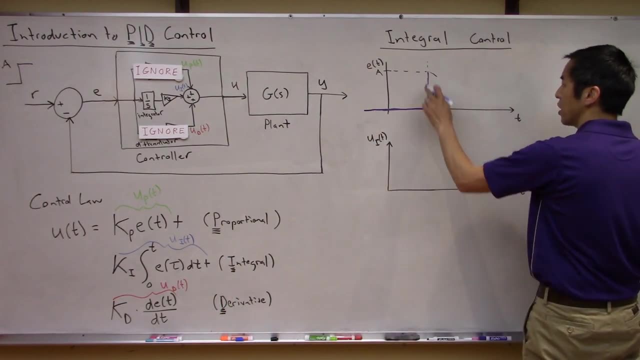 All you have to do is integrate the error and then multiply by some number- KP. okay. So let's take a look at this again. Okay, again, the error is zero, and then suddenly you give it some kind of input, right? 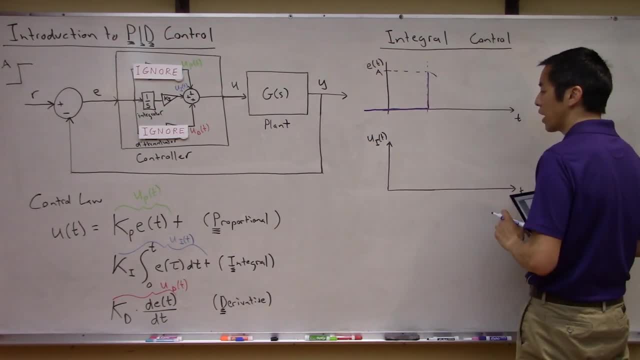 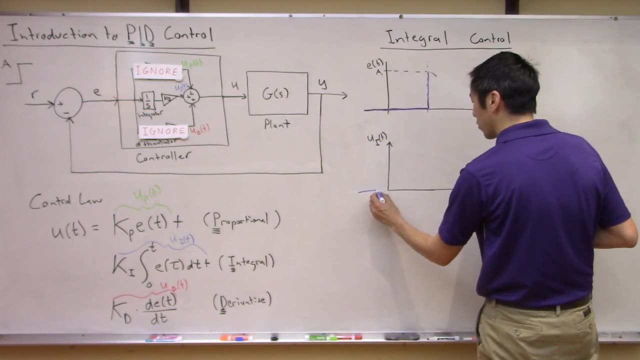 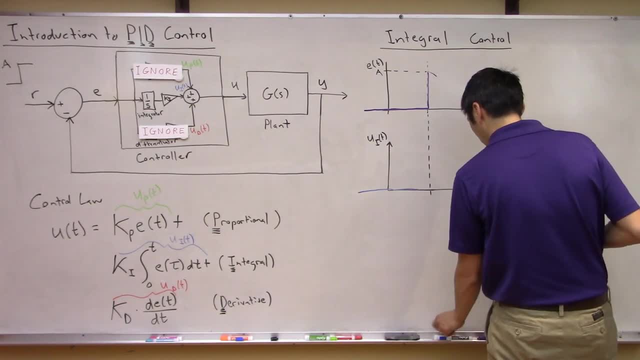 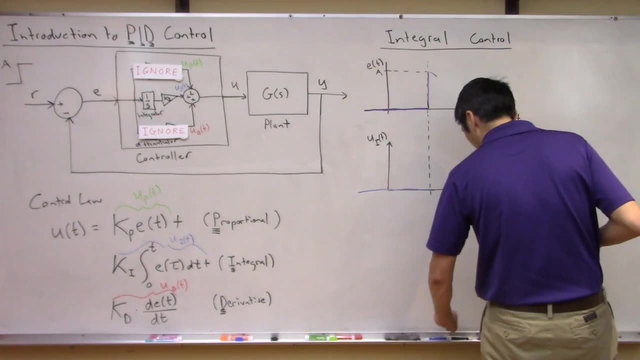 Until some action happens here. when we introduce this error step, something happens. Now we've got to ask ourselves: what is that? something, okay. So the way I like to think about this is: let's go ahead and look at a little time here, okay. 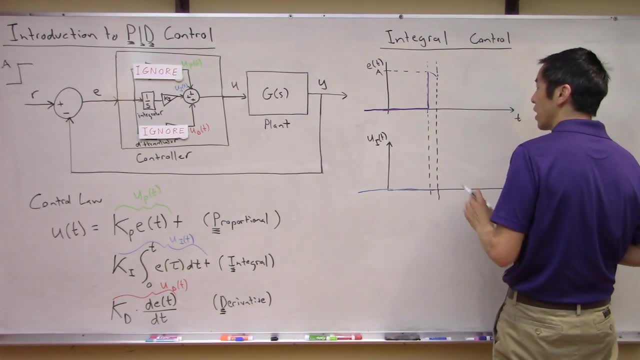 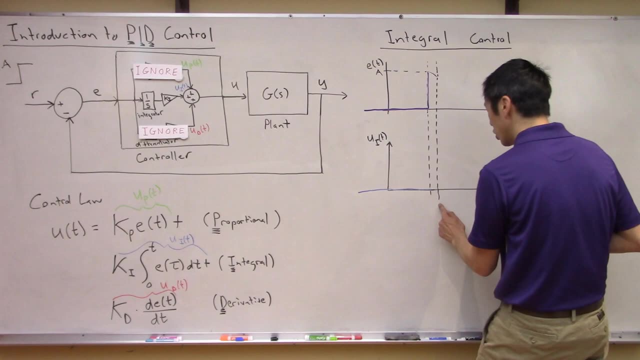 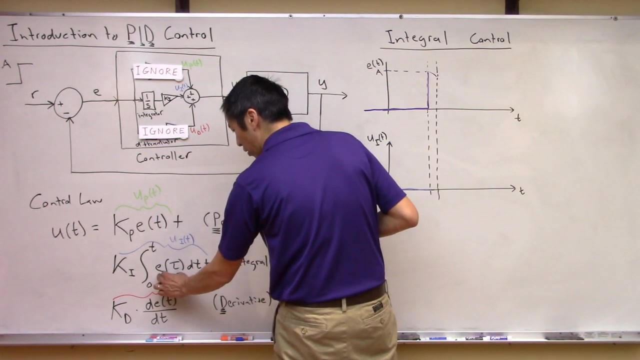 After this step gets introduced. okay, Let's say that the error signal does something like that. okay, Now we've got to ask ourselves: what is the control signal at this time? Well, the way you get that control signal at this time t is apparently you integrate the error. 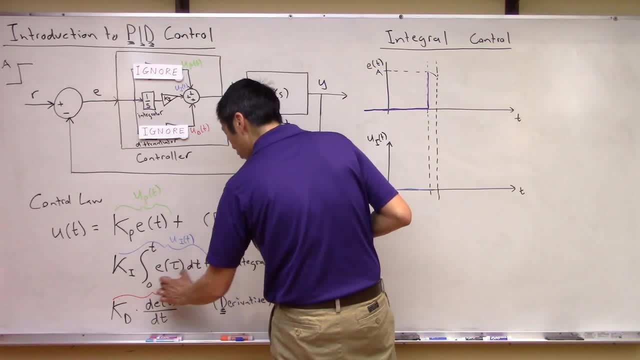 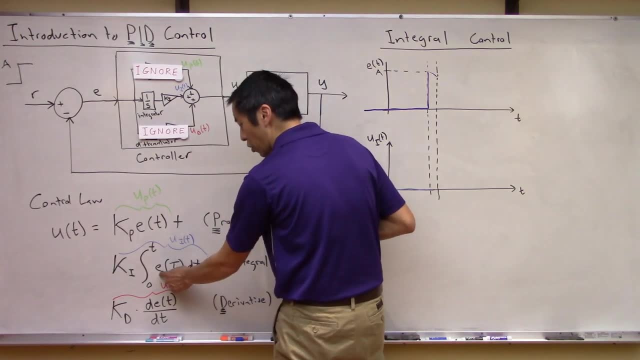 So let's just focus on this integral term. Where is this integral term in this picture? Well, again, the integral of the error signal, it's just the area under the curve of the e of t. So, in other words, it's this area under here, right? 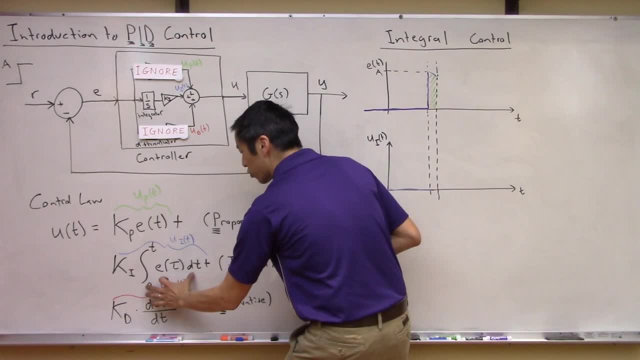 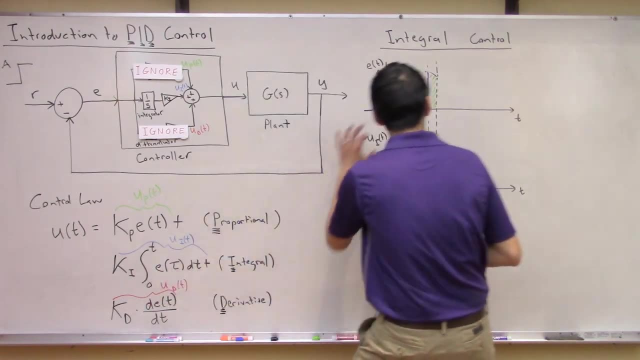 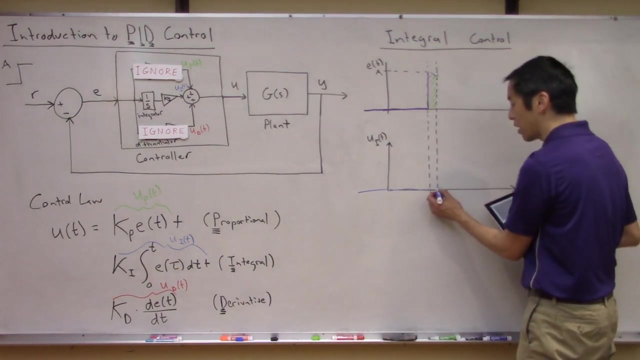 This amount of area is what this integral term is. It's how much error the integrator has accumulated, right? So that is this area multiplied by the number ki. That's going to tell you what the output of your system of the integral control component is at this time. 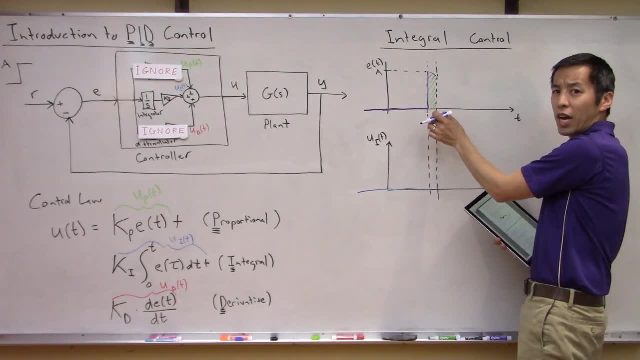 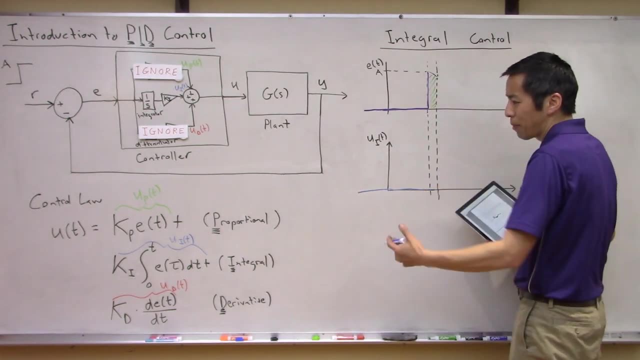 And, as you can see, because there hasn't been a large time- this area is small, right, Sure, it might have a large height, but the width is small. So this area is kind of small. You multiply it by some ki. you probably get some small numbers. 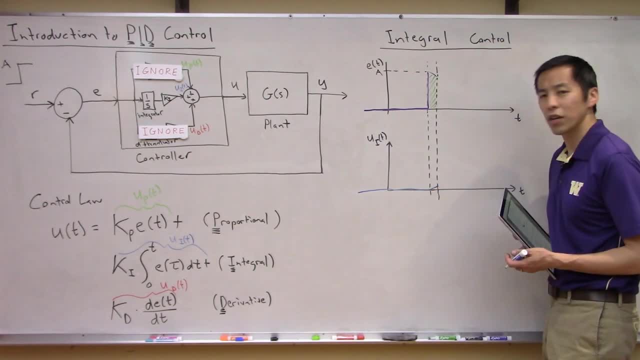 So it's probably something like this, right? So the integrator is going to do something like this. Does everyone see what's going on? right Now? all we got to do is just march along a little bit further in time, right? 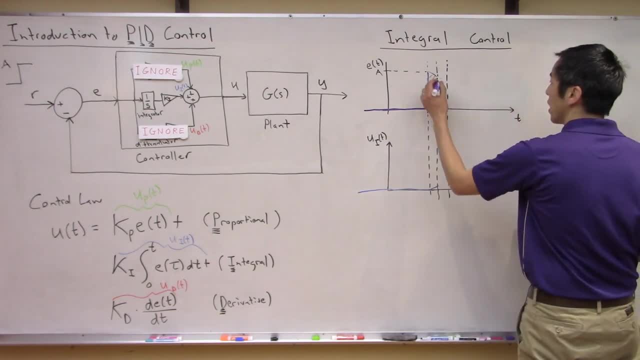 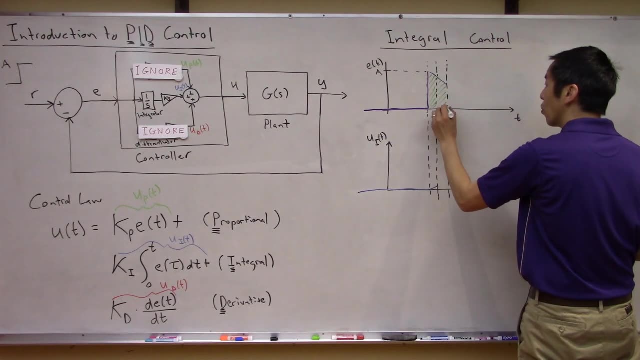 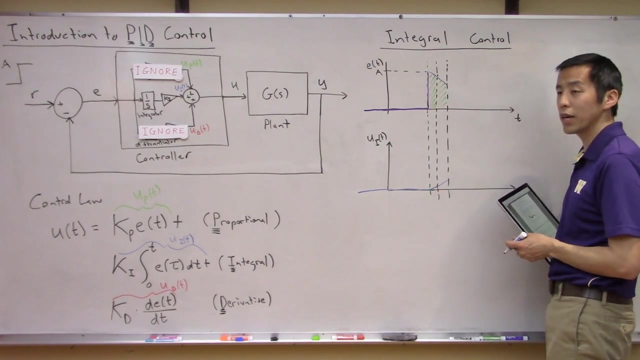 And ask ourselves the same question: right So again. maybe the error signal is doing this. right So now the total area. the total area is this: So the total area is now bigger. right, So the integrator keeps pushing harder, right. 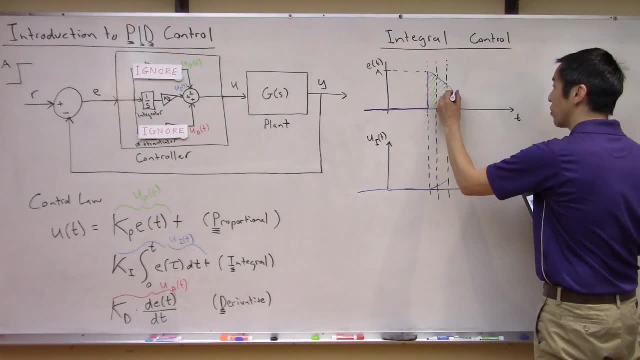 And et cetera, et cetera. You can see what this is going to be doing is it's going to keep going, And let's say that this thing goes down to here. Let's say it does this. At this point, the area looks like that, right. 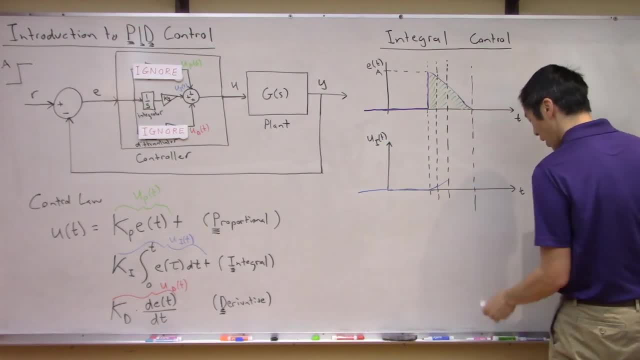 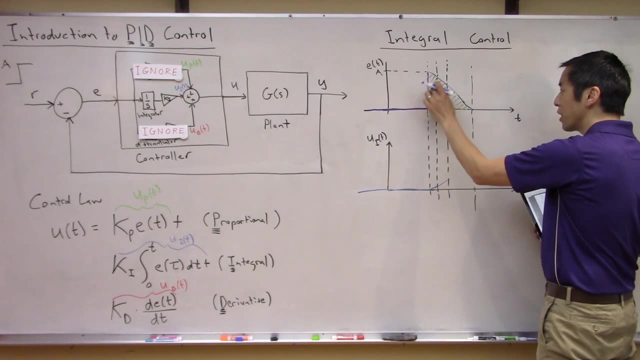 And we can trace this exact same point down And we're going to see. what's interesting is, at this time, t the integrator has accumulated all of this green area, So it's actually, you know, it's actually quite large at this point, right. 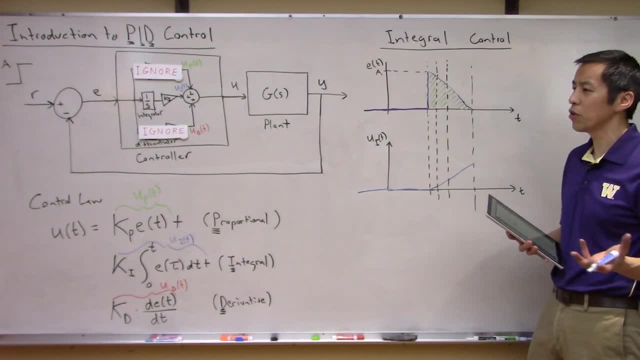 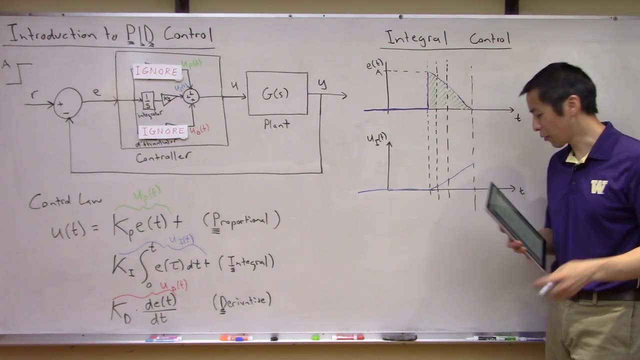 And here's the rub with integrators by themselves, And this is one of the reasons why you usually never see an integrator by itself. Think about what's happening right here. Here, everything is fine, right, This is perfect, This is what you want, right? 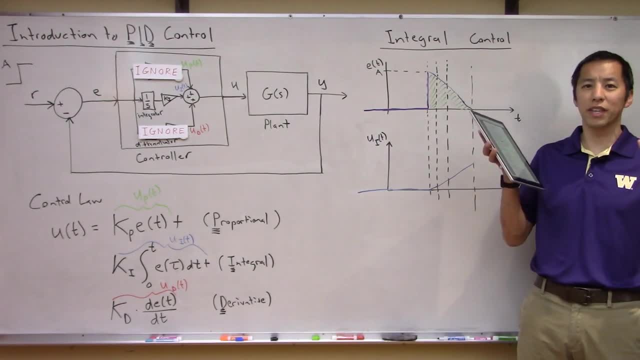 You want error to be zero. So at this point you want to just say: stop right. If your controller was intelligent, You'd be like: okay, stop doing whatever you're doing, The system is where it needs to be, Let's quit, right. 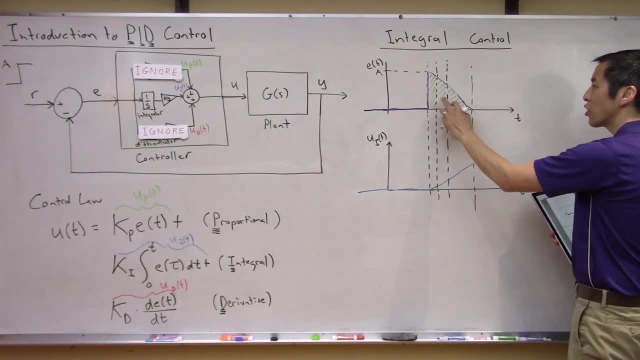 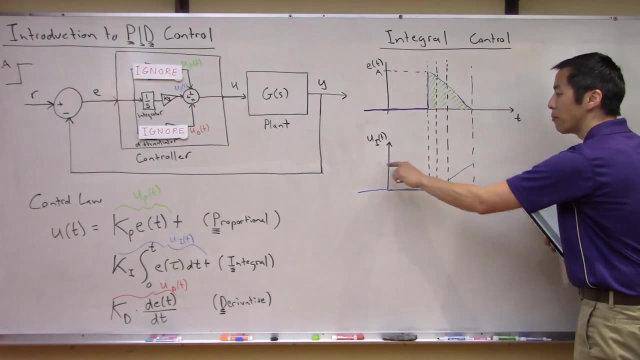 But think about what the integrator is doing right here. The integrator has accumulated all of this green area, So actually it is still pushing. In fact, it is pushing and applying as much control as it ever is going to be doing. 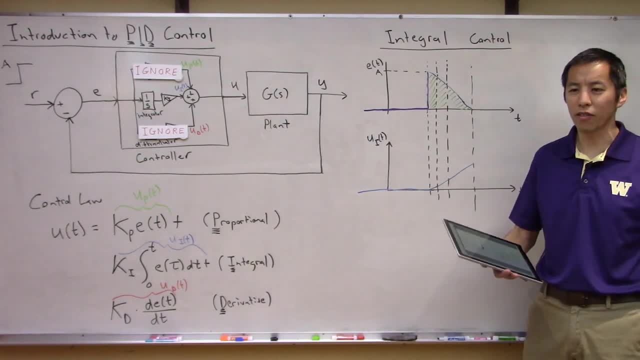 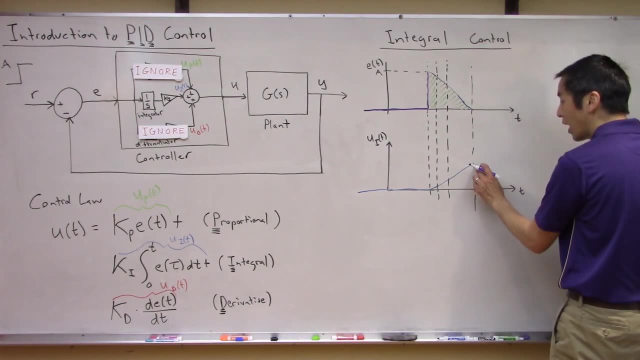 It's built up some almost like some momentum, right, It's almost got some mass and this integrator has got some momentum and it's going along. Actually, what's going to happen is it's going to keep pushing on the system, right. 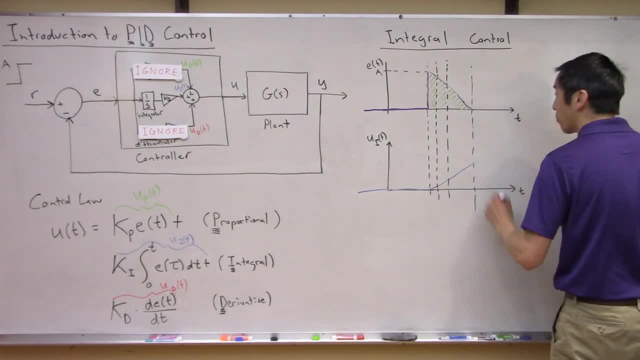 It's going to keep applying control. So the system error it's probably going to overshoot, right, The block is going to go. if this was our mass spring system, it's going to start going down. right, It's going to overshoot the system. 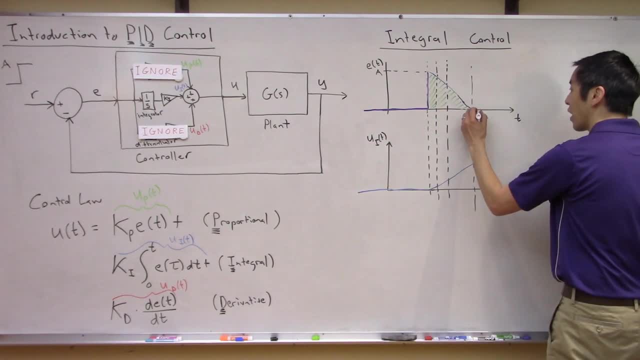 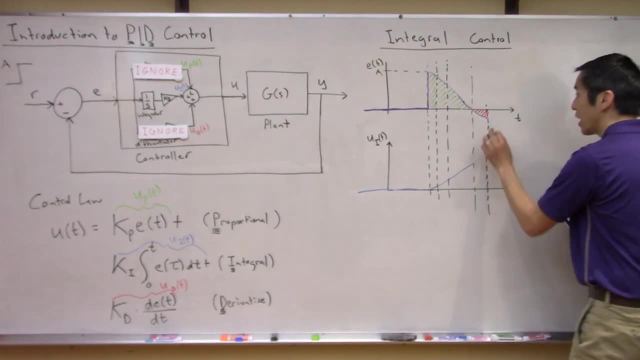 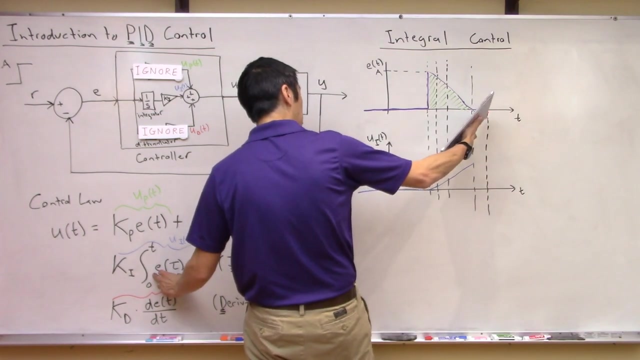 And now what you've got is you actually have negative area here, right? So again, if you think about this, what's going to happen is the error sign. The error sign changes, It becomes negative at this point. right. So now that integral in the red component is negative area. 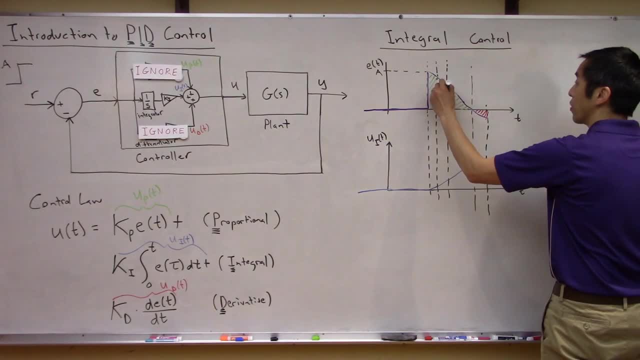 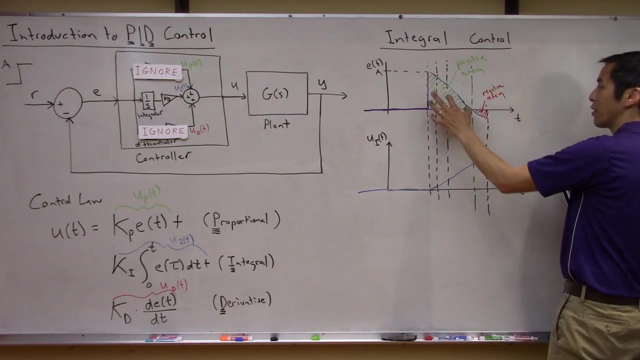 The green is positive area, So maybe let's just label it. So this is sort of positive area that the integrator has accumulated. This red is negative area, right? So what's the net between the green and the red? There's still much more green than there is red. 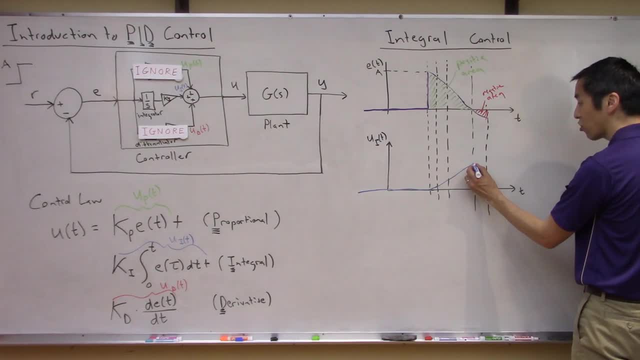 So this signal: It's going to start coming down, but it's still positive, right? So do you see what's going on? You overshot where you want it to be, but the integrator is still pushing in that same direction, right? 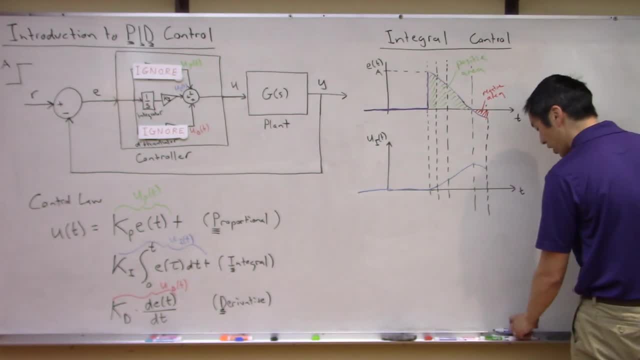 It's not pushing as hard as it used to, but it's still pushing in that same direction. So this is probably going to get worse before it gets better right, Because at some point you're going to have to accumulate a net difference between. 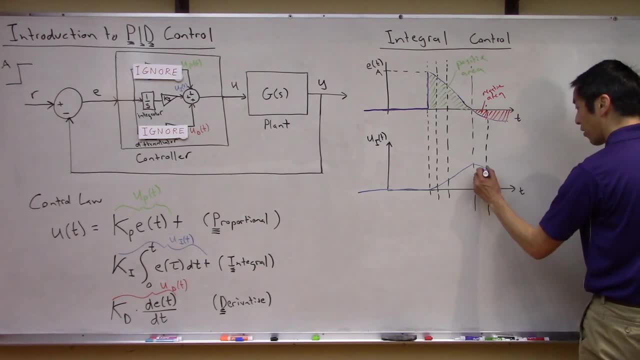 the positive and negative area, such that you get something like this right. What's going to end up happening is that eventually, this thing is going to get you zero steady state error, And that's what's actually the nice benefit of this integral control is that eventually, 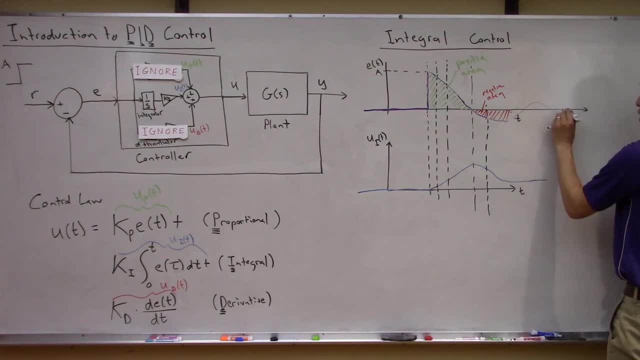 and I should make sure I draw this accurately right. Eventually, what you're going to end up with is zero steady state error. Okay, And what's going to end up happening is that the control needed to achieve that zero steady state error is going to be output by the integrator, and the integrator alone. 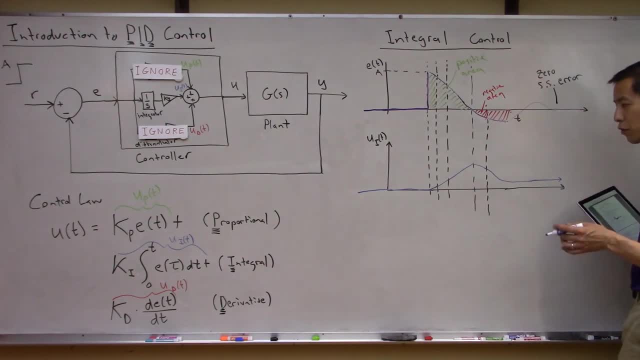 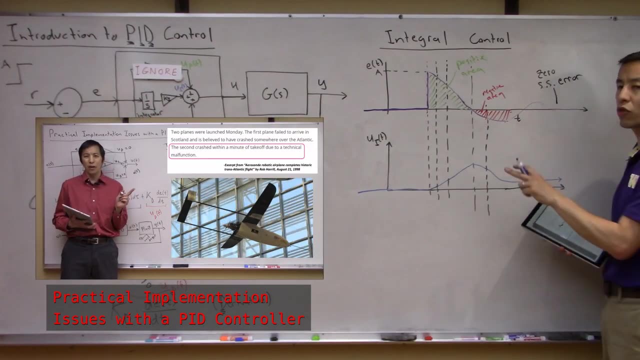 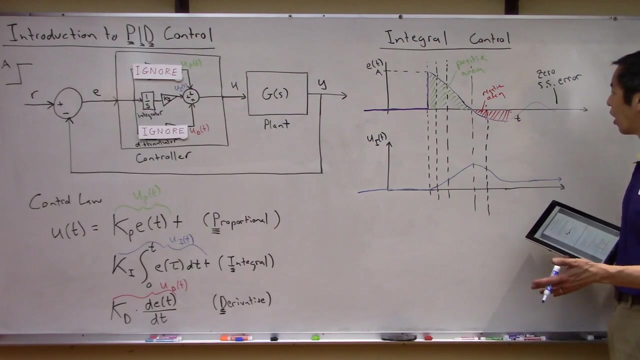 And, again, we are going to explore that statement further in future lectures, future discussions. I just want to state that right now, The thing to take away from this is that the integrator is going to eliminate steady state error. The integrator will not allow your system to have steady state error. okay. 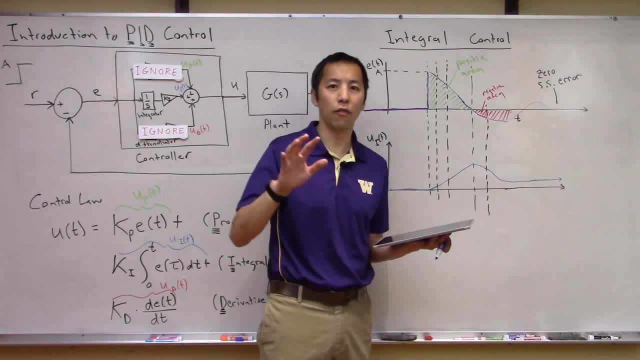 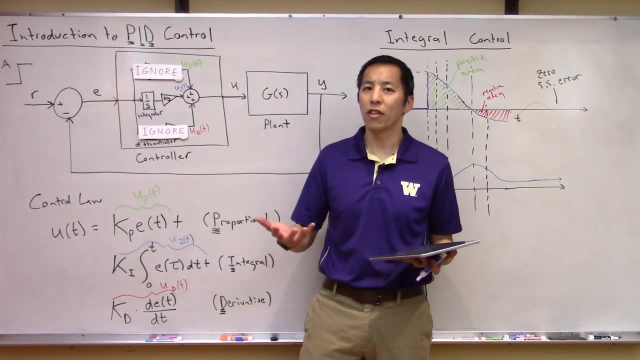 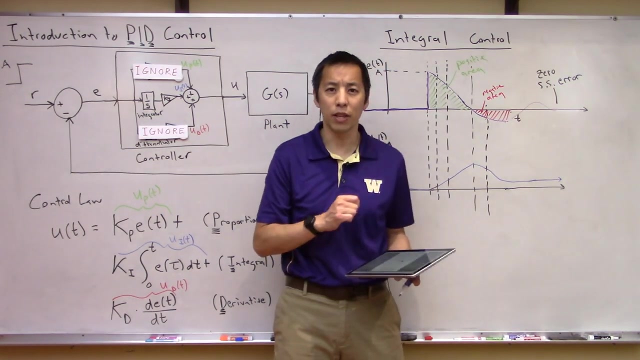 And it does so through this sort of exchange of positive area and negative area when you're integrating the error signal right And again. this is one of the reasons why often this is coupled with other components, the proportional and the derivative, to try to get rid of some of these oscillations, because 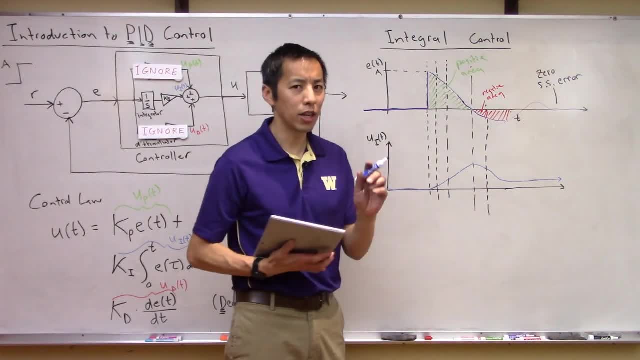 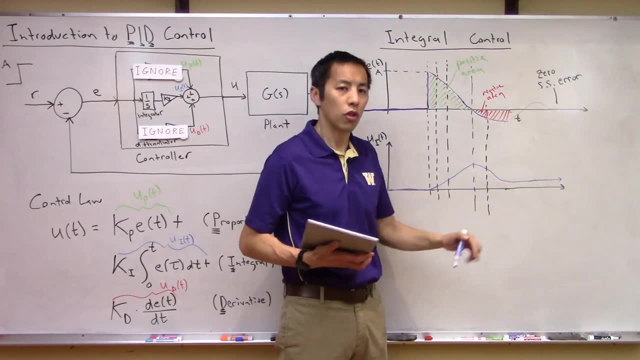 this is probably not great. Now I do want to dwell a little bit further on this idea of This claim that we made here that you're going to have zero steady state error right. The way you can actually kind of think about it and prove that to yourself is almost sort. 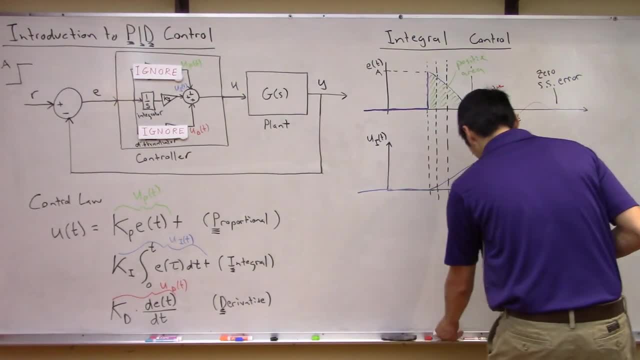 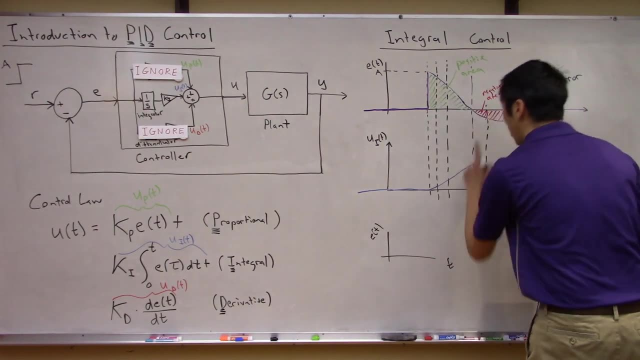 of in a paradoxical sense, right? What I mean by that is let's draw a quick picture, maybe a smaller picture of error versus time, like a smaller version of this picture up here, because it's really quite simple the idea. Let's say that this thing is doing whatever, right. 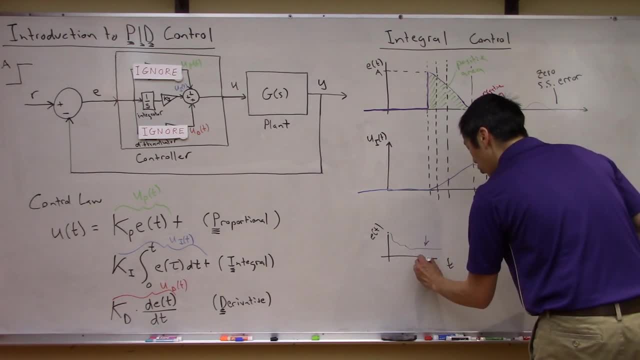 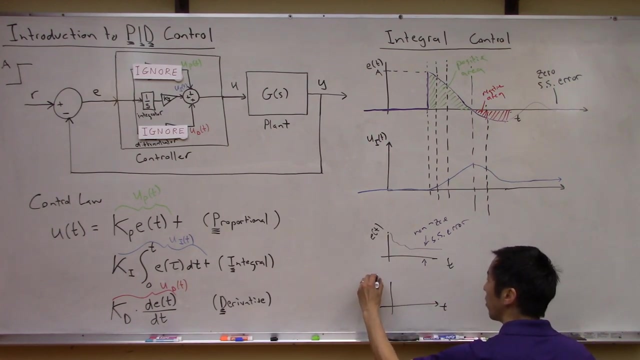 And let's say you have steady state error. okay, Let's assume that somehow You have a non-zero steady state error. okay, What is the integrator going to do in this situation? right? What does the UI component look like? 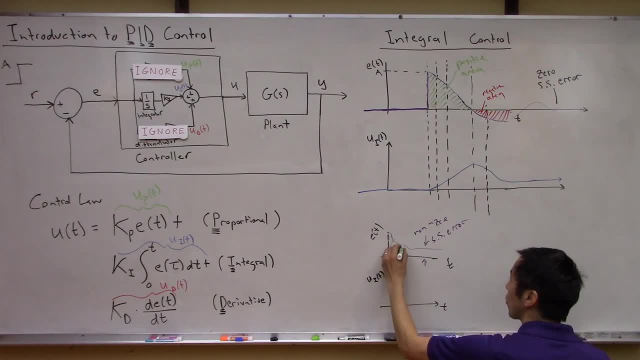 Well, according to our discussion above right, all we're doing is we are integrating the area under the curve right. So what the integrator is going to do- I think we're drawing it in blue- is it's going to do something like this and then it's going to start integrating error right? 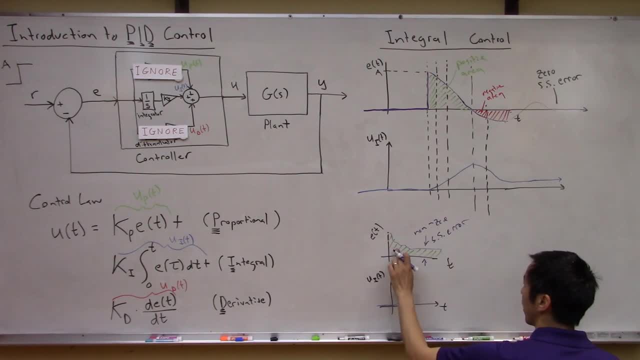 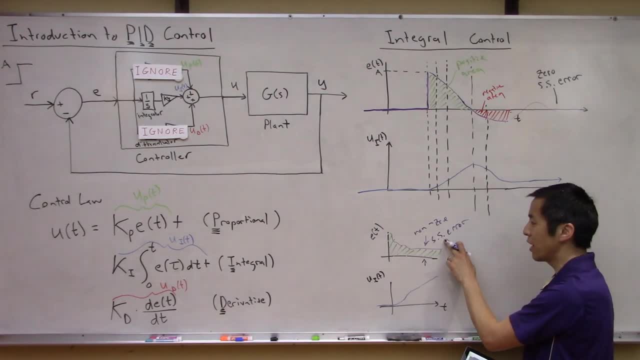 Now think about this right. If you have a non-zero steady state error, what that means is the area under the curve is going to become unbounded, right, It's going to go to infinity. Therefore, your control signal is also going to go to infinity. 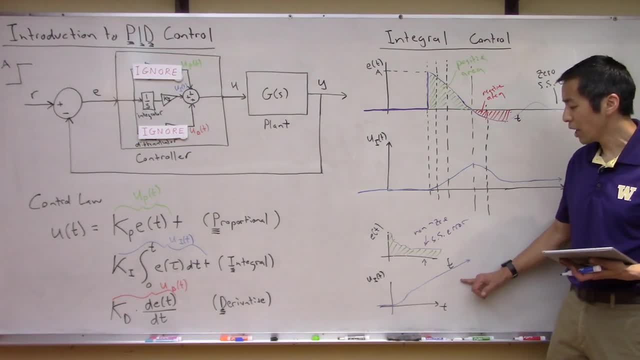 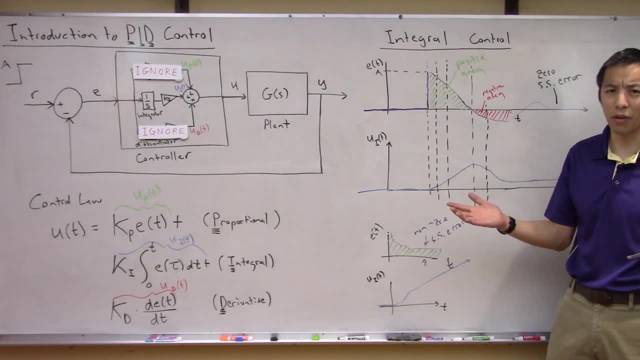 reference signal right. If it's not, you've broken something. right. Something else is going wrong, But mathematically speaking, it should not be allowed to do that right Because of this. This is a paradox, right here, right. 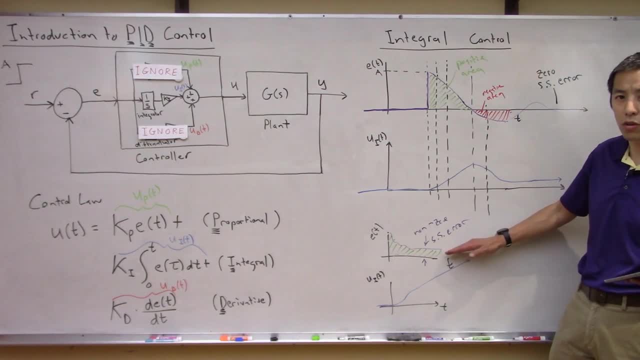 You can't have zero steady state, You cannot have non-zero steady state error, because that would lead to an unbounded, infinite, infinite control signal, which is sort of a catch-22, because if this control signal became large enough, it has to be able to eventually move this signal Y towards the 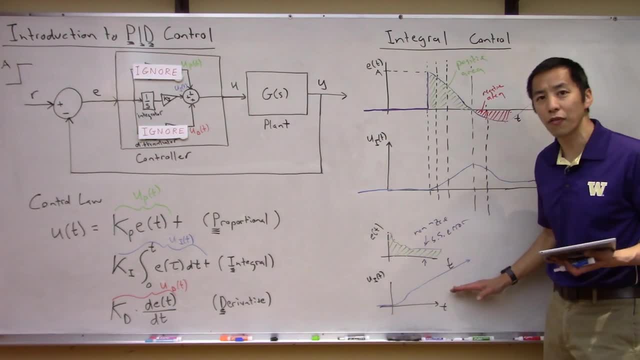 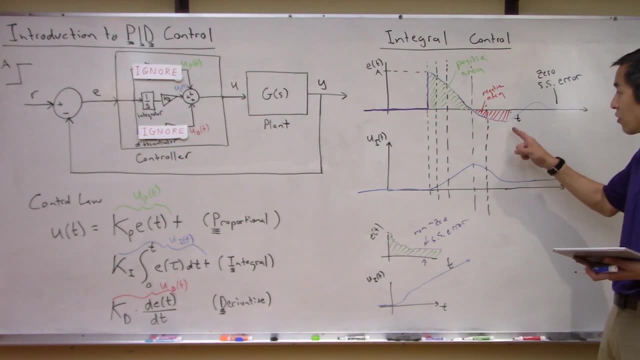 reference right. So this is one way you can kind of prove to yourself that the whole reason of adding an integrator is to get rid of steady state error. It does create some complications, like you're seeing here And again. we are going to dig into some of the complications and problems of things that 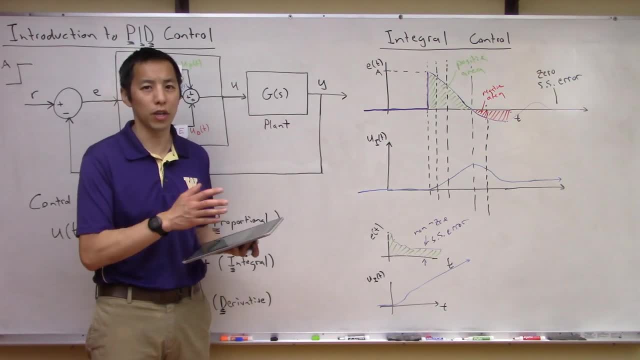 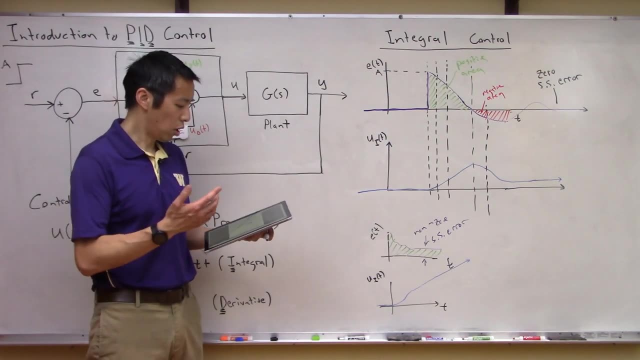 can go wrong with an integrator in a lot greater detail in a future video, But I just want to throw this out here now, just to kind of put it on your radar, so people can start thinking about this idea here. Okay, Great, So that's the integrator. 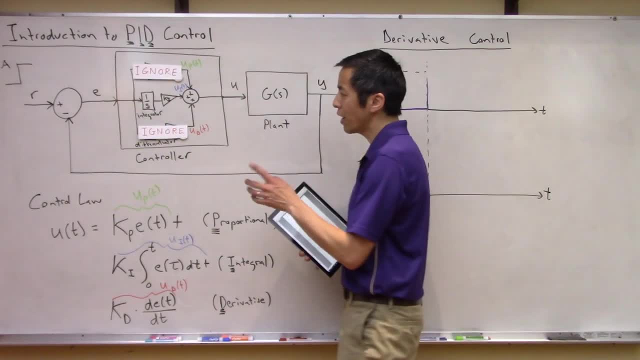 Give me a second to clean up the board and let's look at the last term. All right, So the last term we want to look at is: let's look at the derivative term. So we'll kind of ignore the proportional and the integral. 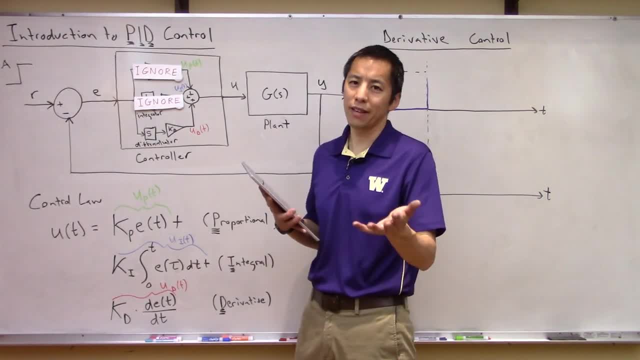 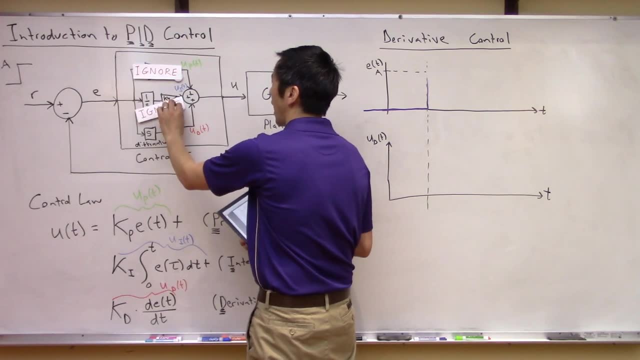 And again I'm going to say kind of, because you're going to see in a second that the derivative control really cannot operate by itself. That doesn't really make a lot of sense. So maybe, Maybe, Maybe I'm going to halfway put the ignore on these. 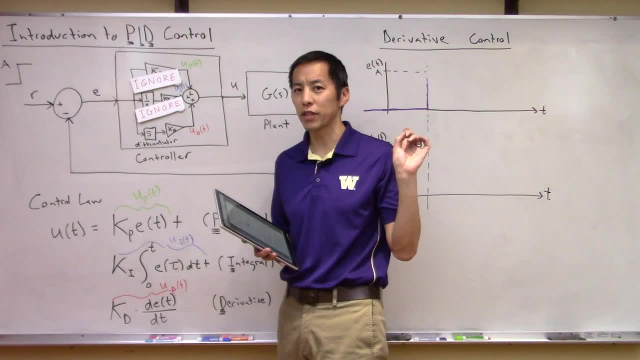 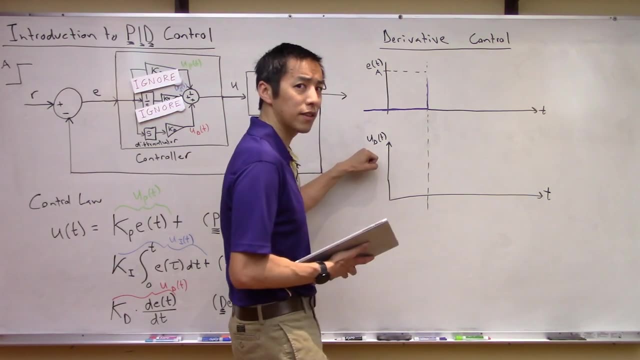 Let's assume that there are other components that maybe drive the error signal. but mostly I want to talk about what does this UD look like? So let's just look at the derivative control portion and what does the UD signal look like? Okay, So again same idea. 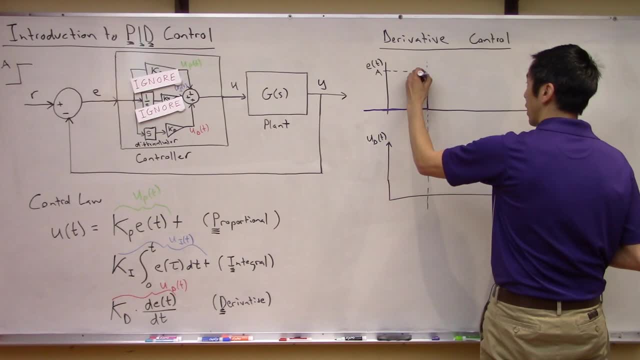 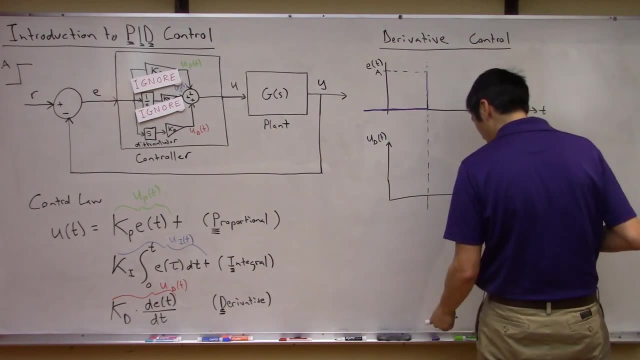 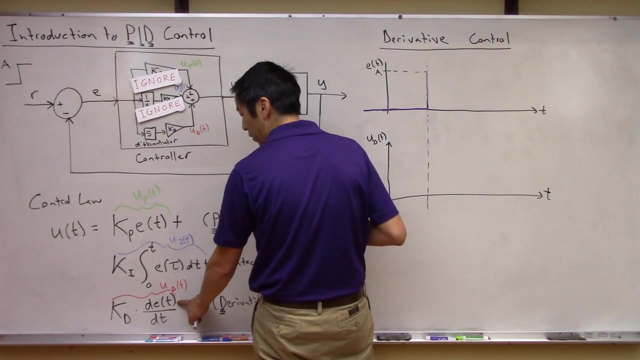 Let's presume everything is hunky dory until this time when we introduce some step in R which generates a step in the error signal. Okay, So again, let's ask ourselves: what is the derivative doing? So again? So the derivative is looking at basically the slope of the error plot, right? 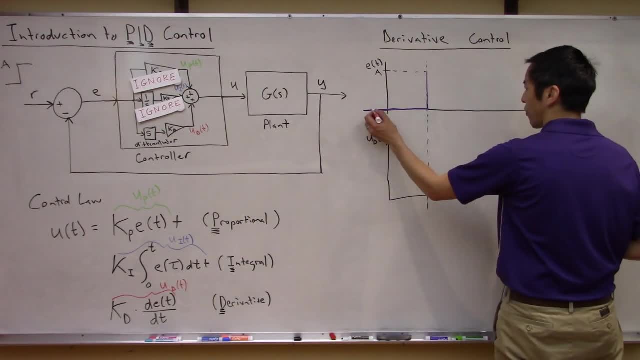 And then it's multiplying it by KD. So you look at this slope here and you're like, oh, that's easy, That's a big fat zero. So again, it doesn't matter what your KD number is. your K, your derivative gain. 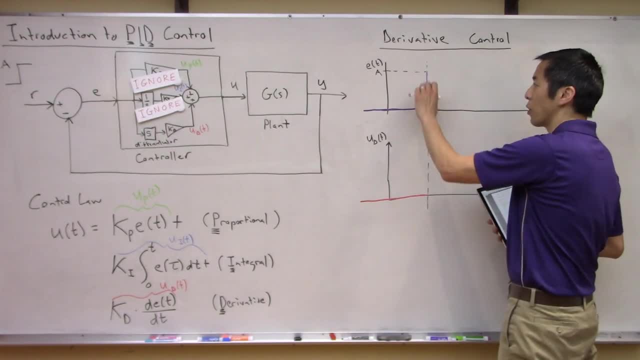 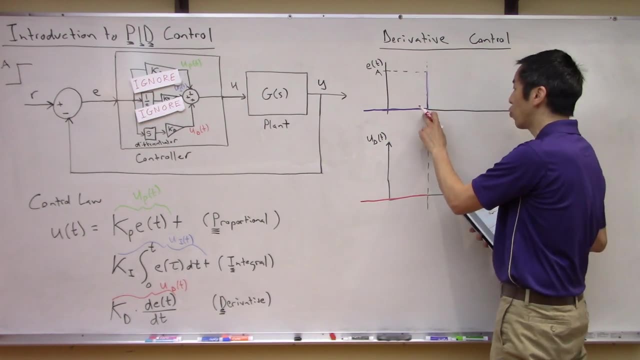 This is going to be zero. Okay, Now, at this point here, when we introduce this step, you actually see that we have a little bit of a discontinuity, right, Because the slope here is infinite, right? It just jumped from zero to something not zero. 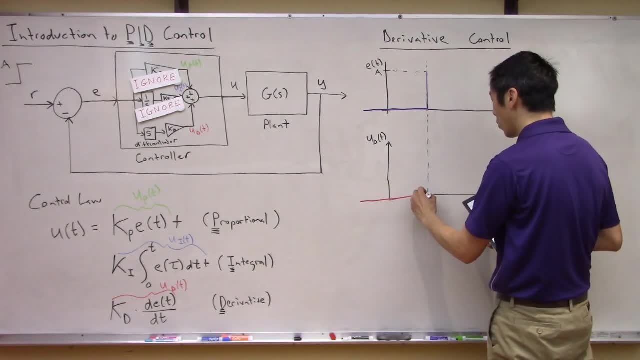 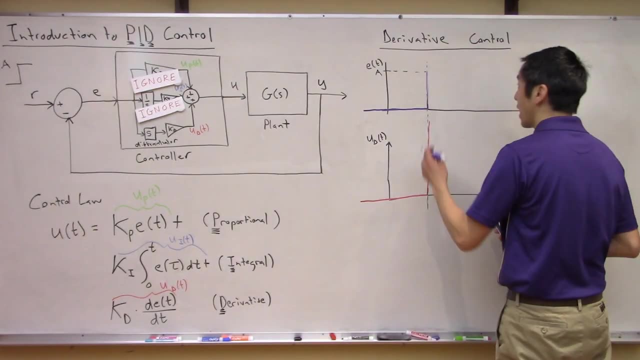 Instantaneously. So actually, the derivative control is going to be: you're going to get some spike here, right? You're going to get a giant number, Okay. And now what's going to happen is this is why, again, the derivative maybe doesn't work by: 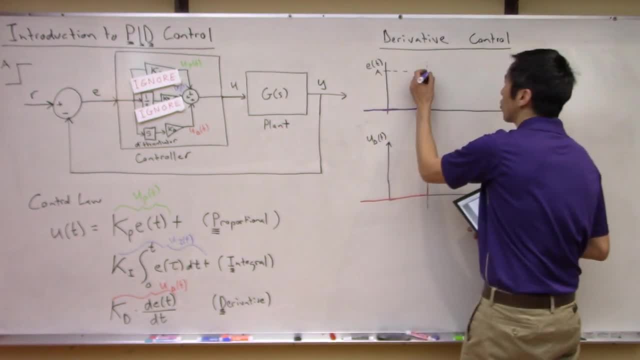 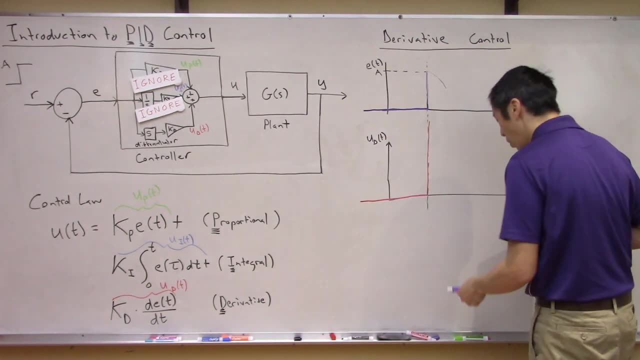 itself, Maybe the proportional control, the integral control, something starts driving the error down right. This thing starts going down towards the reference point. Okay, So now what we can start asking is: I can start looking at the slope here. So the slope here is kind of you know. 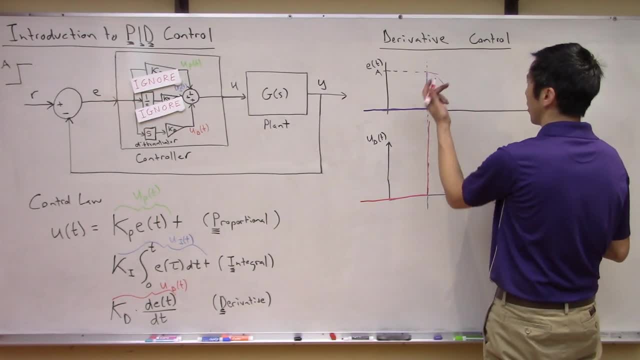 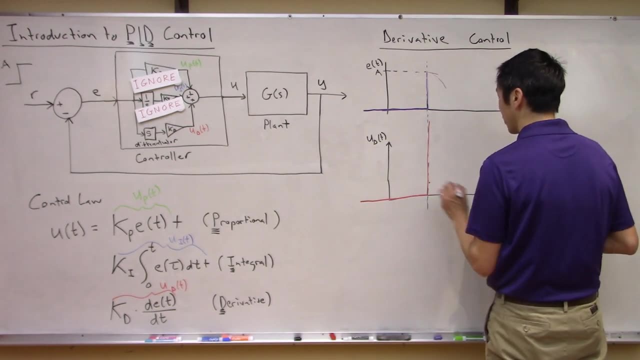 Something right And it's small. So let's just say that this is. I don't know. maybe this thing comes down nicely down to here or something like that. Maybe your KD is negative so that, even though this is a negative slope by the time you. 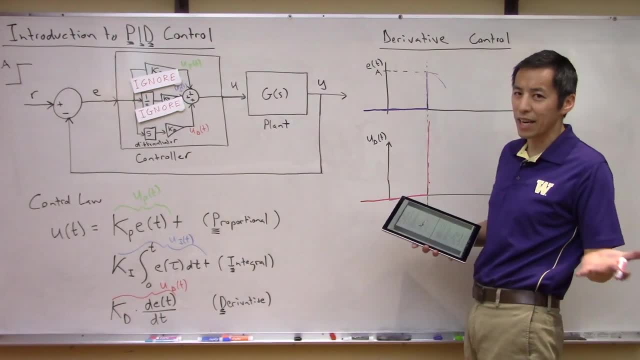 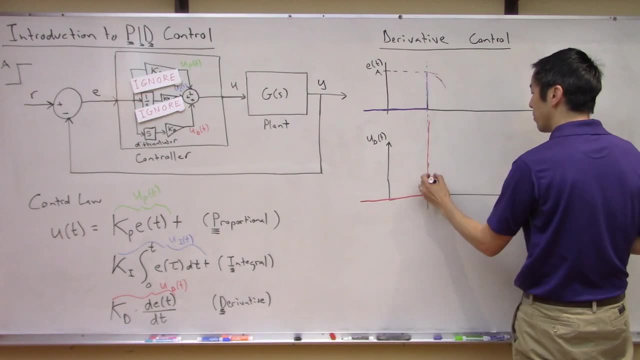 multiply by a negative KD, you get a positive UD. All right, So again, the sign doesn't really matter, I'm more interested in the concepts, right? So the idea is okay, that's like that. And then you see, here the slope is a little bit steeper. 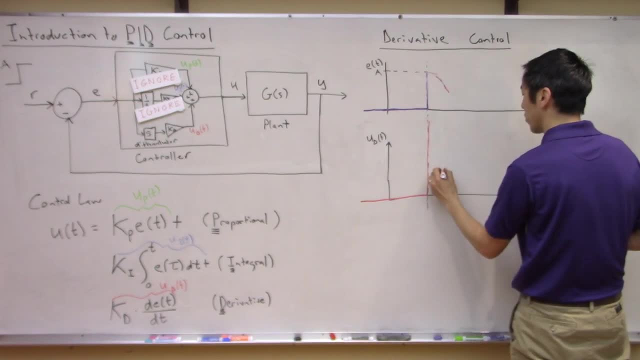 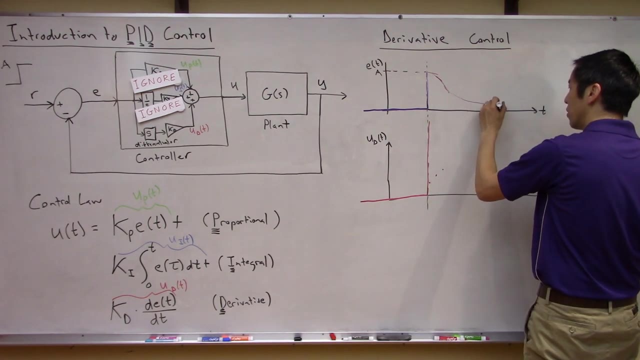 So now it's a little bit more And then it's even steeper, So you get even more. So I think everyone gets the idea right. What's happening is that this derivative signal is basically looking at the slope of the error to basically compute what it's going to do, right. 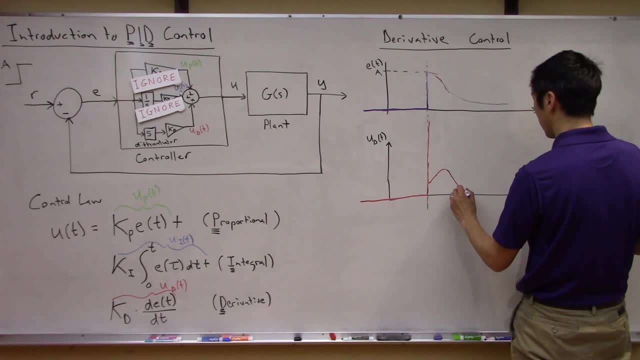 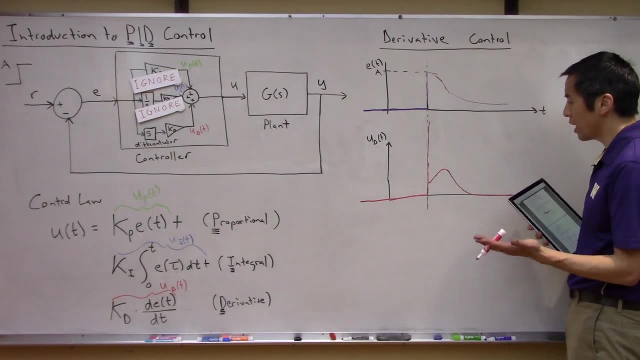 So again, I'm not a great artist, but I think it's going to you know something like this: Okay, Okay. So again, the other thing that is maybe interesting to mention here: Okay, Okay, Okay Okay. 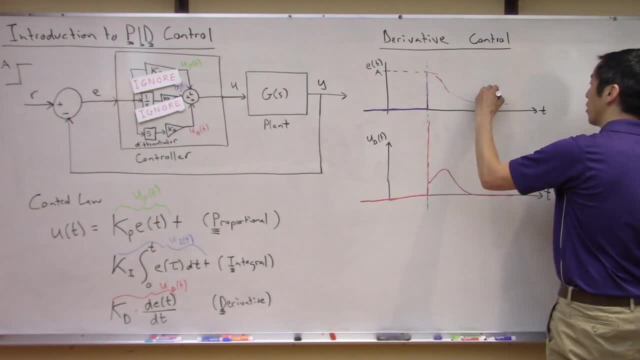 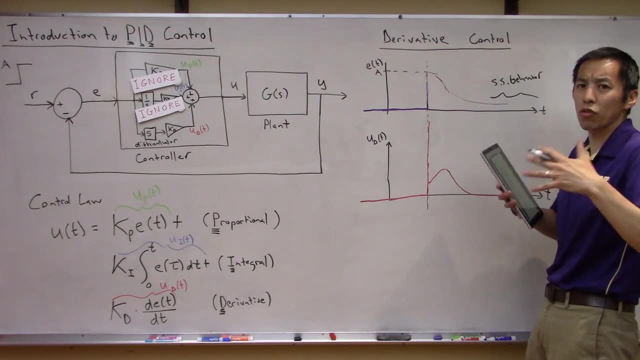 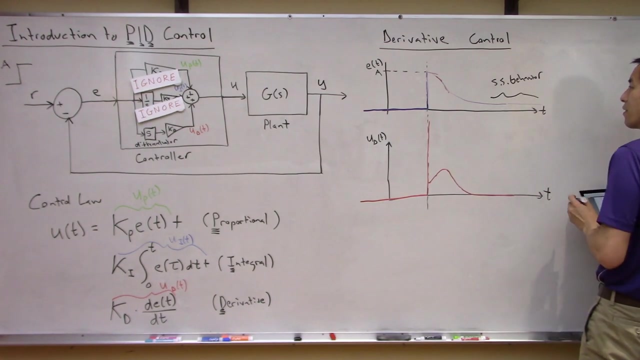 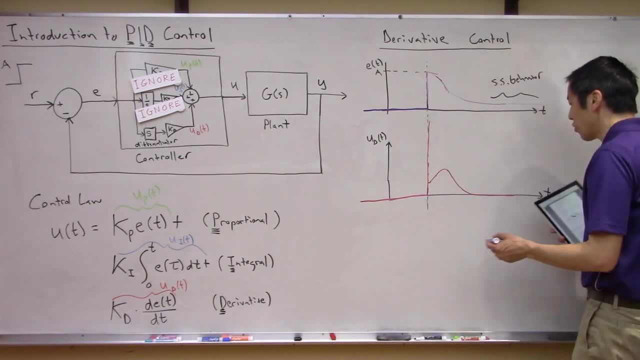 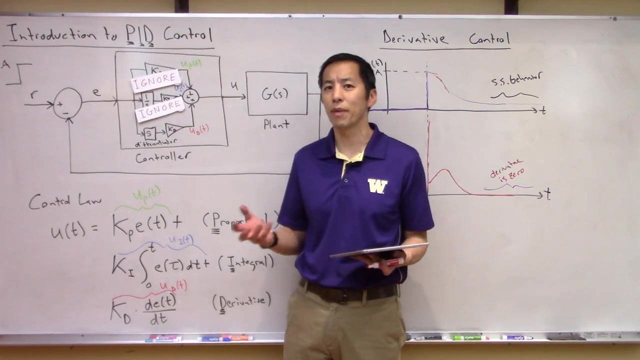 Okay, All right, The slope is zero, right. So at steady state behavior, the derivative is zero, right. So, interesting, right At steady state the derivative does nothing, right. So the derivative is really this D term. this control comes into play only when the system 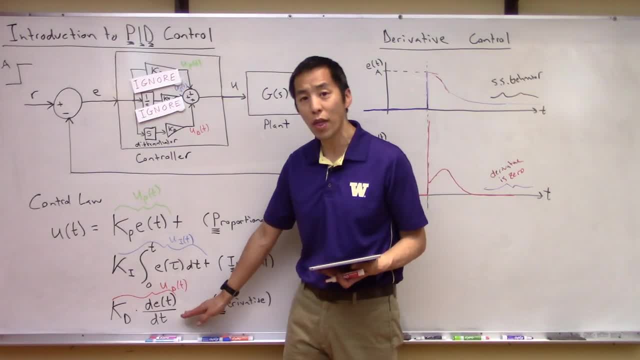 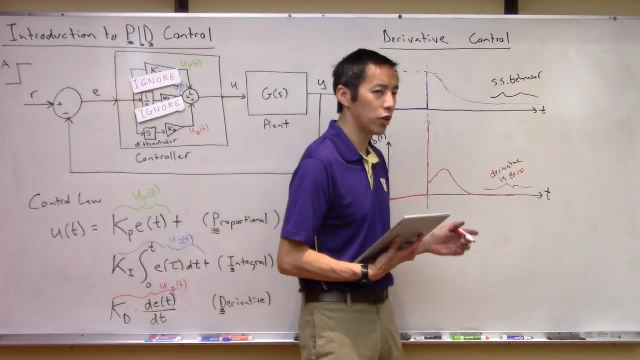 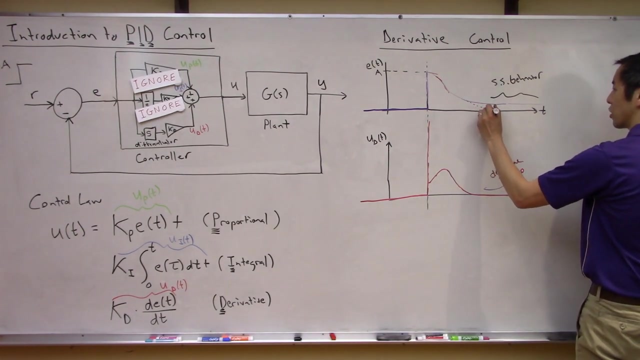 has dynamics right, When the error signal is changing, that's when this thing actually kicks in and contributes something to your overall control signal. right Now, again, you couple that with the fact, as we talked about earlier, that if you had zero steady state error, let's draw maybe an alternate signal, maybe it's like dashed right. 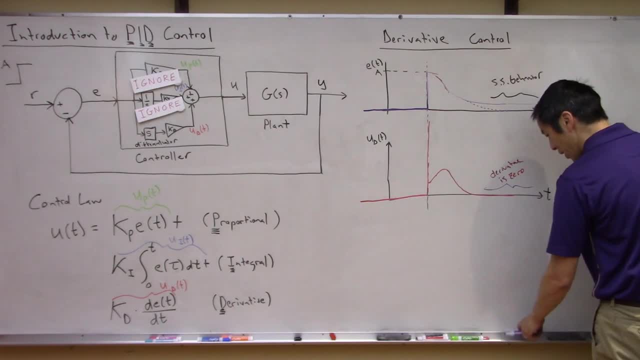 And again, the derivative would look pretty darn close here. So again, this is maybe a nice part to maybe mention: you have steady state behavior and you have zero steady state error, right? This is the picture you want, right? We want, whatever our control scheme to do, we want the error signal to eventually settle. 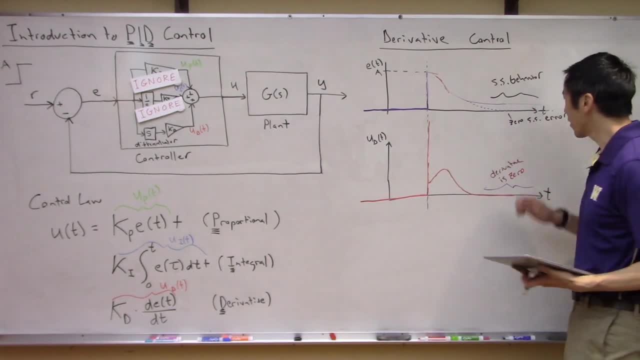 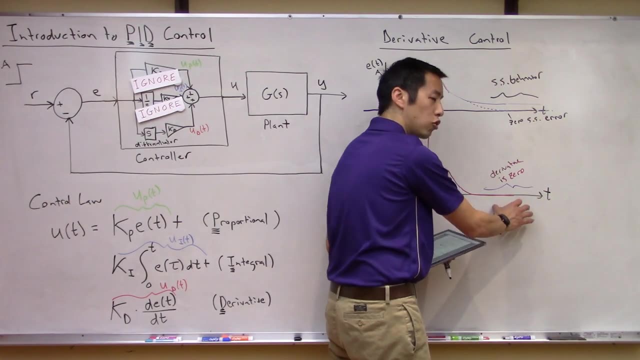 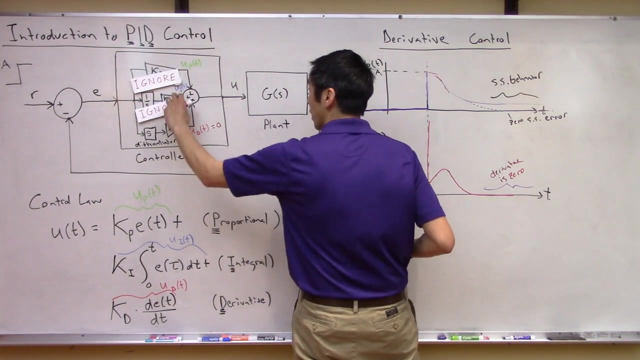 out to zero. okay, Now think about this: if this is zero, right, The slope of this is flat, so the derivative controller is doing nothing, right? So this here is basically zero. I mean it is zero, right, So this is zero. and now let me take away these, ignore things, because now, really, we 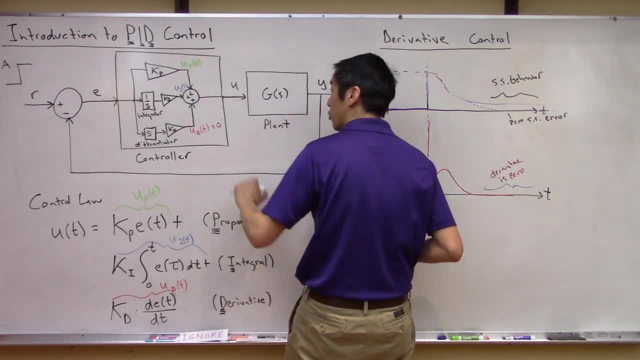 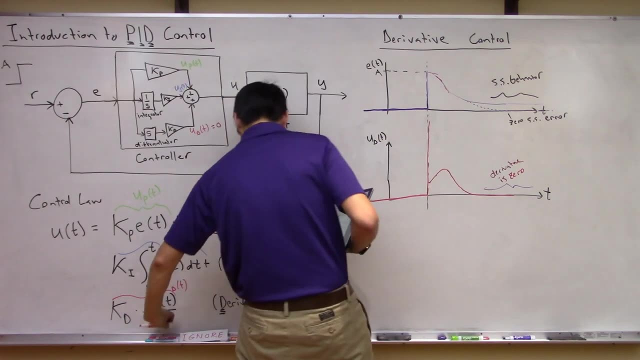 can start talking about all of these together. right, Because that's what a PID controller is- is when you've got interplay between all three of these components. right, And we already talked about the UP idea. right, The proportional part, it's just the error multiplied by KP. 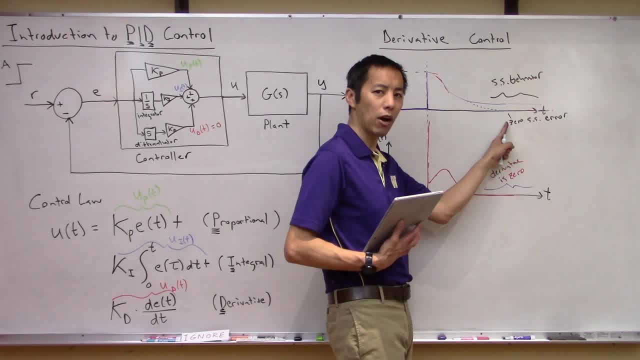 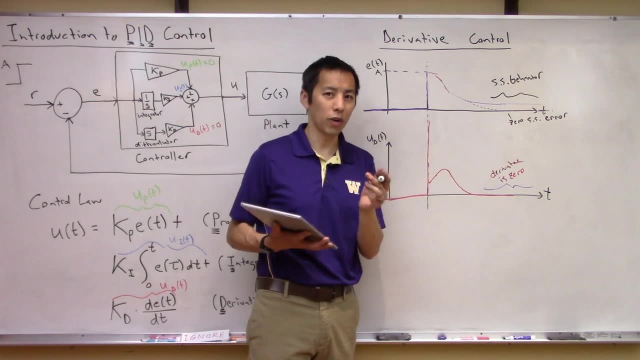 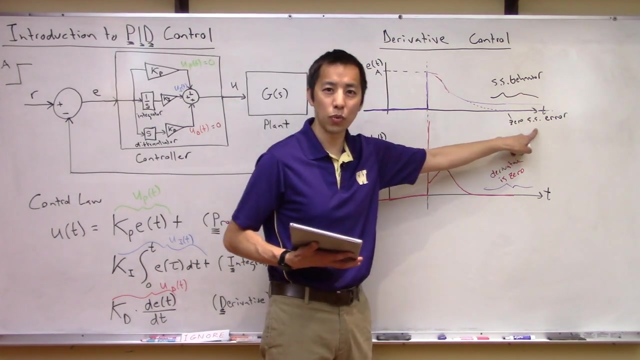 Well, if you have zero steady state error, you have zero error. so therefore this is actually also zero, right? So again, this supports what I kind of briefly waved my hands on very quickly earlier, is that in a good situation, where everything is where things are behaving the way you 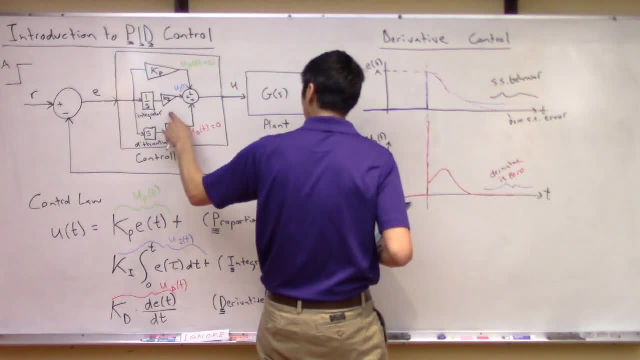 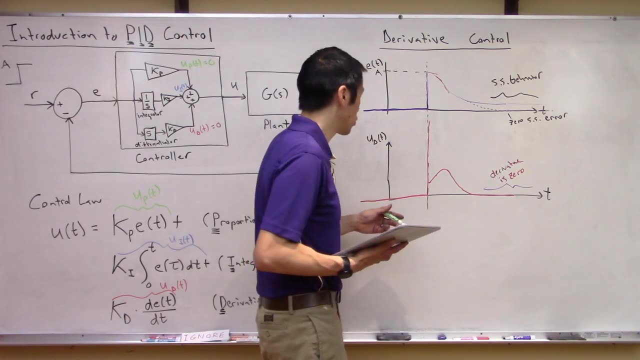 want it to. when you have this picture, The integrator is the only thing that works. Okay, It is the only thing that is non-zero, right, It is the only thing that is contributing to your controller or to your control signal in this configuration. 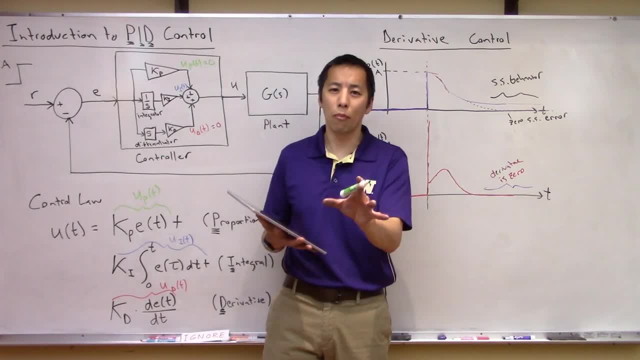 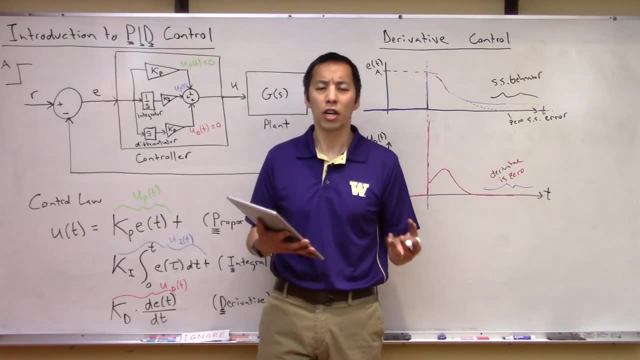 So, again, this is just. there's a lot more discussion to be had, but I just wanted to kind of give everyone some core ideas and get a rough feeling of how all these little terms contribute, what they do, what they feel like, and now the game is considering. 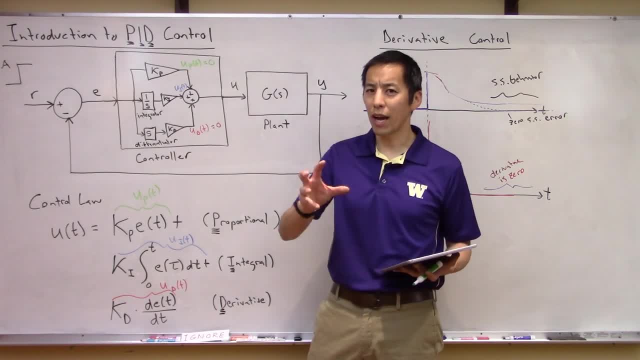 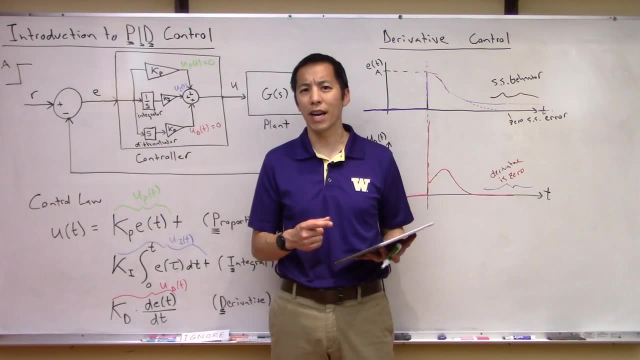 all of them simultaneously, So to maybe get a little bit more intuitive feel for what these are, Let me, let me, actually let's- jump outside, and I've got a little demo that we can look at with a physical system to see how these all interplay. 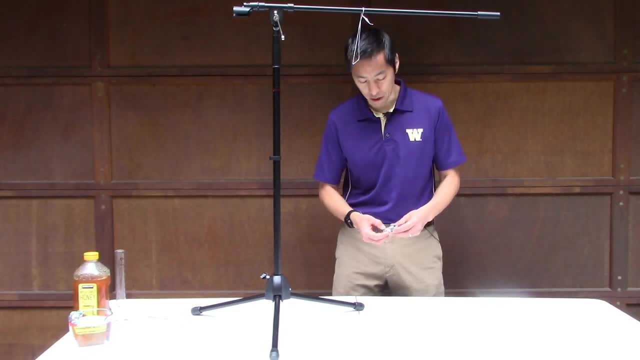 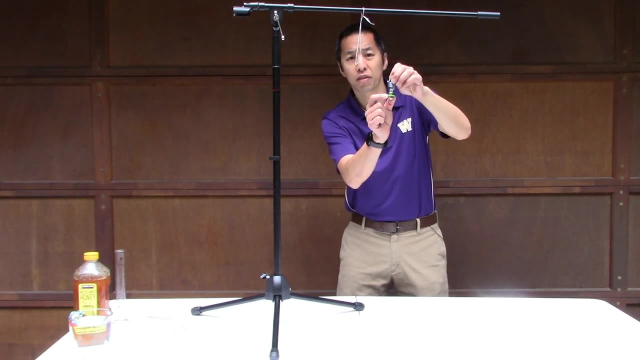 All right. so I've got a little experimental set up here and what we'd like to do is think about: I've got this little weight here and you can see. it might be a little hard to see on the camera, but I 3D printed this little green piece of plastic. 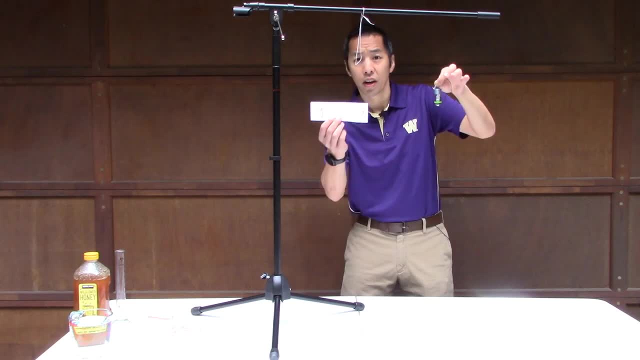 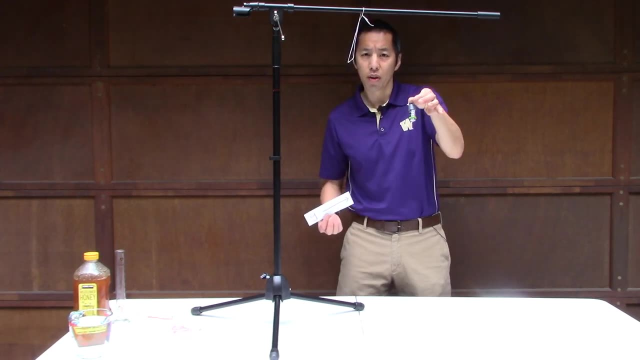 That's going to be our variable of interest. That's our position Y. So let's track the position Y of this green disc. All right? All right, All right, So now on this weight. Okay, So now what I'd like to do is, you know, let's just sit this down. 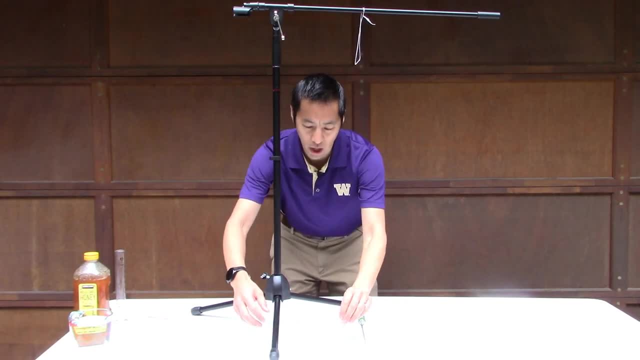 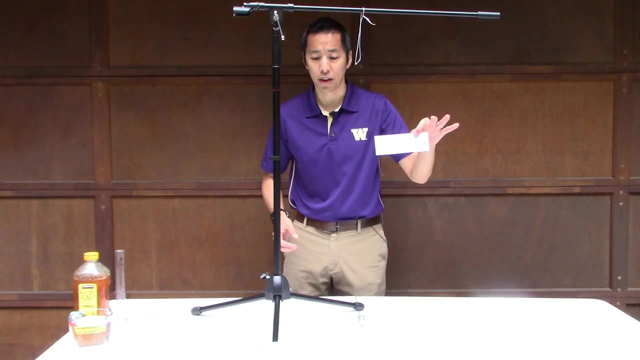 Okay, So the weight is just hanging around here and the position Y is just, you know, down here at the floor right now And again. if the reference position of where I'm trying to track is also down here at the floor, everything is fine, right. 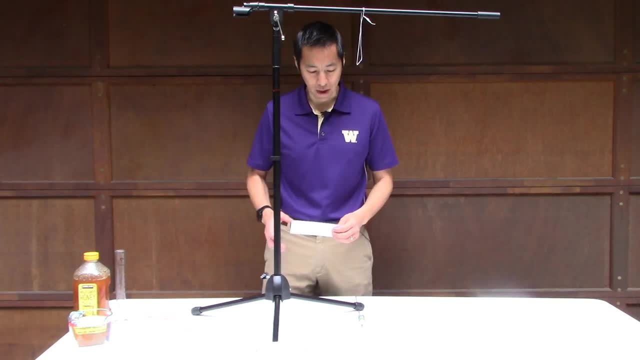 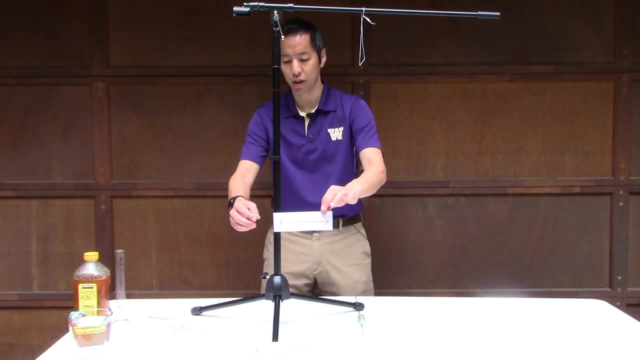 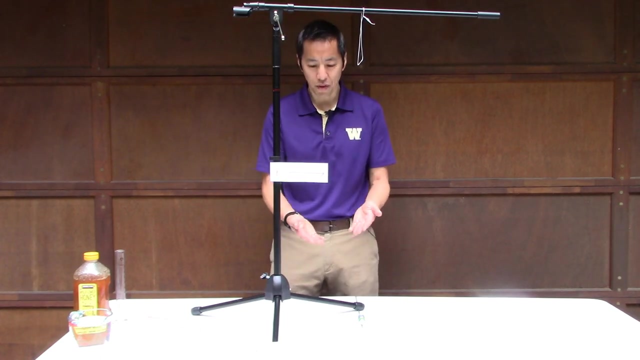 There's zero error right now. What makes this interesting is: okay if this is all, fine. what if we go ahead and change this reference position? So what if I want the reference position now to be don't know something up here, maybe right? so now you can very clearly see there is. 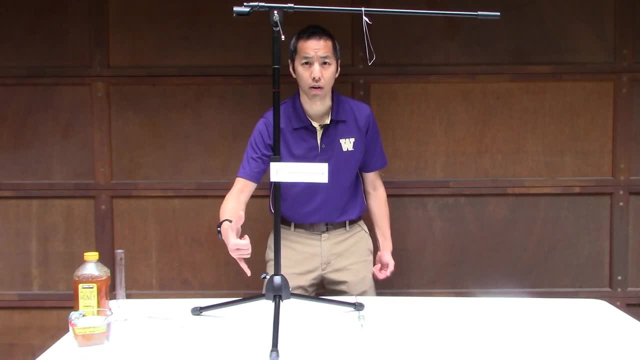 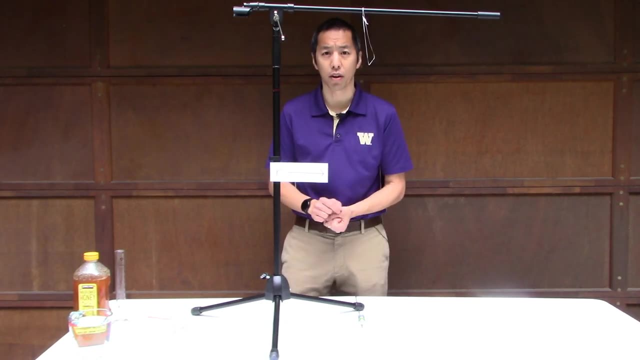 a difference between R and Y. so we have a nonzero error and now that's the job of the controller. so we need the PID controller to try to fix this error and make this error go to zero. so now, right now, you can see we have there's, there's. 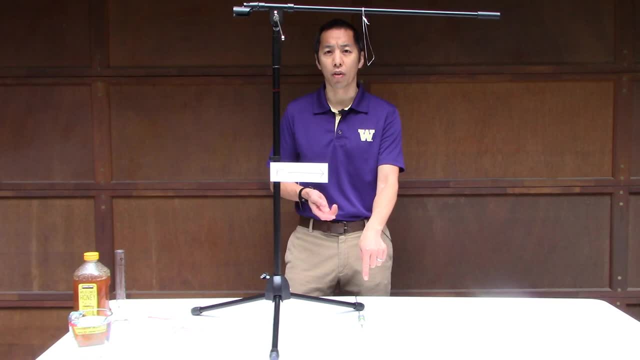 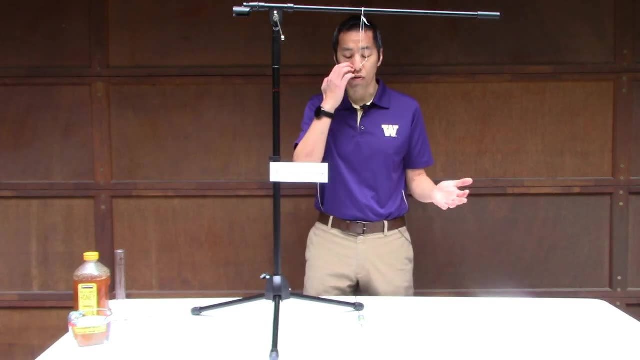 no control. the control in this case is going to be a force that we're going to apply on this mass to try to move it to this position R. so right now there's there's nothing right, there's no control input. so let's again start simple. let's start with the proportional component. so remember the proportional. 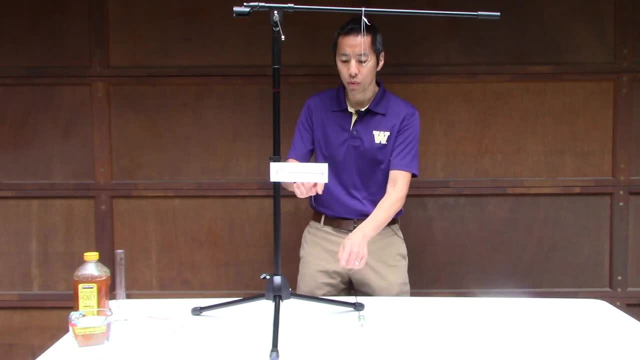 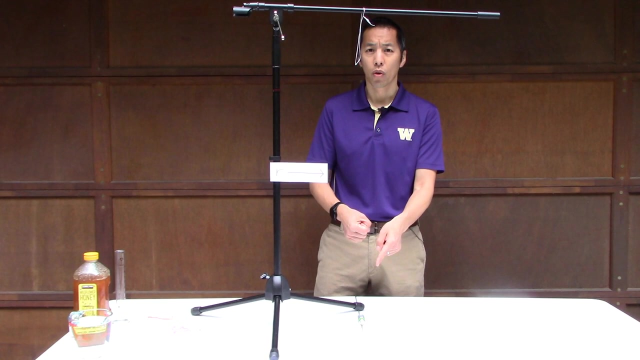 component of the controller. it's going to be a control signal which is directly proportional to this error. right, and if the error grows, then the force or the control on this is going to grow. so now you got to think: is there some kind of thing that we can apply to this mass whose force is proportional to this? 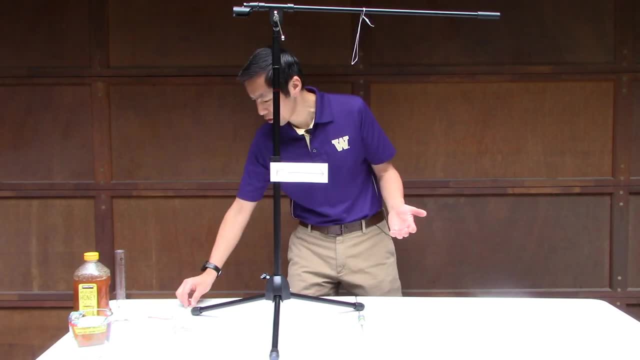 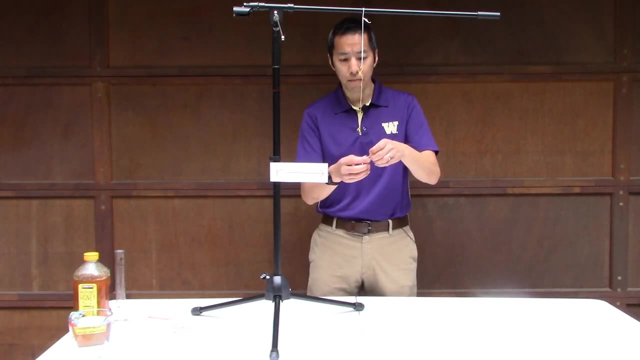 distance. that's exactly what a spring is right, or a spring or maybe like like a rubber band or something like that, right? so maybe what I'm going to do is I'm going to hook up this rubber band and I've measured this in such a way that, again, we need this to 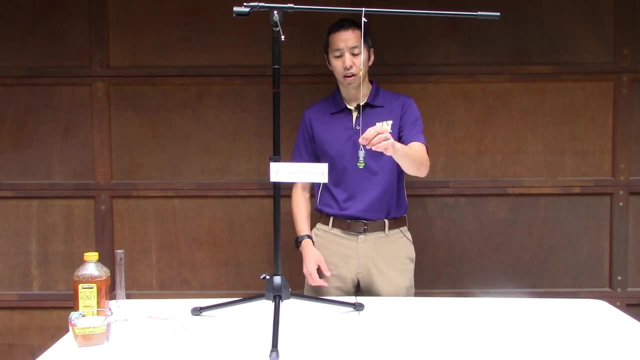 be when this rubber band is not elongated right. when it is, when it is, uh yeah, basically not elongated right, there's no force by the rubber band. so this is perfect, right? so when there's zero error, there's going to be zero force from this rubber band. and now? 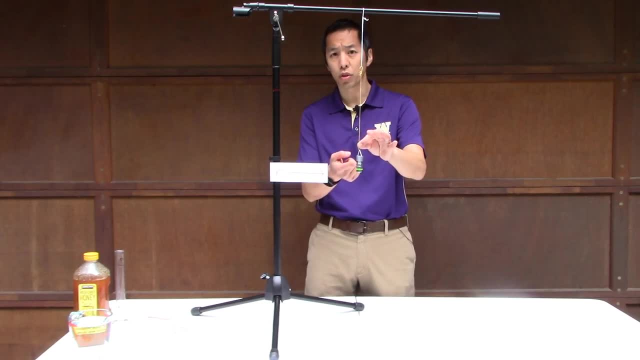 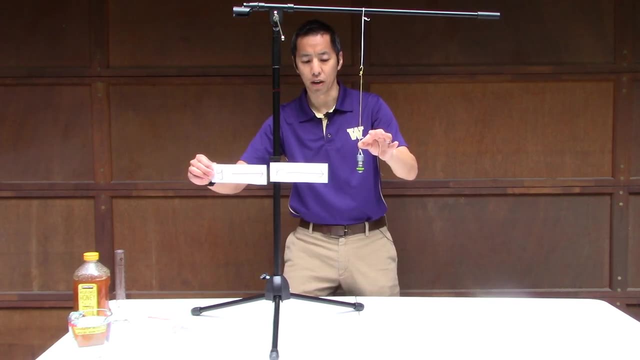 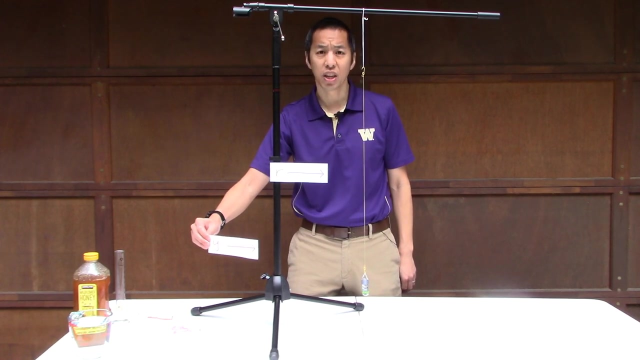 we should be able to let this thing go and and see how does this proportional controller work, right, because right now, if the position Y is right here at R, there's no force on the rubber band. but the problem is, as you can kind of see, is that that's actually not the case right. so this thing it's doing better than it. 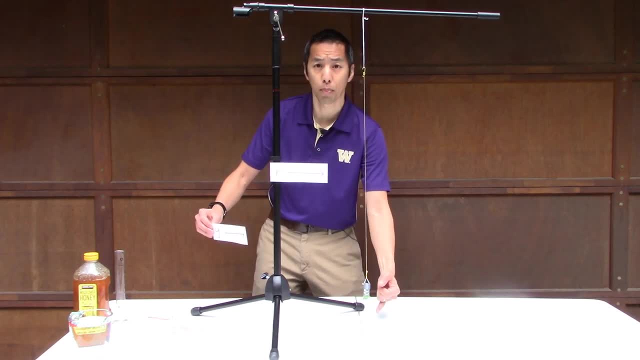 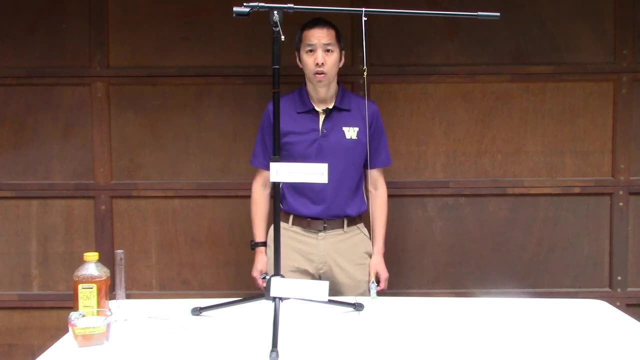 was before. right, it used to be all the way down on the floor. but now this proportional controller is able to move the position Y to about you know something like that. so we see there is steady state error in this case. so it's trying to bring it up to this R. but the fact that you actually 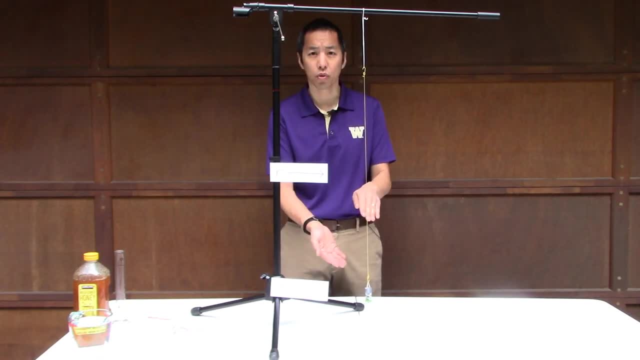 need some finite error in order to have a finite control is what makes this problem with a proportional controller a little bit. uh, it's not going to solve the entire problem right now. you might ask: is there something better I can do? how can I, um, how can I decrease this error? right, we talked about that. well, 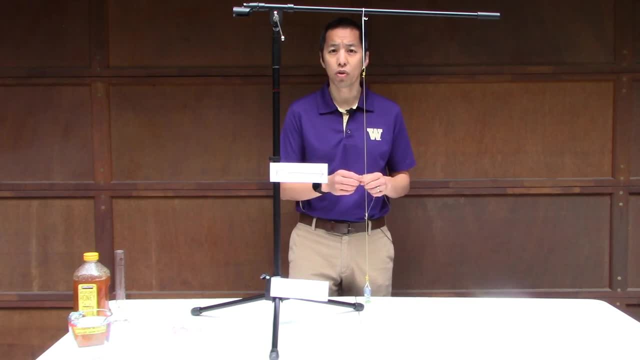 it means your first try might be to do something like just go ahead and increase the gain on your proportional controller. so in this case, what's the gain of the proportional controller? what's the physical equivalent? it's basically this spring constant. right, if we increase the spring constant, we 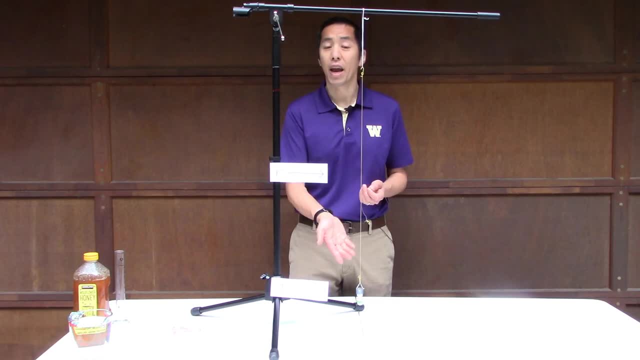 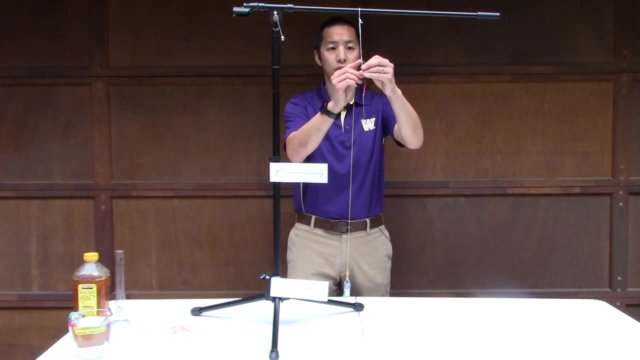 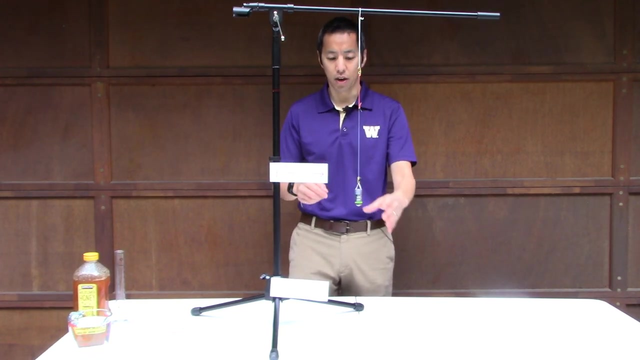 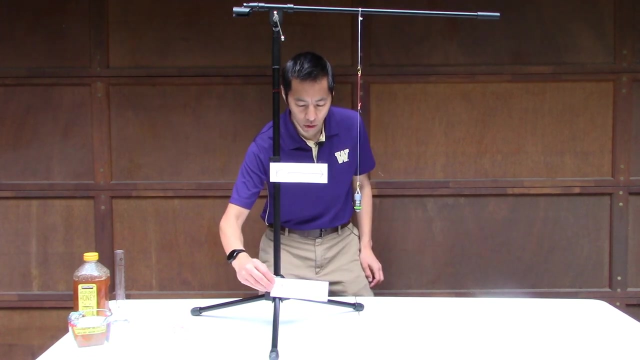 should increase the gain and therefore, um, the behavior should change. so I've got a stiffer rubber band here. let's do the same thing. let's go ahead and add now our stiffer spring and see if that changes anything. okay, so again now. aha, now look at this right. so again, we still don't make it. 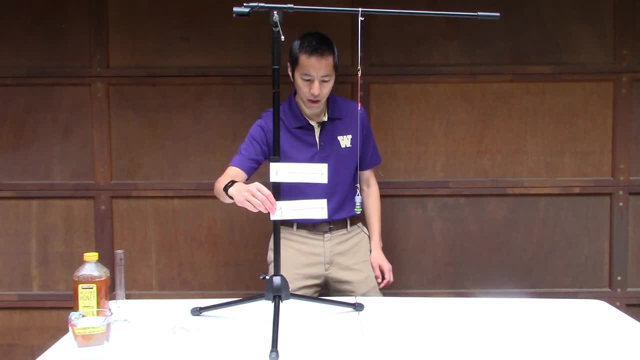 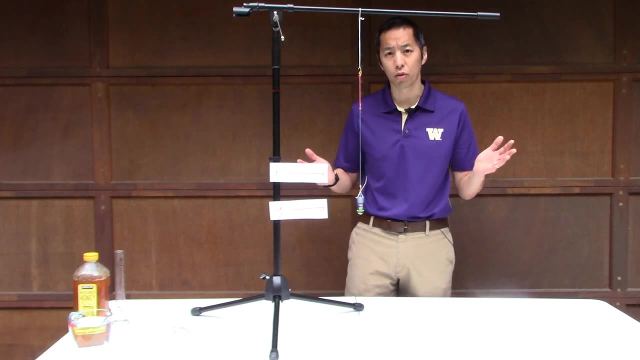 all the way up to R, but we have reduced the amount of steady state error. but again, the problem with the proportional controller is again: no matter how stiff you make this spring, in other words, no matter how big you make that gain KP, you are not going to get zero steady state error right. that's the whole issue now. 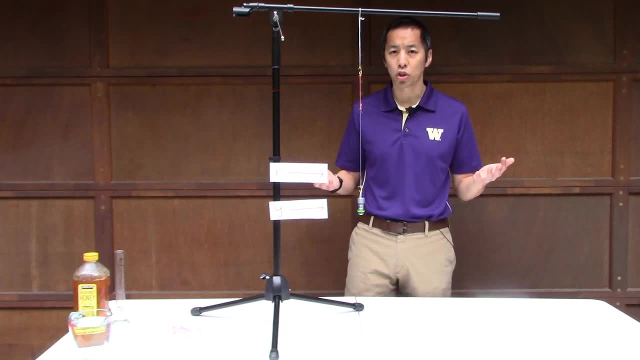 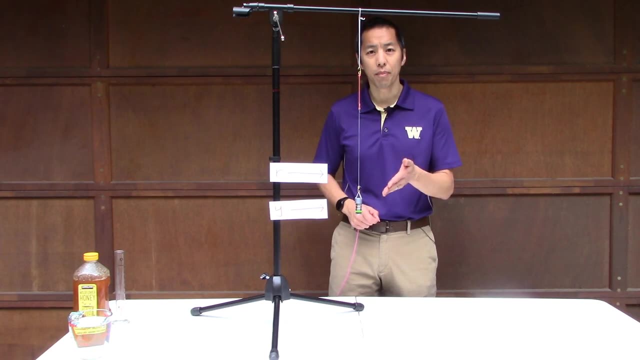 what we talked about on the board is all right. so if that's the problem with a proportional controller, maybe what we're going to do is start adding an integrator right. so now what I need is to add some type of control to this system where the control component right. 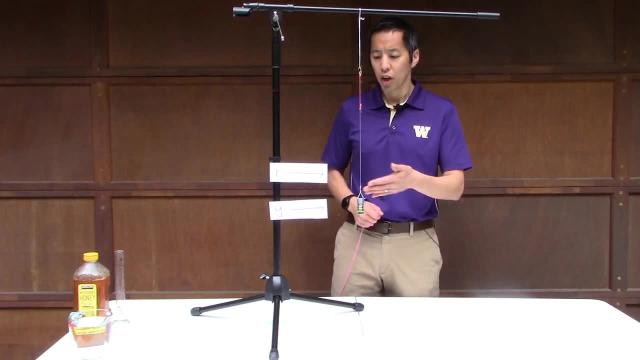 the UI. it's somehow related to the integral of the error, because right now, with just a proportional controller- right, we can be sitting here at steady state error like this forever and nothing is ever going to change, right? that's what the integrator is going to do, so I'm going to go ahead and add this: 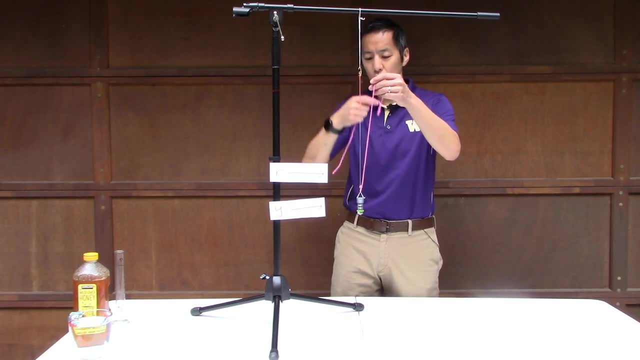 pink string. this pink string is supposed to represent the integral component of control and right now it's slack. you can see the integrator is doing nothing because we're going to pretend we start our experiment right now. and now the integrator starts seeing there's some. 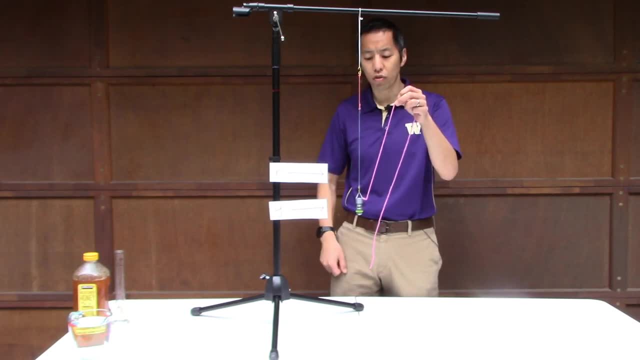 non-zero error, right? so it's going to start integrating it. so this string is going to start: whoops, hold on, it's stuck. this integrator component of the force. it's going to add on top of the, the proportional part, but it's going to start pulling harder and harder and harder. so I'm going to, I'm going to have 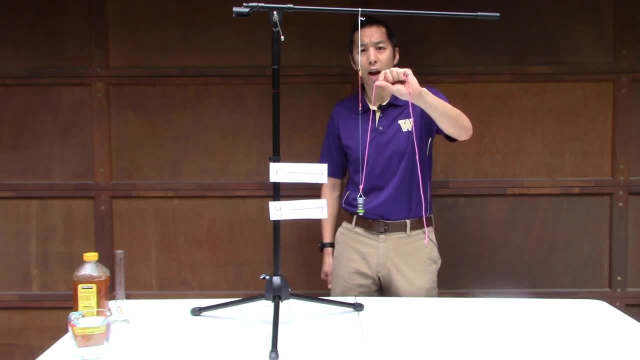 the integrator and I'm going to have to integrate the area under this air error curve and I'm going to have to start pulling and pulling, and pulling. and as I see that the the error is still non-zero, right, I'm going to keep pulling harder. 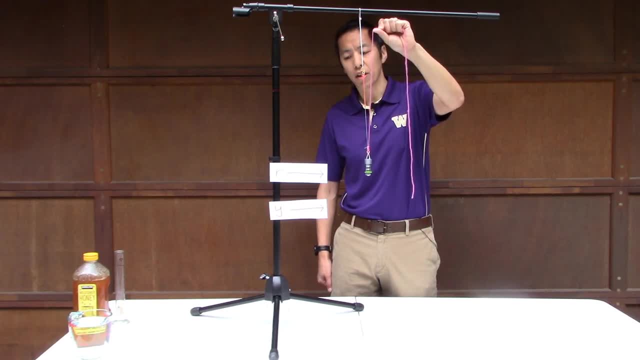 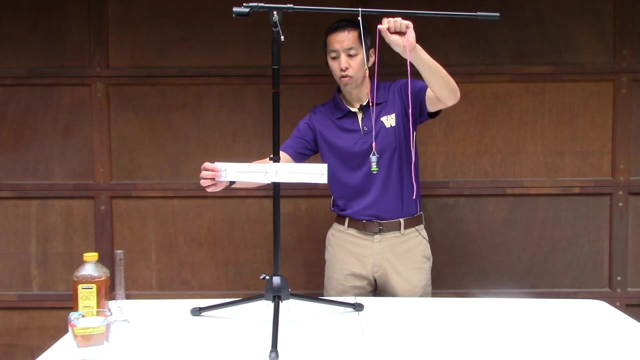 and harder and harder until eventually it hits here. but I've wound up so much error in my integrator that it might overshoot a little bit and then it might come down and oscillate and whatnot, but at some point, right, the pink string component you can see, brings the actual position of the weight up to R. so now R. 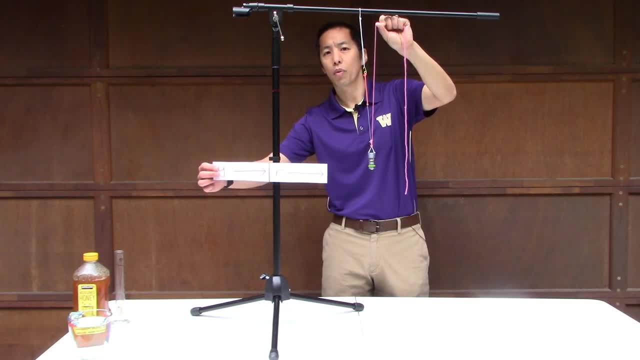 and Y are the same thing and there's zero error. and what we said earlier is because there is zero error. right, this rubber band, the, the, the spring or the proportional component is doing nothing. right, the pink string is taking up all of the force, is generating all of the control, right? so this is kind of 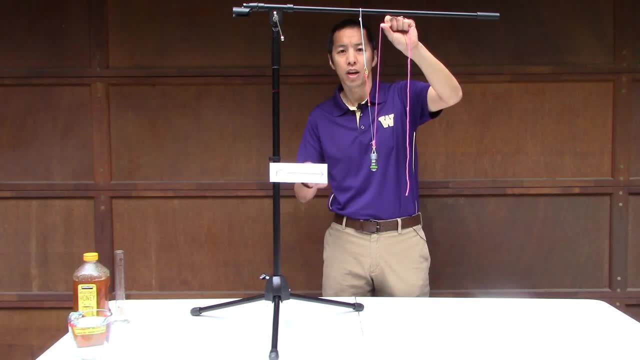 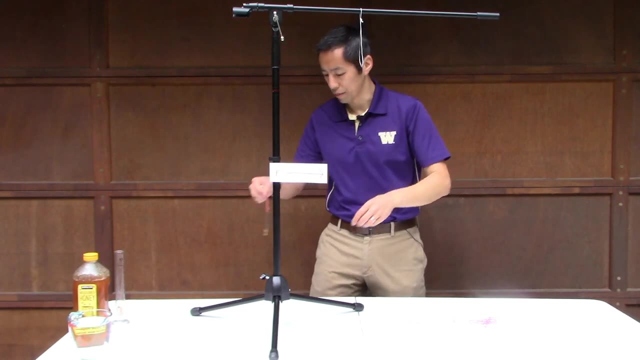 interesting. so there you go. here's a physical demonstration of a PI controller. why don't we add the last component? let's go all the way to maybe PID and and for giggles. let me go back to the um, to the weaker spring, because this one is. 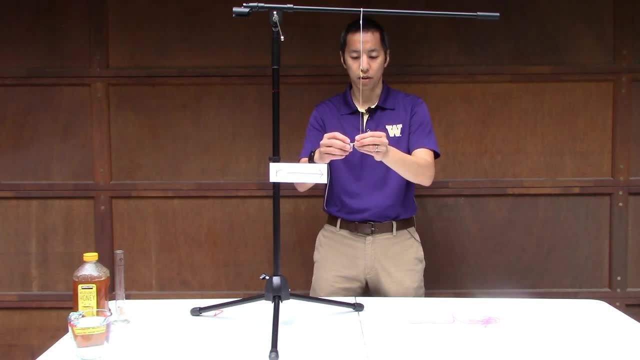 actually more interesting. so let's go back here. uh, if I can hook all this back up, okay, all right. okay, so now we're back here. right, here's our P only controller again, our. we've got some error. now let's go ahead and make. let's make a mark where. 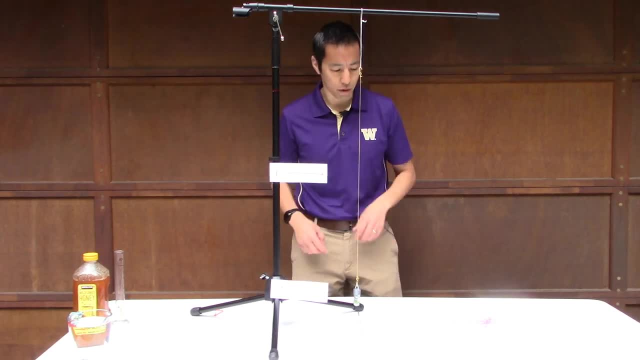 that is okay. again, we're trying to get up to this reference. and now, um, you know we made the claim earlier that this is a P controller only. right, because right now there's only a force which is directly proportional to this distance. right, actually, if you think about this long? 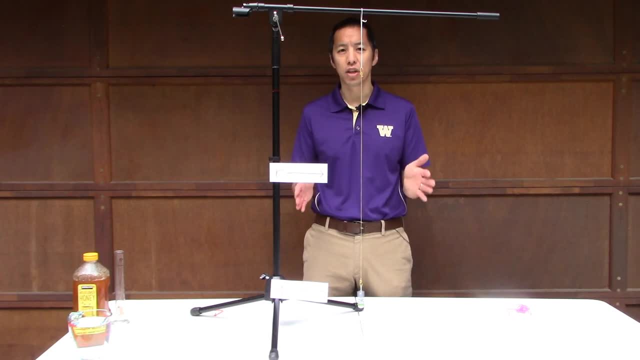 enough. this is actually a P and a very weak D controller. right now, because there is a force that is acting on this weight which is proportional to its velocity. right because we're sitting in it, we're sitting in a fluid. right we're sitting in air. so there's some. 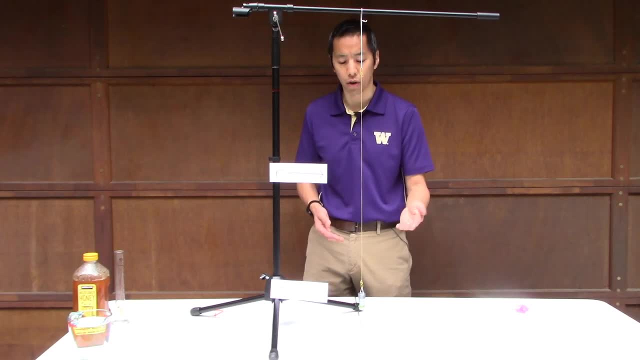 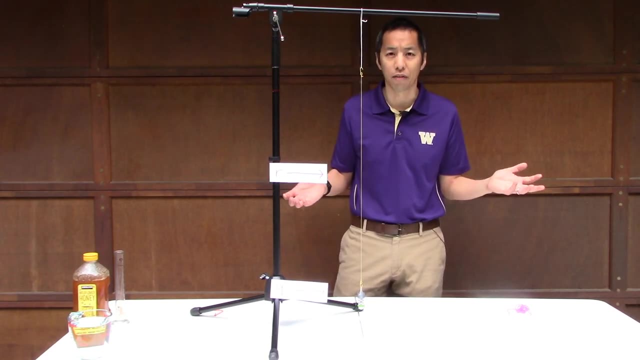 air resistance. right, that the faster you try to go through the air, the more force it's going to put onto it. of course, that that magnitude is negligible, right, because the air is, it's it's not very viscous, there's not a lot of aerodynamic drag in this regime. okay, but what if we increase? 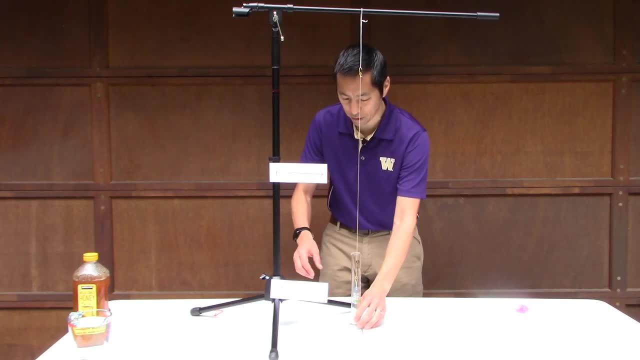 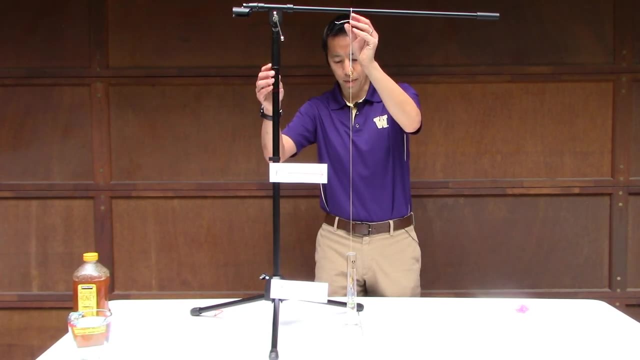 that. so, for example, let me put this inside, maybe this little graduated cylinder we've got here, okay. okay, let me scoot this over just a skosh, just to make this thing up a little bit more nicely, okay, okay. so I want to add now, or or I guess I to be- 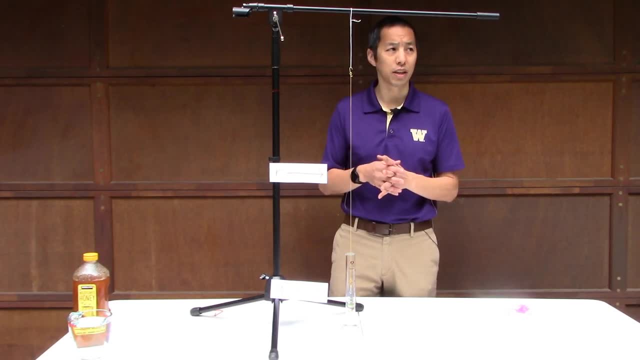 technically correct. I want to increase the derivative component of the PID controller, right. so what I need is I need to increase the amount of force that is applied to this, which is proportional to its velocity. so if air is not a very good viscous fluid, why don't we? 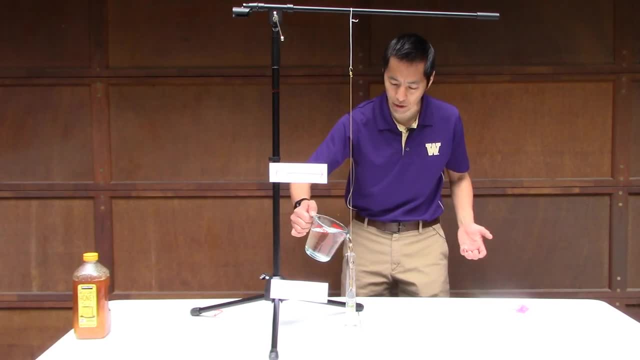 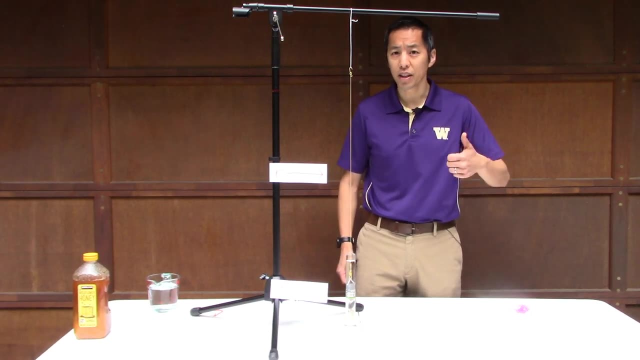 try something a little bit more viscous, like: what about water? so if I pour water in here right now, what we have is I have basically increased the D component of this controller. right, because now you see how much more damped out. it is right, you see how this thing does not. 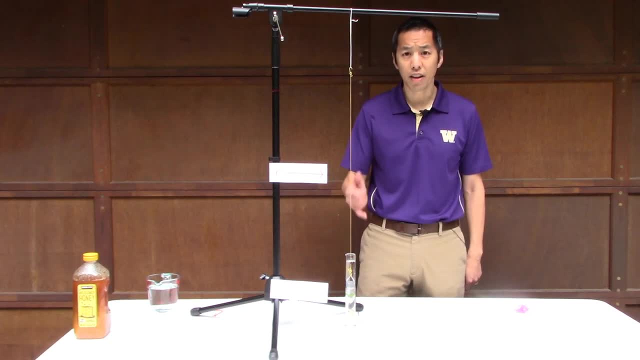 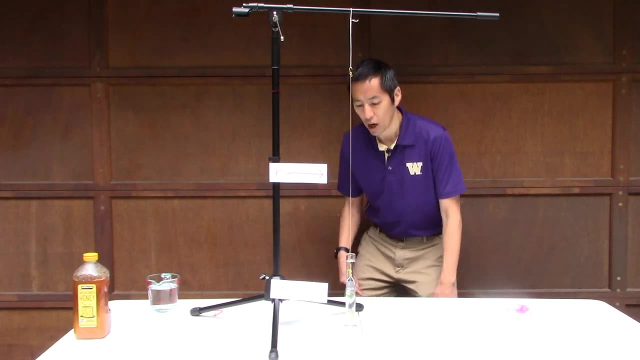 bounce around or oscillate as much, right, because there is now a lot more force, it's much harder for that weight to move through the fluid quickly, right? but what's interesting also is: look at this PID state. the derivative is doing nothing, right? the velocity is zero, right, error dot is zero. so 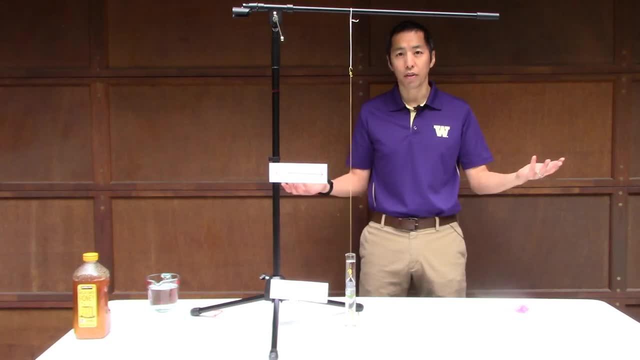 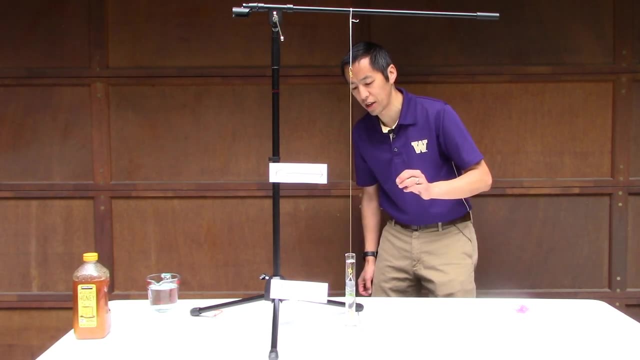 the velocity is zero. so right, the derivative component actually isn't playing that much of a role in this situation, right? so, again, just to maybe compare and contrast, let me oscillate this a few times, and you can kind of see that when we increase the damping ratio- or, excuse me, increase, 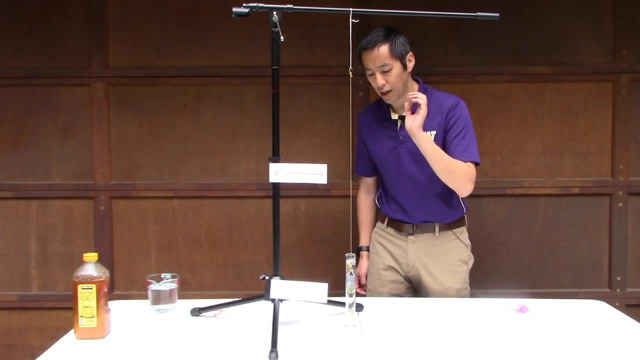 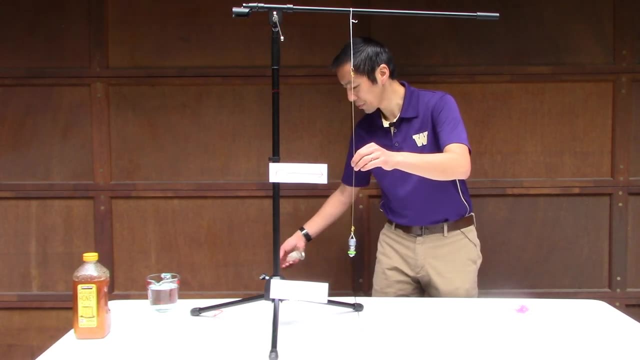 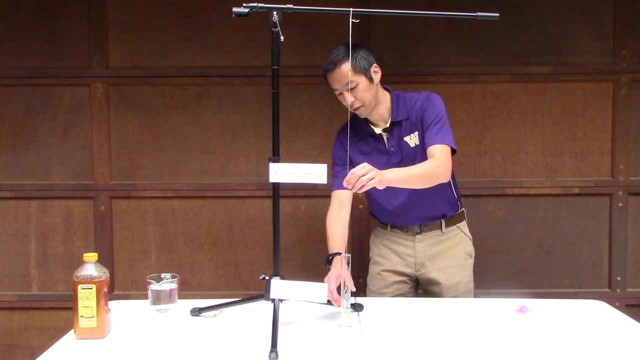 the D component of the PID controller. you see there's a lot less oscillations right and again. just to compare and contrast, it is with water. let's go ahead and pour this out and again. now you can kind of see with air: whoops, right, there's a lot more. i guess it's kind of sticking now. okay, this isn't quite the way i. 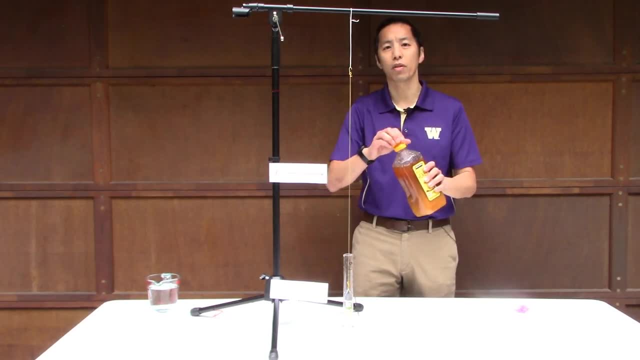 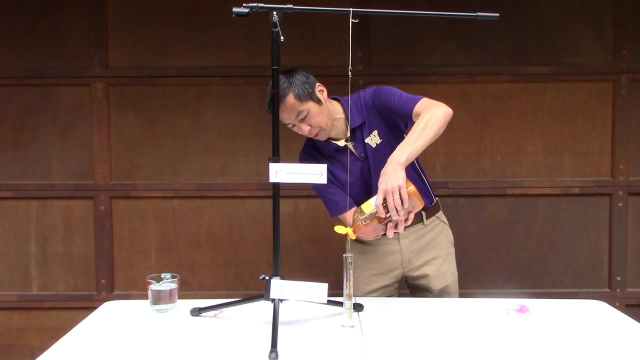 envisioned it, but you get the idea right and we can even go even further, right? what if i want something even more viscous? what about, like honey? right, if i pour honey into here? this is going to really increase the d component of this controller, actually probably to the point of it being a 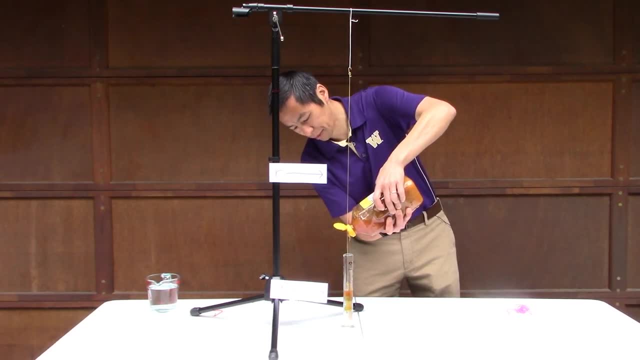 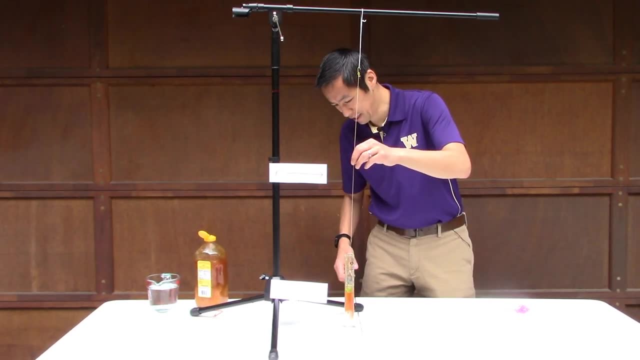 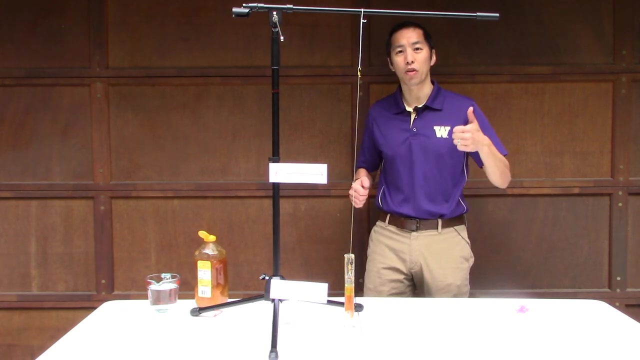 little bit ridiculous, um, so give me a second to fill this up. i'm just kind of curious to see if this is going to work. okay, let's try that. boy, oh, boy, okay. so now we have really messed it up there. the the d component is way too high, so 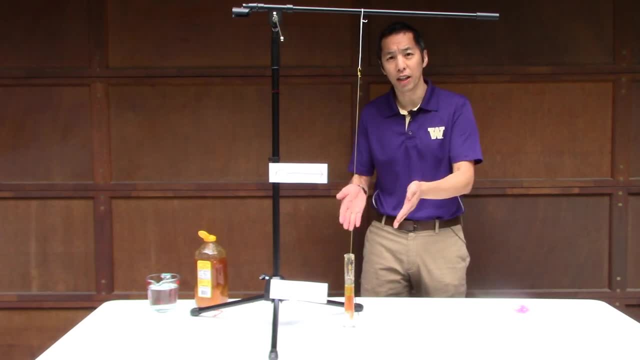 you can see, the thing does not want to move, but it is moving, right if we let this thing sit long enough. right, that d component of the control is not going to affect it. right, because the velocity is going to be zero, so there's going to be no force on it. so all of that should work out, and 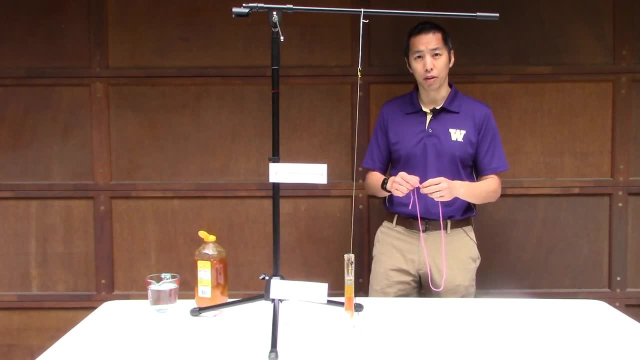 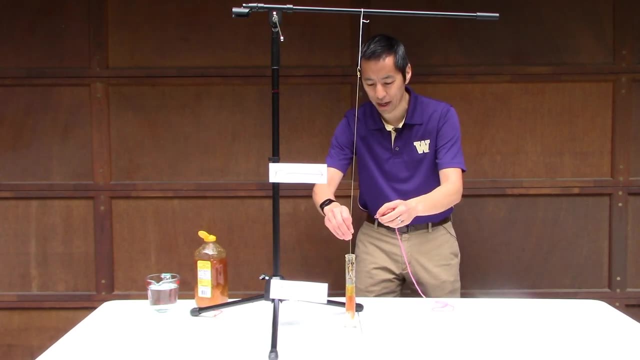 again. i guess, in the, in the interest of completeness, let's talk about the full thing now. so we've got the proportional, we've got the derivative right, which is this viscous fluid. now let's add the integrator back into this picture. again, my integrator is this pink string, and again we can. 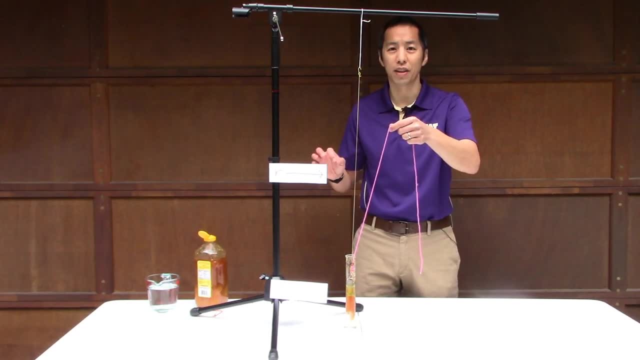 play this game. so now this is sort of a you can think of as a physical manifestation of this full pid controller. so now you know it, it has moved around and now i'm going to start pulling on this integrator, i'm going to start integrating this non-zero error and i'm going to start bringing 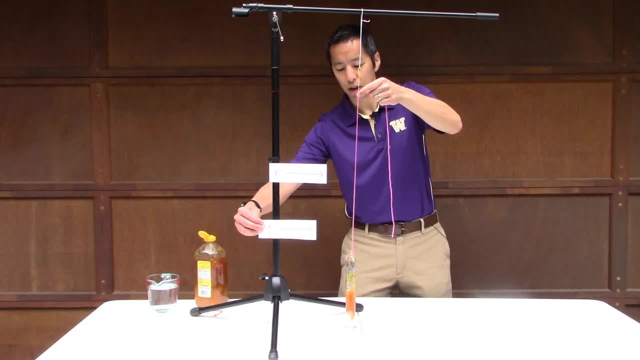 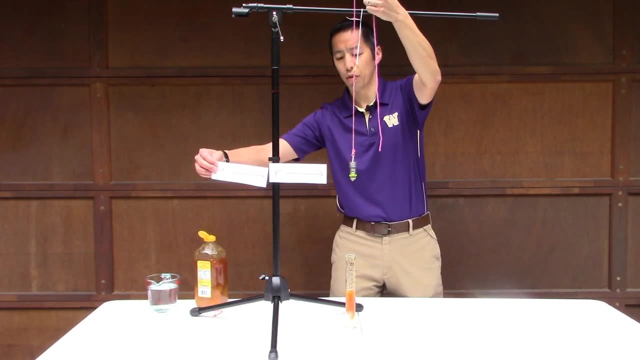 this up to where it wants, to be right, that. so now the integrator is doing the work, the integrator is doing the work, the integrator is doing the work until we come up to around here, right, and now again, you can see here, at this point, even with the full pid controller, right. at steady state, when everything is where it wants to be. you can see here, at this point, even with the full pid controller, right at steady state, when everything is where it wants to be. you can see here, at this point, even with the full pid controller, right at steady state, when everything is where it wants to be. 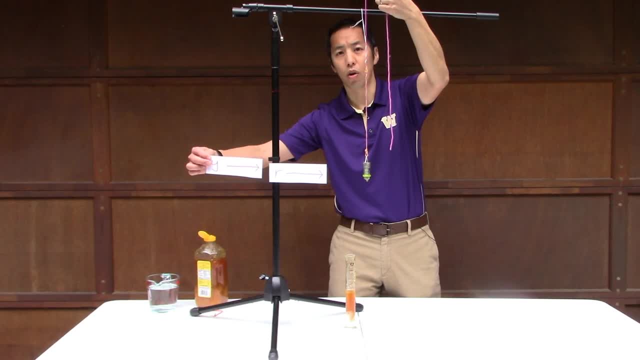 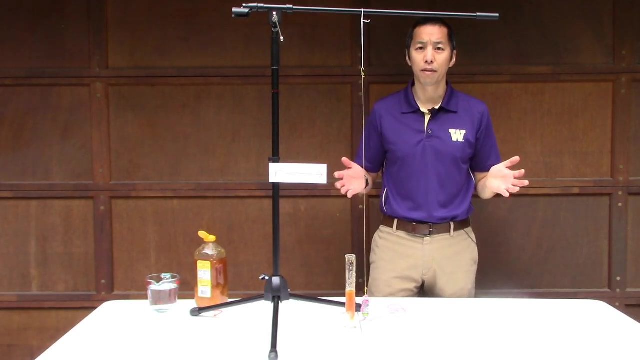 it's the pink string which is taking all of the work right. the all the control authority is coming from the pink string. the rubber band, slash spring, which is the proportional component, is doing nothing, and the derivative component, which is basically the viscous fluid, is doing nothing, right. so that's my- uh, my demo. hopefully this gives a little bit of an intuitive feel for what this pid controller is doing. right, you can almost think about it as a proportional component is adding some amount of springiness, um, to your 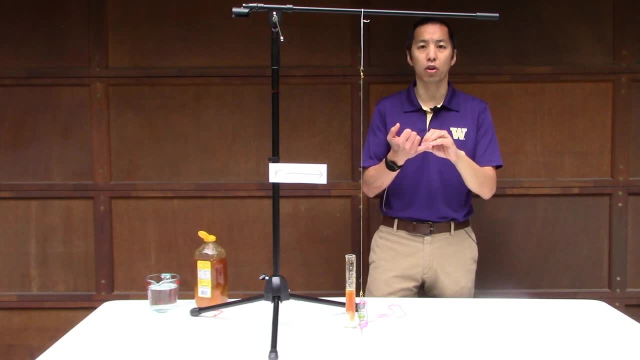 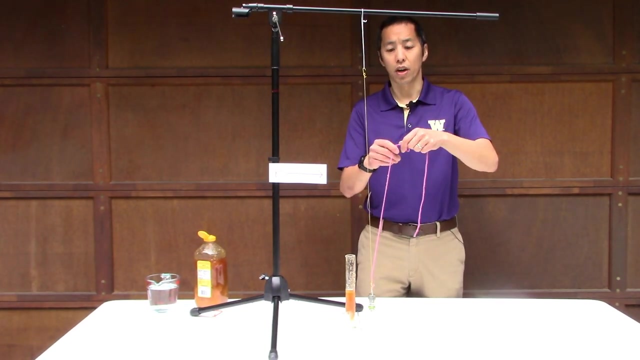 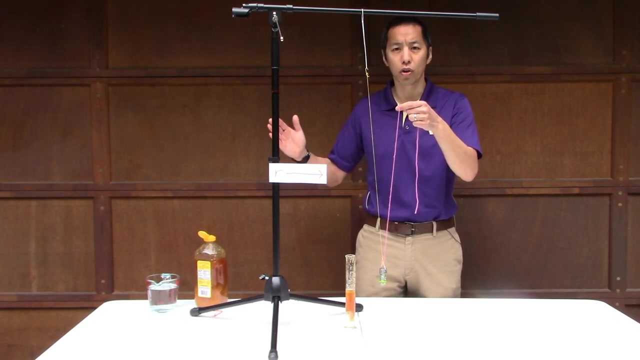 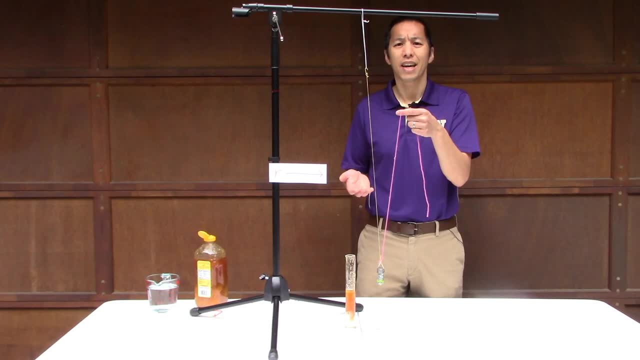 the control signal. so the integral sort of thinks about the the past. and from this analogy you can also see that i guess, um the integral, you can kind of think about it as like adding inertia to your system, right, because the integrator winds up all of this state error and it has a tendency to overshoot it's. it's like this idea of momentum, of inertia, or inertia of your system, right. and then finally we saw the d component of the derivative component, right, that is almost thinking about you, can. you can kind of again think about, like thinking about the future, right, it thinks about, looks at. 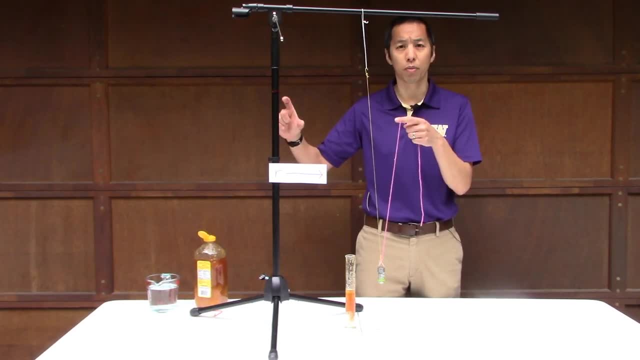 the roots of the future, right, you can kind of draw到 things around the future. right, it's almost thinking about where the system is going to go. you can think about the time periods of time rates of change to kind of help predict where the system is going to go. so you can see the PID mane. 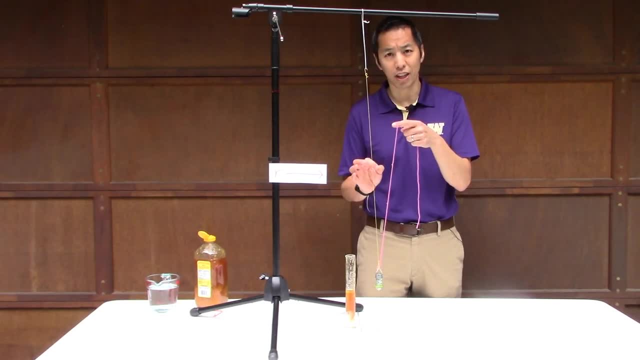 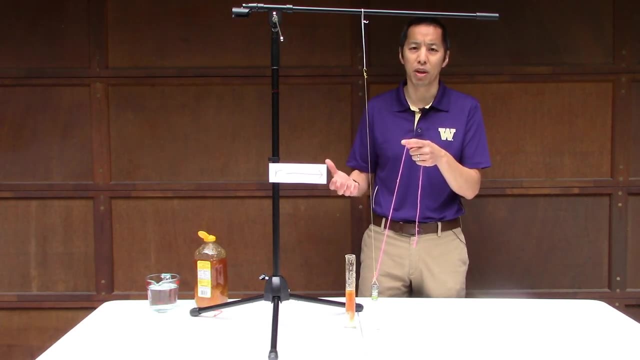 self controller is sort of looking at the present, the past and the future all at the same time in kind of a loose hand wavy sense, and then lastly, um. the last analogy to maybe draw is that again we saw the derivative component is sort of basically a past, present or sorry, present, past, future kind of system, or you can think of it as: 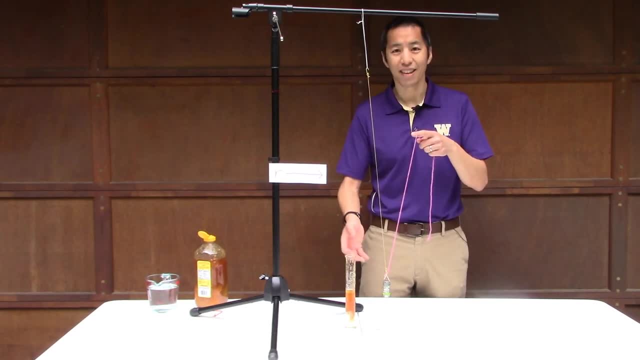 like a adding a spring, mass and damper to your system. So there's a lot of nice kind of parallel analogies but again, I think the rigorous way to look at it is mathematically, as we saw earlier on the board, I hope this demonstration just gives a little bit of a physical intuition of what all. 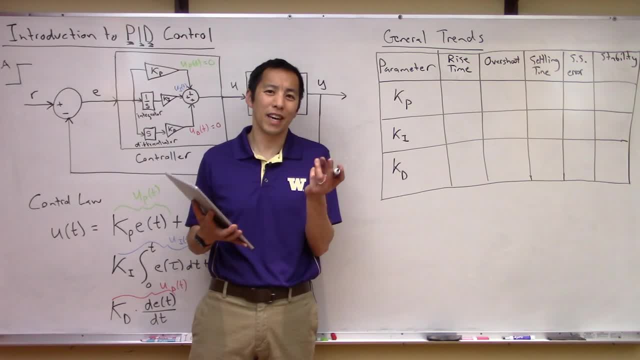 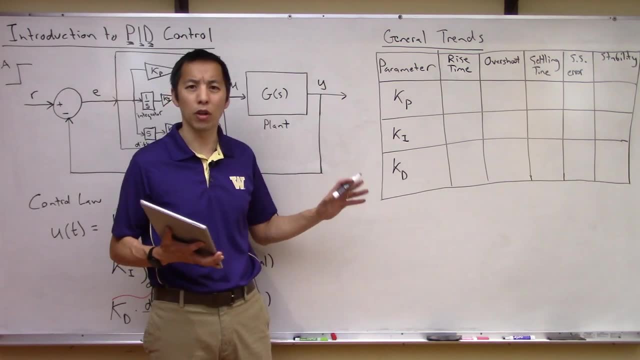 these components are doing All right. so now hopefully you've got a good intuitive feel for what all of these terms do, So maybe it might be helpful to just make a little quick table. This is sort of some rules of thumb about how adjusting these parameters are going to affect. 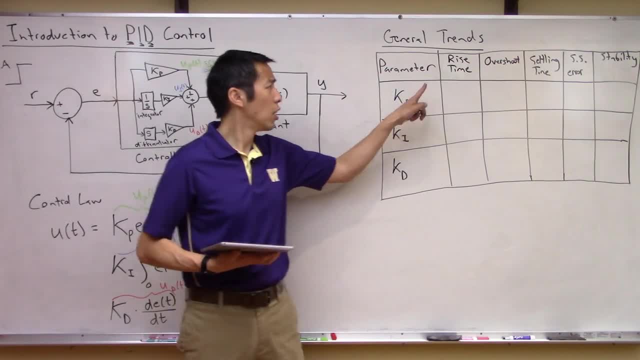 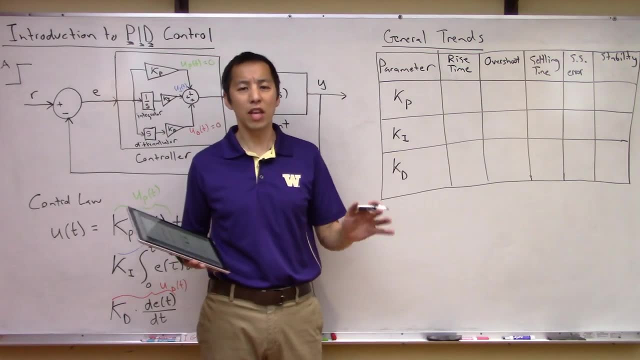 different parts of your system. So if you adjust KP, let's ask about how does that affect things like the rise time, overshoot, settling time, steady state, error and the stability? And again, keep in mind these are real loose generalizations, shooting from the hip kind of ideas. 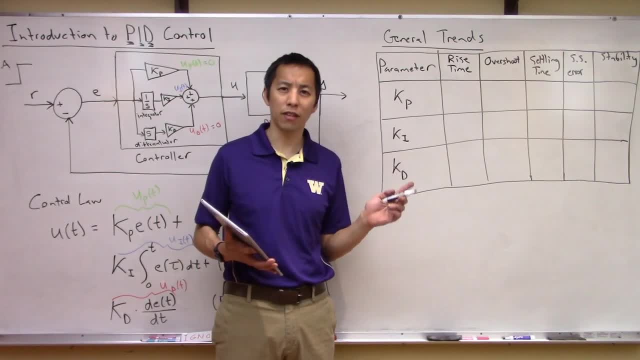 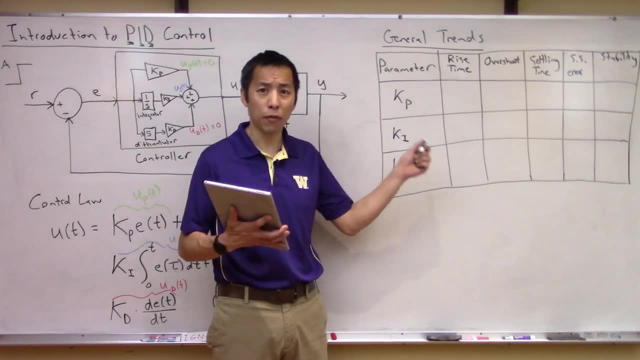 Don't take any of these for gospel. We will do the actual analysis down the middle of the video. So if you have any questions, feel free to reach out to me. The road in other discussions so we can make quantitative and qualitative statements, But for 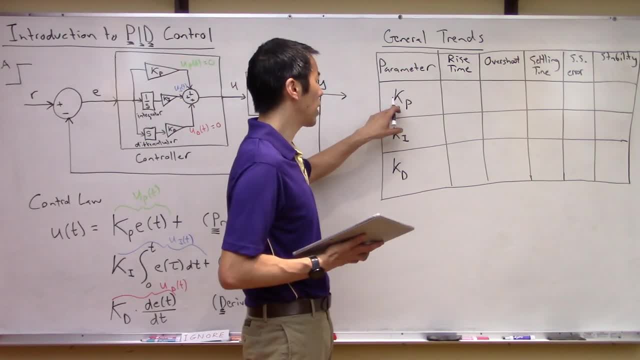 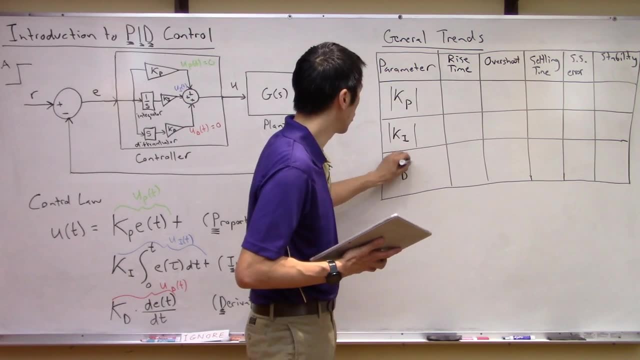 now let's just look at these general ideas. So again, what we're talking about here is if you make KP bigger and again, maybe, this is maybe really- if you make the absolute value of these terms larger, right As these sort of increase. basically you're talking about making these. 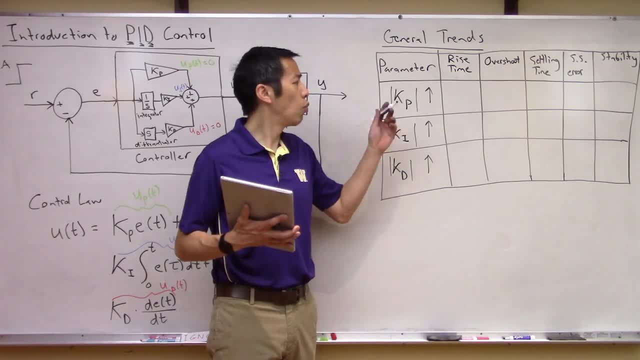 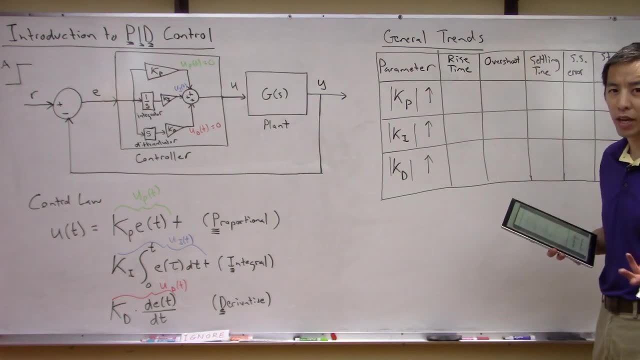 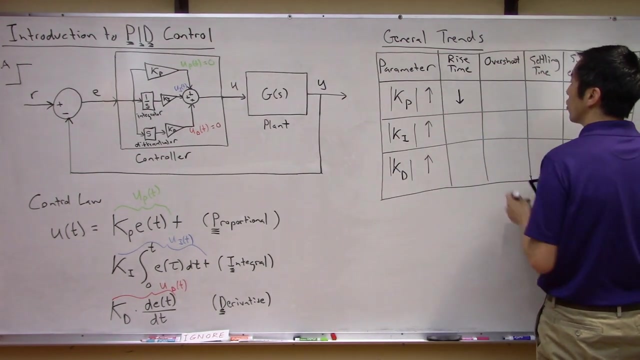 components more aggressive. What does that do to all these parameters? So we saw that KP. this is really like it's kind of like you think about as adding like a spring right, A stiffer spring to your system, right. So what this does for rise time is: this is going to generally try to, it's going to decrease. 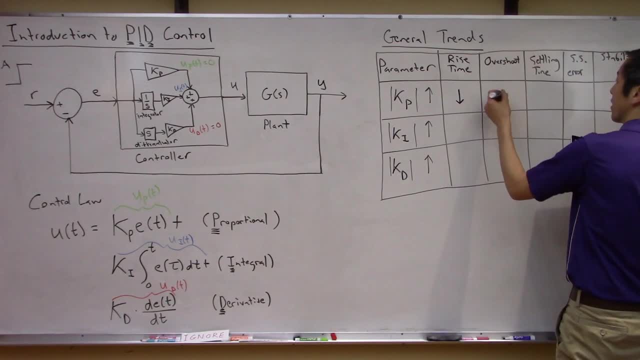 your rise time right, You're going to get there faster. The consequence of this is usually this is going to make your oscillations or your overshoot, go up Settling time. this is really a small change. It doesn't have much effect here. okay, Steady state error. we saw that this is going. 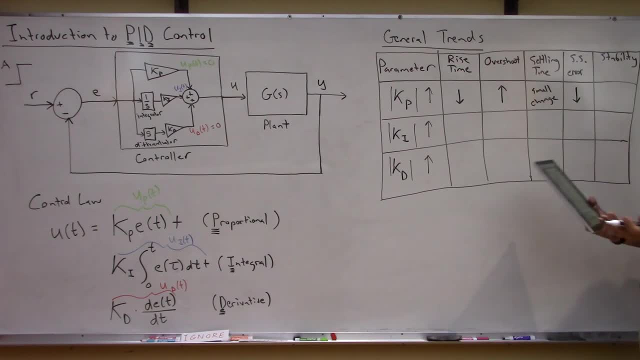 to decrease your steady state error, Right, But you're still going to have steady state error with a proportional only And in stability. the problem with this is it sort of decreases your stability- right, It degrades your stability. It makes you more likely to have issues and become unstable. okay, Let's talk about the. 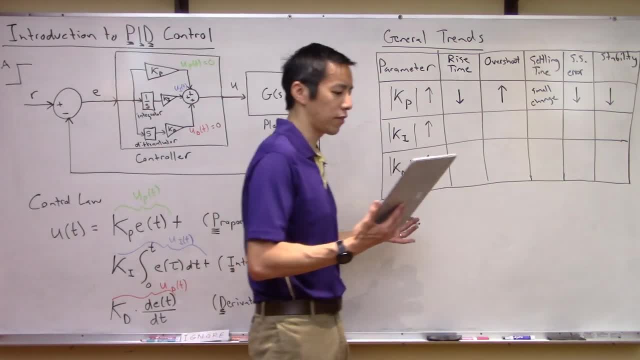 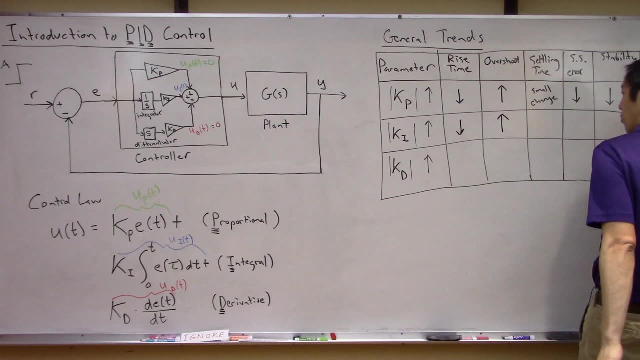 integrator. As you make the integrator magnitude larger, how does this affect it? okay, So your rise time, this tends to go down Your overshoot. we saw the. you know the integrator is one source of major overshoot in this case, So this goes up. 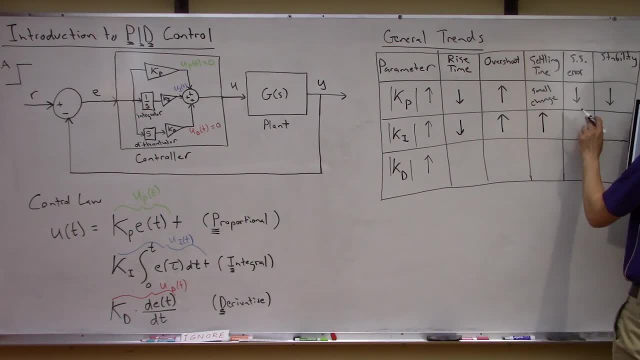 So the rise time. this also tends to go up, okay. Now, the nice thing about the integrator, though, is steady state. error. this, really, you know. it eliminates it, right. That's the whole point of the integrator, So let's just write eliminate here, okay? And in terms of stability, though, the price you pay for this is again. 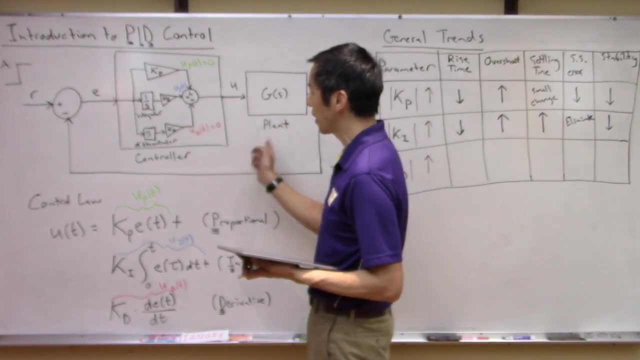 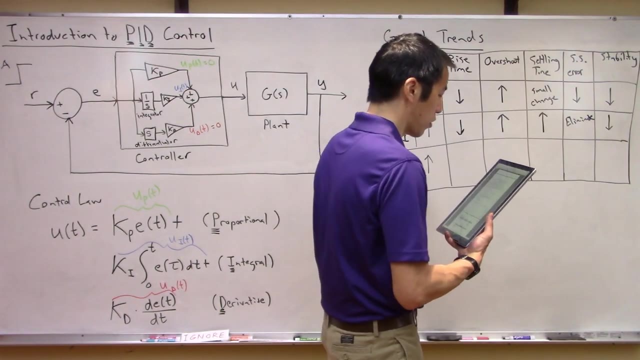 you add the integrator, you add some dynamics and you're more likely to make this overall system unstable. okay, So you got to be careful with that, right. Okay, Let's talk about the derivative. okay, So the derivative- again, this is: 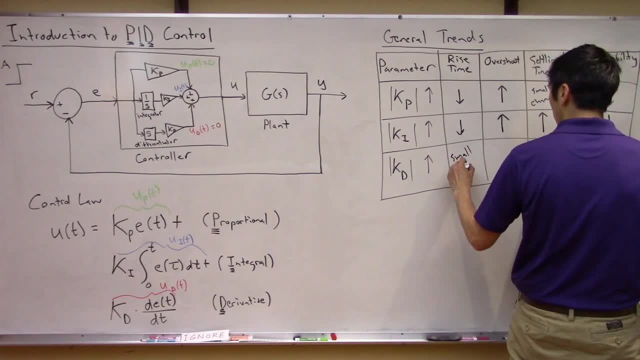 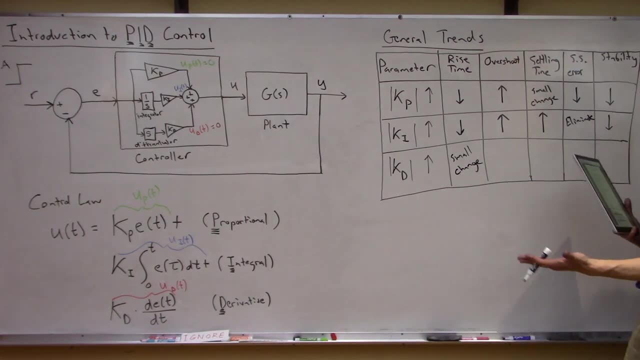 doesn't really do much to the rise time so it's not going to matter a ton, right, what it does do, right, we saw that the derivative it's. it's like adding a damper to your system. so actually this decreases your overshoot, right, it makes. 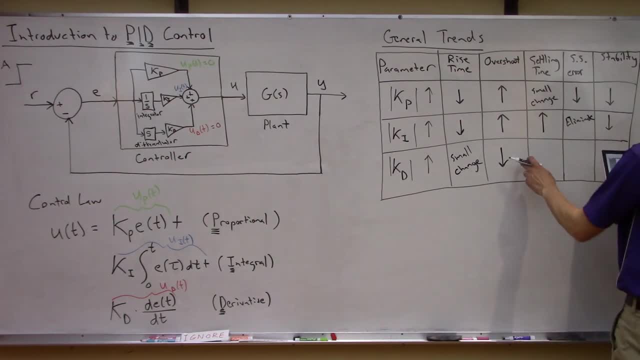 it like you're sitting there in honey and it's making it slower, so it's less likely to overshoot. um, okay, settling time. this also. if you increase KD, it tries. it usually makes your settling time a little bit less because your oscillations go down now and we saw steady-state error. this is really no. 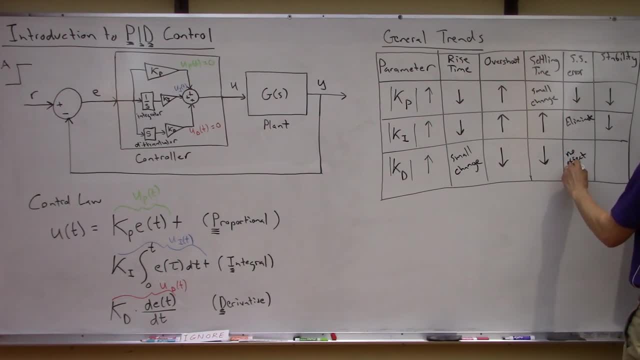 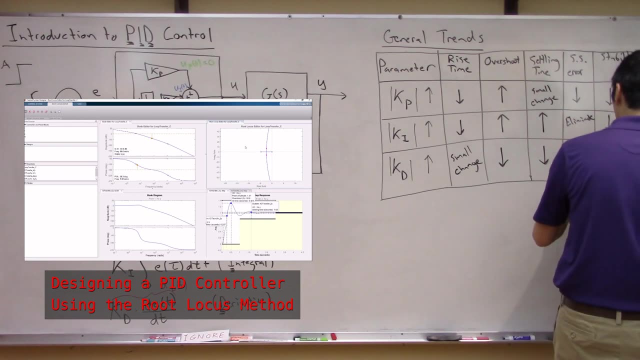 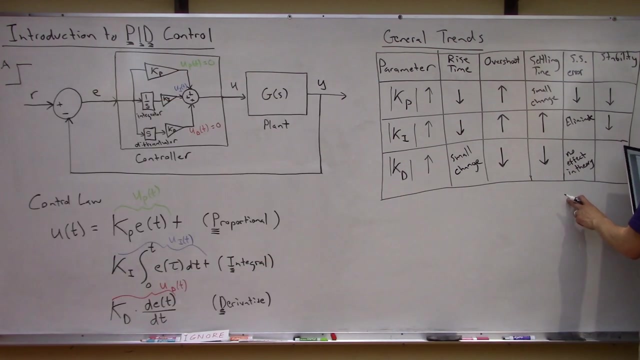 effect in theory there are. we're going to see when we start looking at this from designing a from a root locus perspective or other techniques, that this does sort of affect it. but really right, we saw that at steady-state the derivative really is not playing a role. okay, um, and this is also the stability. 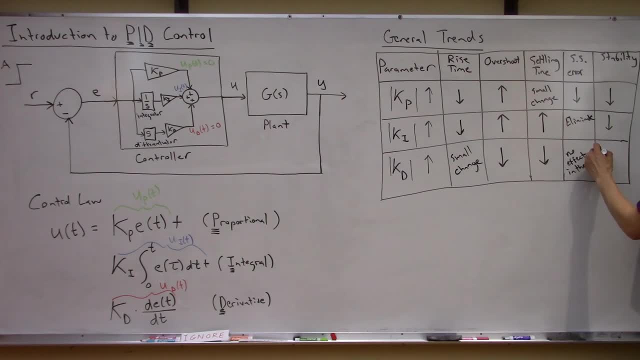 is. I don't know if I want to draw any hard conclusions here. let's just say that maybe this, this might improve stability if KD is small. so it's again. it's one of these things: everything in moderation. you don't want to go overboard, because you definitely can. 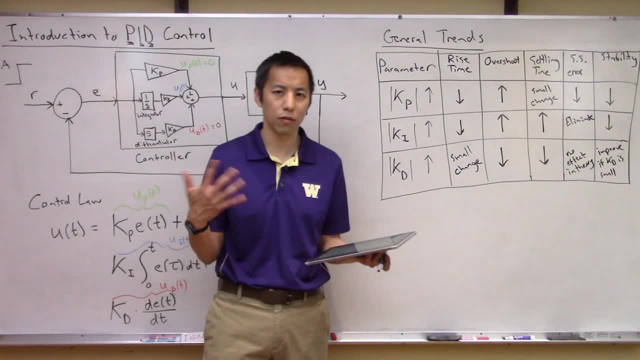 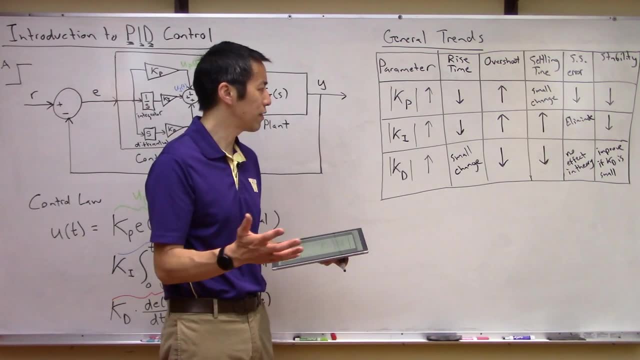 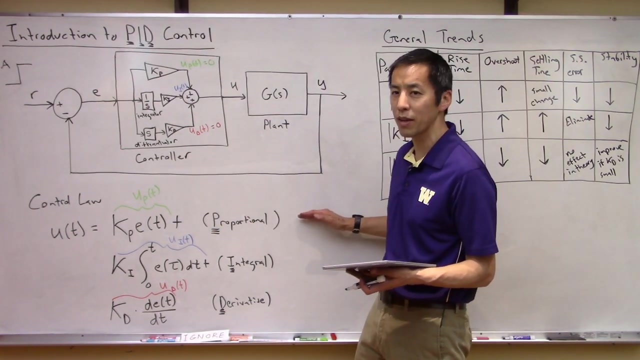 drive things unstable with a large KD, but if you keep them small, it's it's usually pretty reasonable. so again, these are some rules of thumb, um about how to tune these gains. again, right, because the whole game with the PID controller we said it's incredibly versatile. it's used all over the place. the only thing you got to really do is pick these three numbers: KP, KI and KD. and the only thing you got to really do is pick these three numbers: K P K I and K D K P I and K D K P and K D K I and K D K I and KD K.